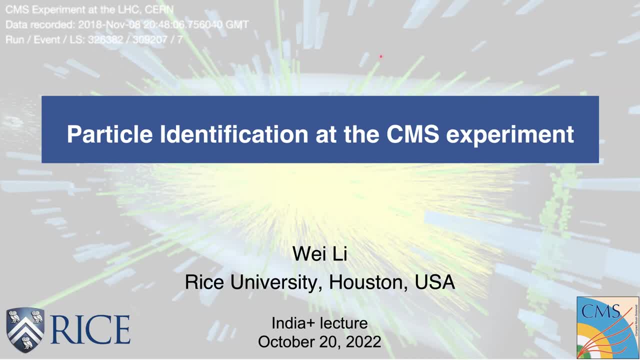 talk, professor lee, please. okay, thank you, uh. thank you for the, for the introduction and and also the opportunity to tell you about the cms experiment. um, so, this is an experiment that i work on and uh, so, yeah, i learned that. uh, last week you heard from about the star and at least, 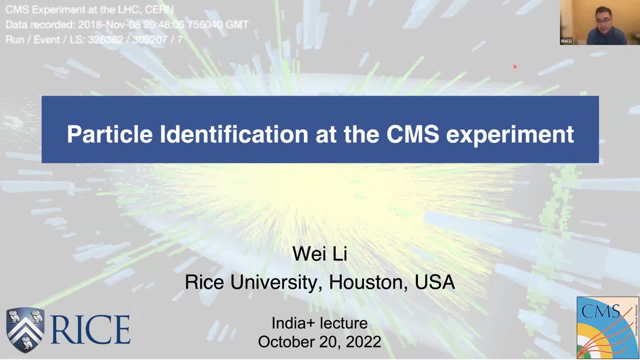 uh experiments. so those are the experiments dedicated to uh, to have a physics uh, whereas the cms experiment is probably best known as a particle physics experiment. right, it's a general purpose project experiment. however, it was designed um. it was designed uh in such a comprehensive way that 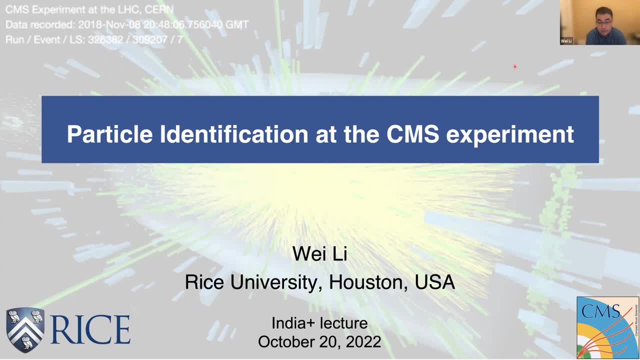 it turns out, it's also an excellent detector for, for hyperphysics. um, this is- i will try to tell about this today- and, um, and in fact, uh, speaking of the particle identification, um, this is something i actually probably uh, uh, the cms is not best known for and, however, i will also, uh, show you that. 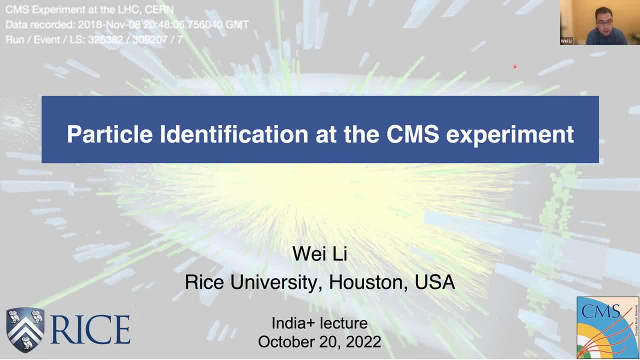 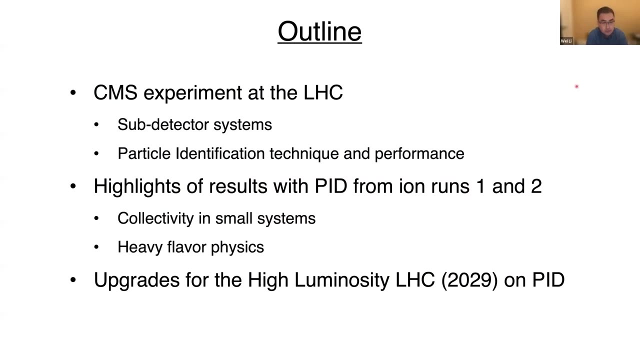 actually, where cms is also very competitive. um in uh, with the pilot identification, and that are physics we can, can do with that. okay, so we move along. so, as this is my plan, so i'll first, uh, I will introduce the, the detector, the cms experiment at lhc. i will walk you through all the Uh, it, uh. 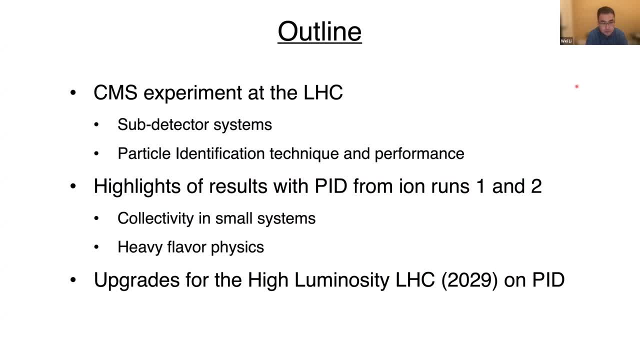 will walk you through all the key sub-detector systems and, along the way, I will introduce you to the ParticleID techniques for each of these subsystems and show you some of the performance. So then, with that, I will highlight some results we had with ParticleID. 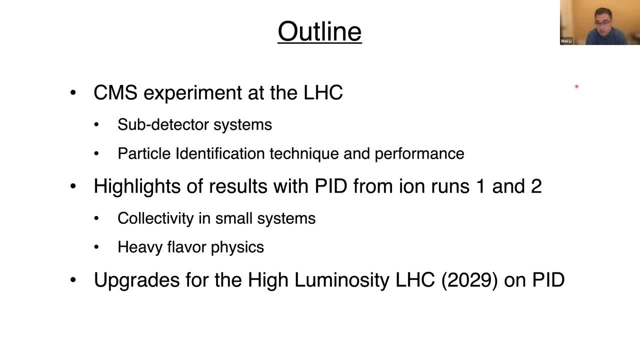 from the Havion runs from LHC Run 1 and Run 2.. The Run 2 just ended in 2018, and this year we are starting LHC Run 3.. I will focus on. there are lots of results coming out of the CMS Havion. 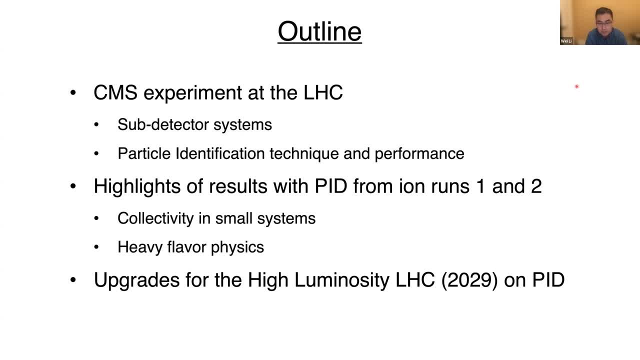 program. I'll focus on two aspects where the ParticleID played an important role. So one is to study the collectivity flow in small system collisions and the other one is related to the heavy flavor physics in Havion runs. And in the end I'll also tell you about the upgrades, the future upgrades for 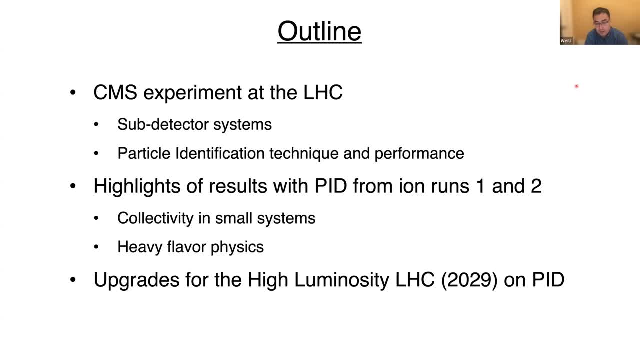 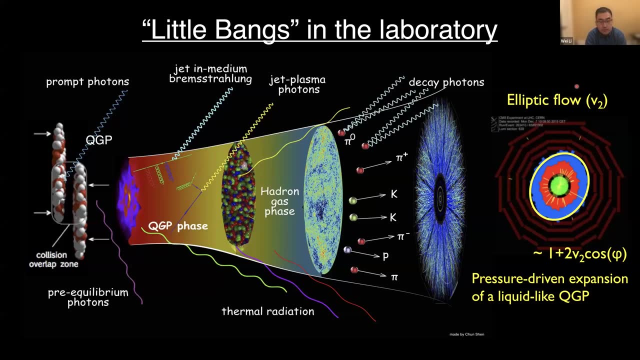 the high luminosity LHC in CMS, where there is a new detector that will provide us a new ParticleID capability. Okay so, very brief introduction, because I know you already got some background from last time. Okay, so let's get started. So I'm going to talk a little bit about what we did in the last week's. 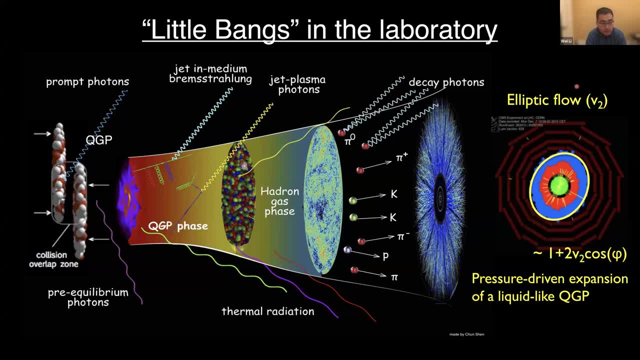 talk That in the in the Havion collisions, as we know, we are collecting two relativistic moving ions like two pancakes, where the expectation is that we want to create a very high energy density, very high temperature medium which kind of mimics the very early stage of the universe. It's like 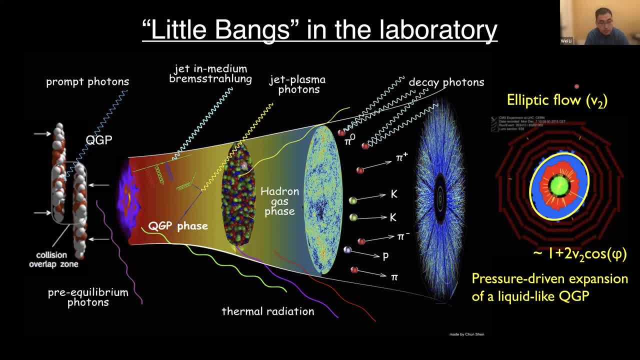 oh, big bands in the laboratory. And shortly after the collision, the medium that we created. we call it the quagmire plasma, and it will then rapidly expand and go through a stage of hydrodynamic evolution And at some point it will turn. as the temperature goes down, it will. 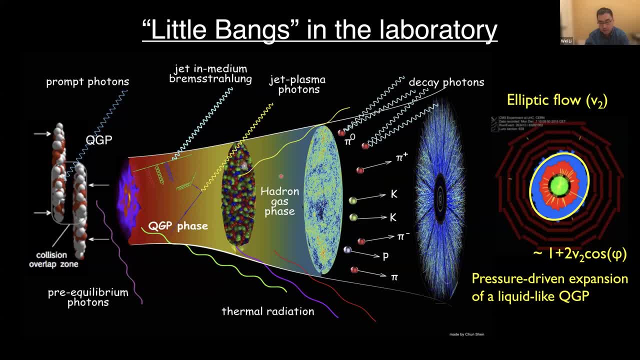 go back to the hydronic phase and it will still in the hydronic phase. it will still interact a little bit until at some point it will freeze out and all the energy will, entropy, will turn into particles that we will detect in the experiment. So there are different types of 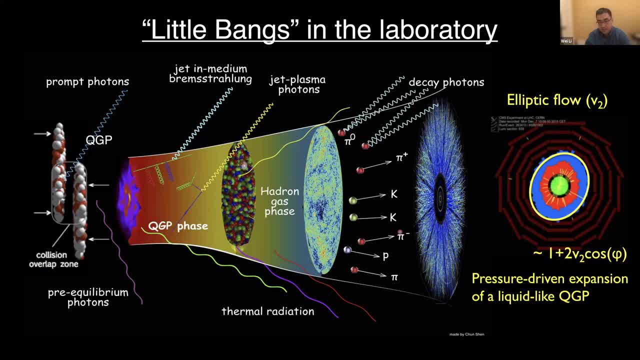 particles that will come out of these collisions, like the pion ka, proton, the charged particle, neutral particles and pi zeros decayed to photons and so on. So we're going to talk a little bit about how weIt's kind of solid. you can see the electron and the neutral one, And then you can see 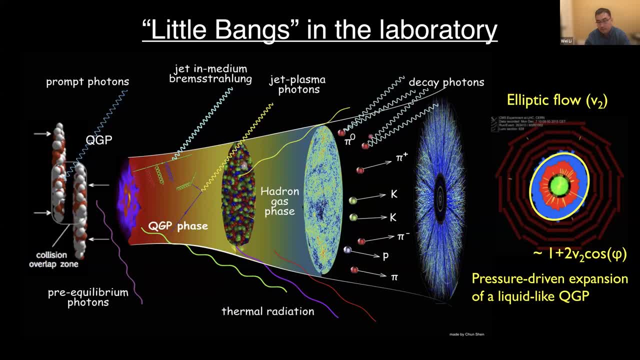 the toton and you also see the leptons and so on. So basically, by mirroring these particles of the last scattering at the freeze out, we try to trace back to the information happens early on, so the dynamics during the process of the collision or the evolution of the QGP. 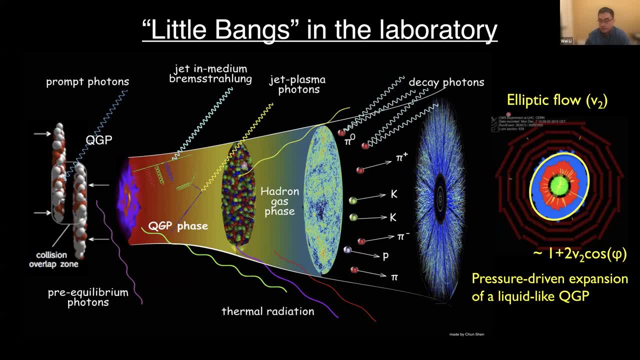 Pseudomagnetic norm-sensor, And we have discovered something very striking in the this type of collisions, for example, the well-known phenomena for elliptic flow, which is the the essence of anisotropy in the final state particle as well as distribution. 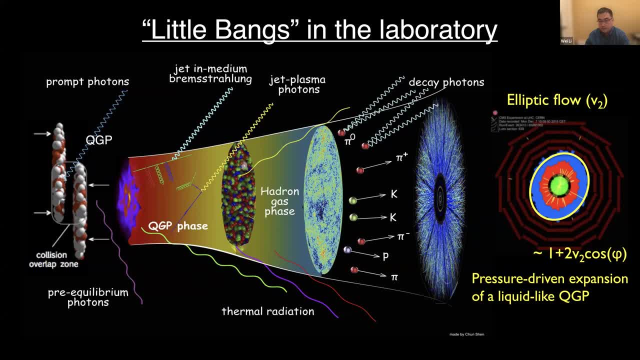 For example, here I show you one event display of the CMS experiment: the energy distribution. the calorimeter you can clearly see is the elliptic shape, cosine two phi energy distribution, And this indicates that we create a medium that behaves like a liquid. 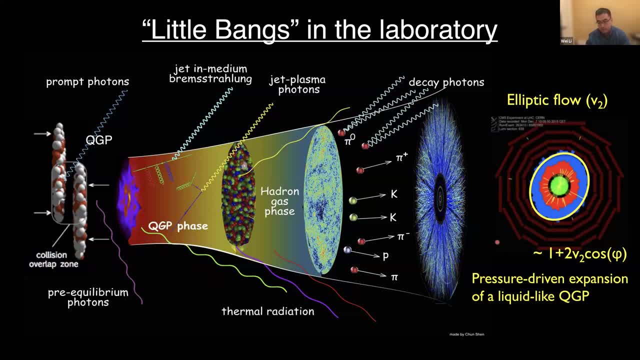 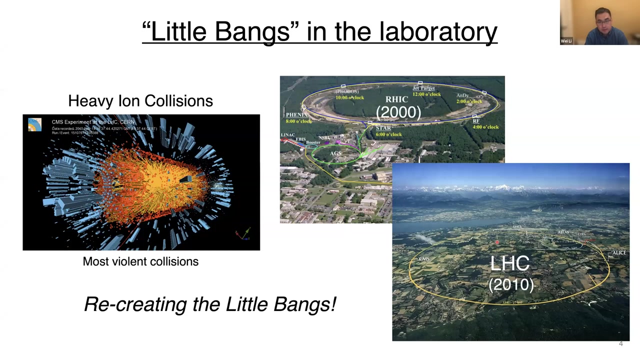 and expounds for a pressure driven function. And this liquid is very special because we found that it has a very little, very little viscous momentum dissipation, so that we call that a nearly perfect liquid. So there are two places in the world that we are creating these little events. 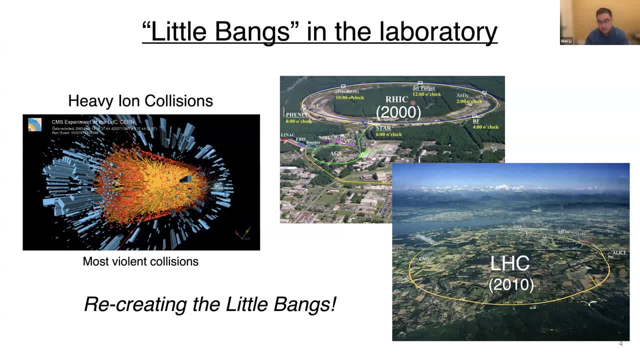 The first one is at the RIC. You heard about this last week already. The RIC started in 2000.. There were four experiments at the beginning, So right now the STAR is the only experiment that's still operating, And next year a new experiment, S-Phoenix, will come online. 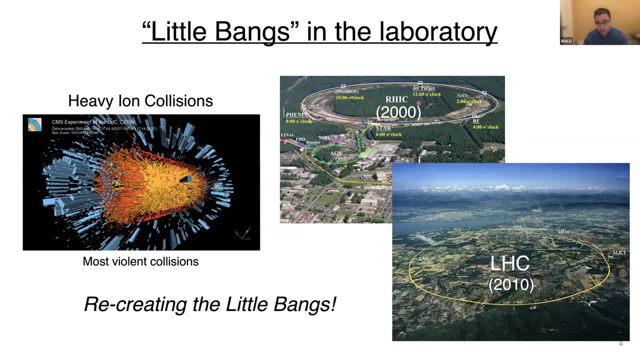 So RIC operates the energy up to 200 GeV, the same term as energy- whereas the Large Hadron Collider at LHC, which started 10 years later, collide also heavy ions at roughly a factor of 10 or 20 higher energy. 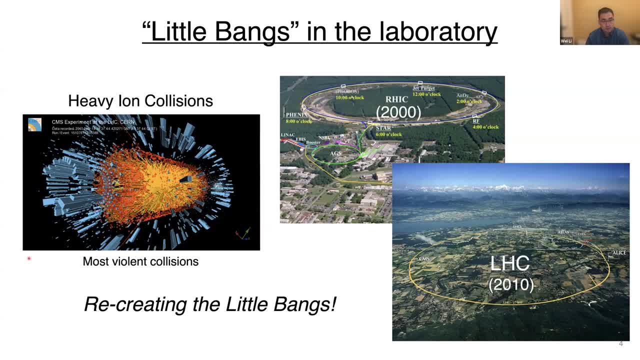 So this is an event display of the three-dimensional event display of CMS experiments. It was a very interesting experiment For head-on light-light collisions where we see tens of thousands of particles coming out of one collision. So these are the most violent collisions that we ever created in these colliders. 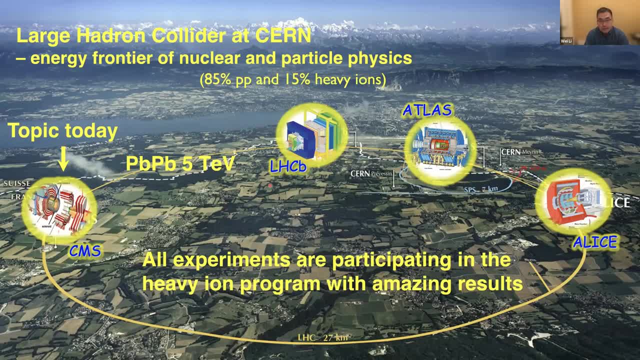 Okay, so Large Hadron Collider at CERN is the energy frontier of nuclear and particle physics at the moment, And so what it does is so about 85% of time every year it collides, Sometimes protons, protons. 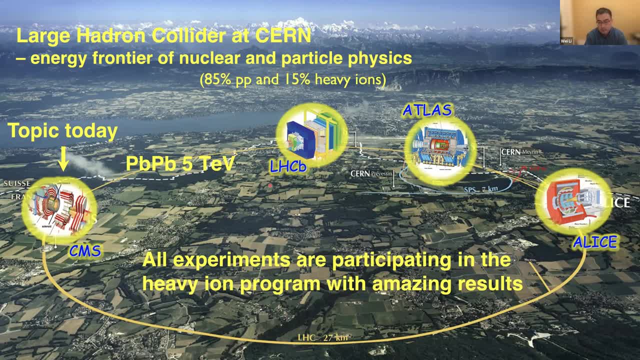 Whereas 15% of time it collides heavy ions, Light-light collisions, sometimes proton-light collisions. So there are four experiments: CMS, ATAS, ALICE and LHCb. ALICE is originally. ALICE is only an experiment that's designed for studying the heavy ion collisions. 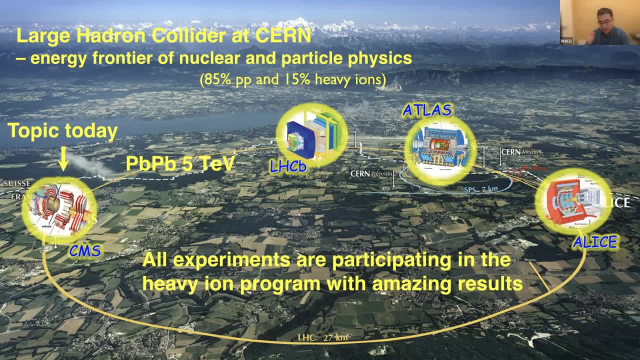 However, if you look at now, so all the four experiments are actively participating in the heavy ion program, And all with amazing competitive results. They are complementary to each other. So the experiment I'm working on is CMS, So this will be the topic today. 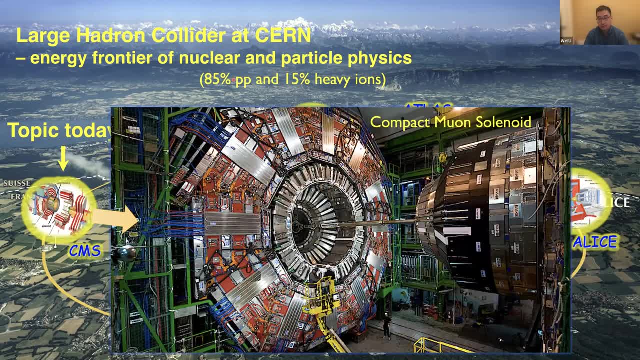 So CMS stands for the Compact Muon Solenoid. It is an enormously large apparatus. You can see the size of it. You can see the size of the person here, The CMS. so the diameter of CMS is about 15 meter. 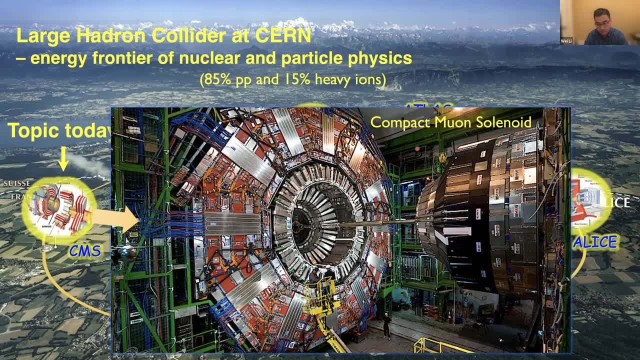 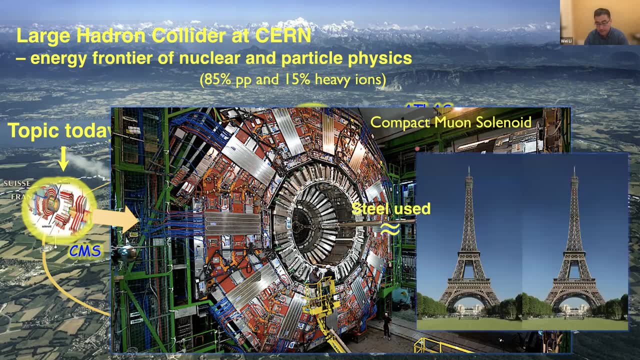 If you may be wondering why we call it compact despite the fact that it's so big, If you look at the amount of steels that are used in building CMS and that is roughly equivalent to the amount of steels used to use for two effort talks. 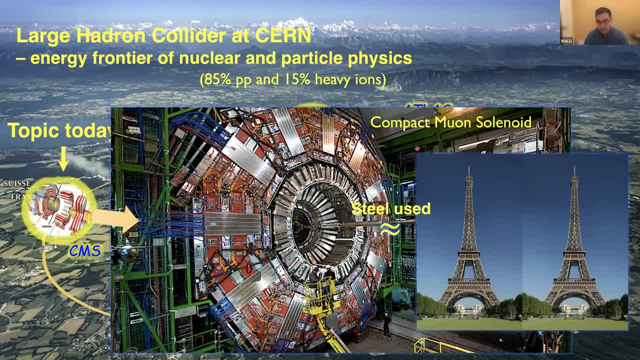 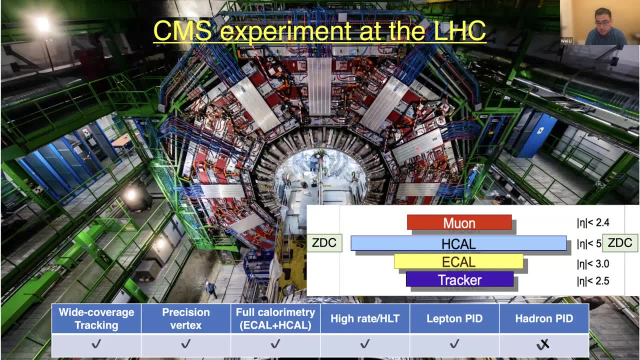 So in that sense it's really a very compact device. This is another view of CMS. To give you an overview of the capability of CMS, it's featured by the very large acceptance in solar activity coverage. Starting from the inner tracker it has a coverage of five units in eta. 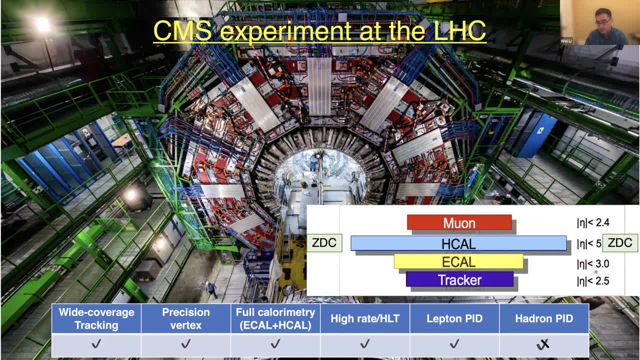 And then the electromagnetic calorimeter, which is a coverage of plus minus three units of ceta And the three units of six units in eta, And the hydronic calorimeter covers 10 units. In addition, there's also the zero degree calorimeter, that's 140 meters away from the interaction point. 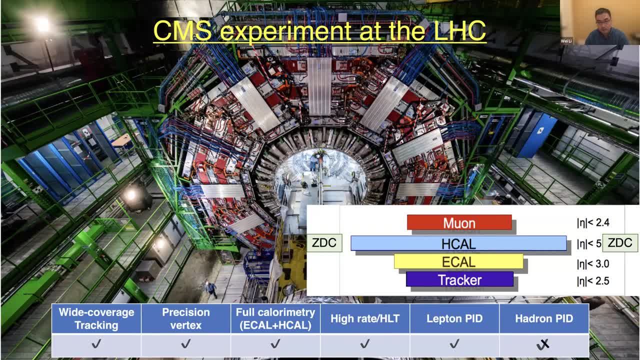 In the most outer layer, this red part, those are the muon system, which have coverage of about five units in eta. So CMS is featured by the wide coverage tracking Precision vertex from the silicon detector, Full calorimetry, the e-cal and h-cal. 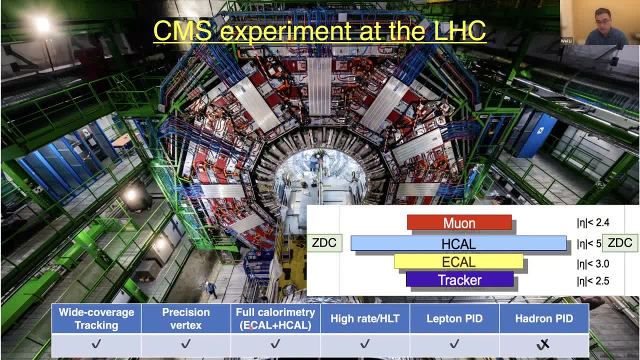 So that's very important for the jet measurements And it can take data at an extremely high rate And it has a high level trigger system that is very flexible. You can run the close to offline reconstruction algorithm to select events online. It has excellent lepton, TID, muon electron. 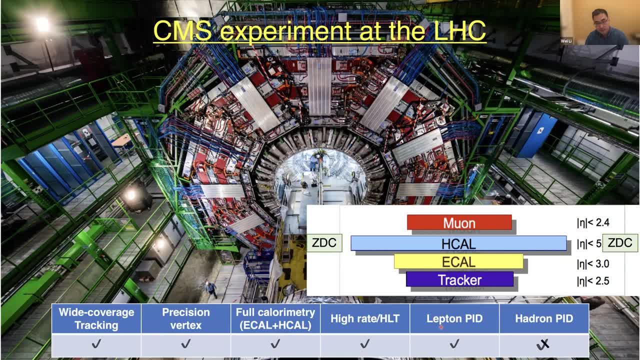 Photons And the hydronic TID is an area at the moment that is a weakness of the experiment. It's hard to build one detector. You can do everything right. So the hydronic TID, we can do some. 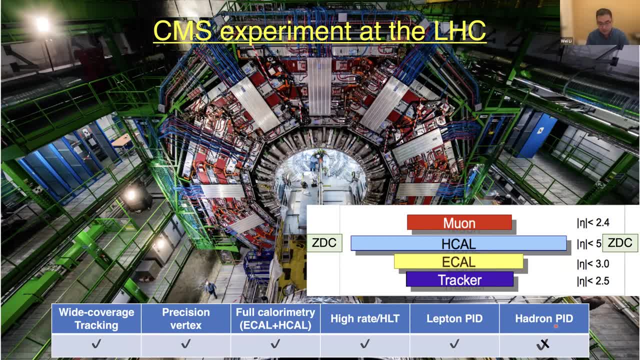 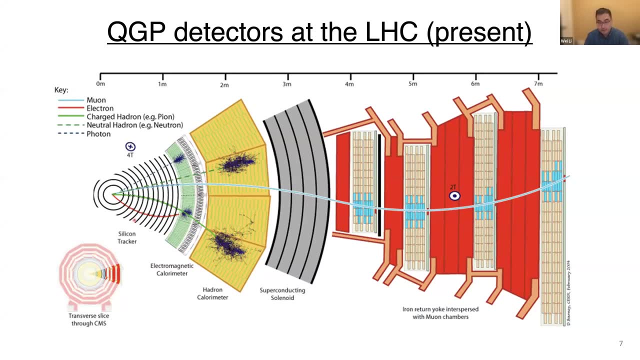 So I'll show you, But this is not the best among all experiments. But later I will talk about the upgrade that actually will improve that in the future. These slides give you kind of a glimpse How CMS detect particles and identify particles. This is a kind of a transfer. 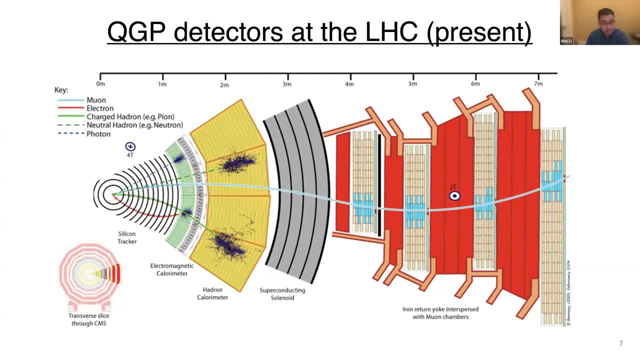 Taking a slice of CMS. Starting from the most inner part is the silicon tracker. It's inside a magnetic field, So once the particle is produced, the charge particle will get bent inside the tracker And then, when the particle reaches this layer, this is the electromagnetic calorimeter. 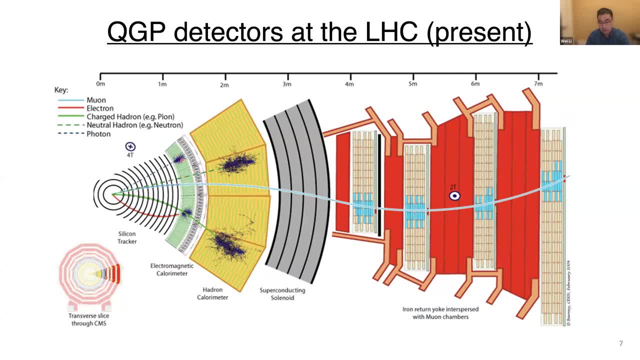 The electrons and the photons will be stopped. The other energy will be positive. This particle will be an electron because it can be connected to a track in the tracker, Whereas this one must be a photon because you don't find a track that connects to this. 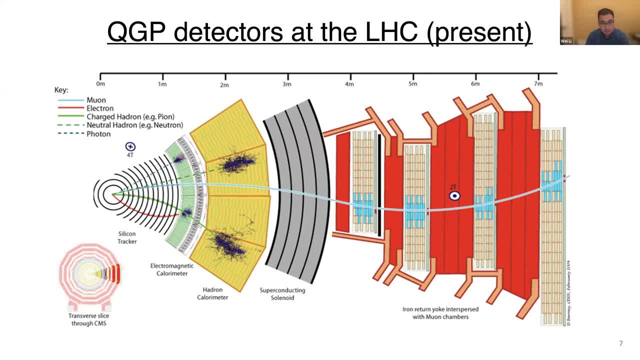 This way, you can tell which is which And then you'll reach this yellow part. This is the hydronic calorimeter, where the hydrons that will deposit all this energy In this sector. Similarly, if you can connect your energy cluster with a track in the tracker, it must be a charged hydron. 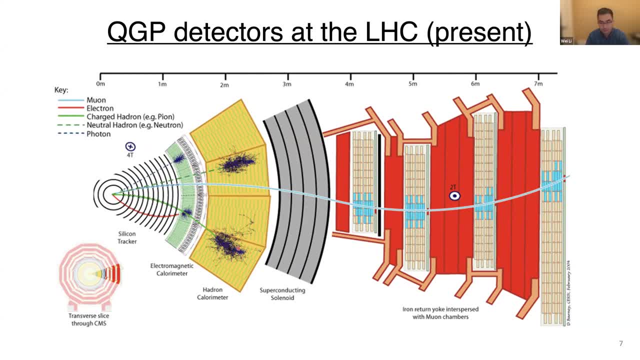 Well, we don't know whether it's a pi on, k or proton, But we know it's a charged hydron, Whereas if you don't find a track, then it's a neutral. It's a neutral pattern, It can be a neutral, for example. 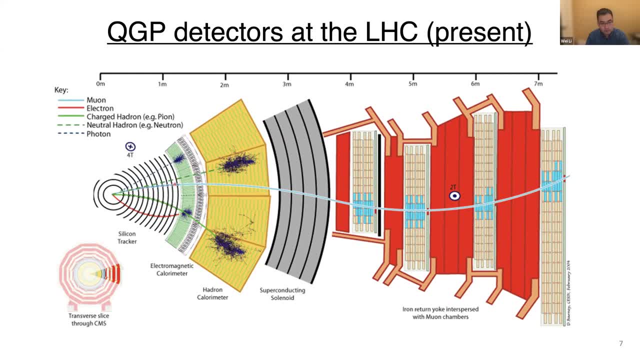 And then this kind of cyan color line that goes all the way through To the entire detector. this is a muon. This muon is like the heavier chasm of the electron, And it's much heavier. It can go through a lot of material. 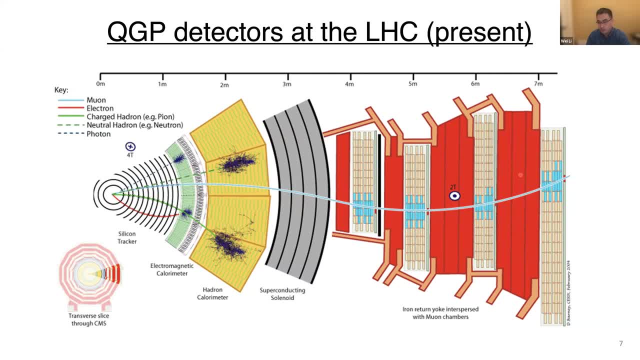 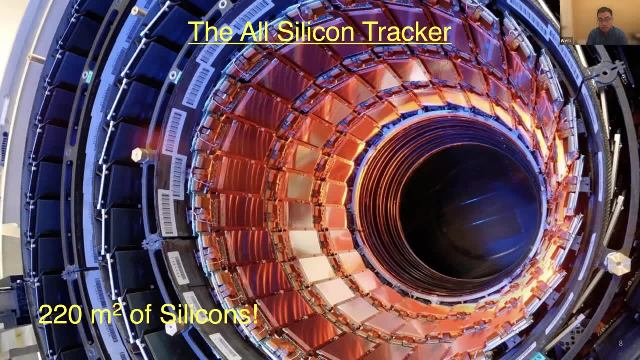 And so we put the detector in the outermost part of the detector to detect the muon. OK, so next I'm going to go through all the major detector subsystems in CMS And I'll start with the CMS. In the tracker, this is an old silicon tracker. 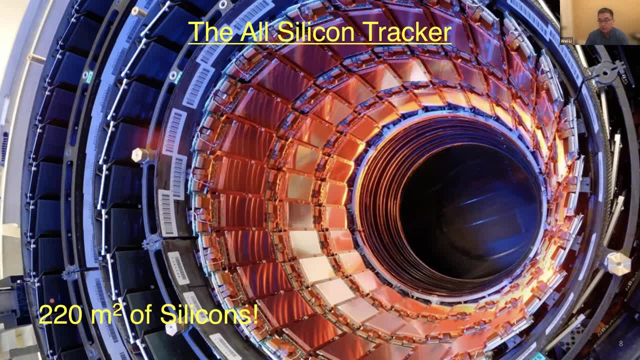 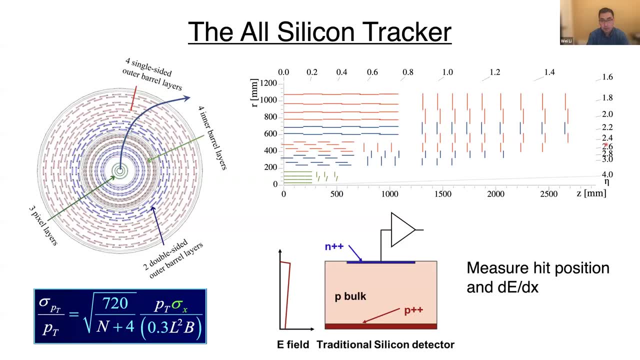 It has used a total area of about 220 square meters of silicon And this is the world's largest silicon tracker. So the old silicon tracker is in the transfer cell. You see there are many layers. In the innermost is the four layer pixel silicon pixel tracker in the barrel part. 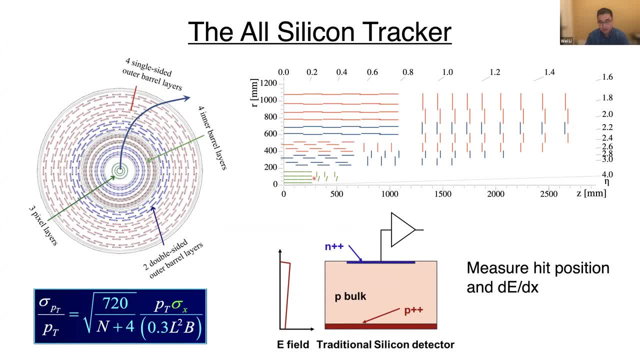 And there are three layers for the end cap. So these are the pixels And then the outer layers where you have to cover a larger area, And then we switch to the silicon strip detector, The long strip, roughly a few centimeters long strip. 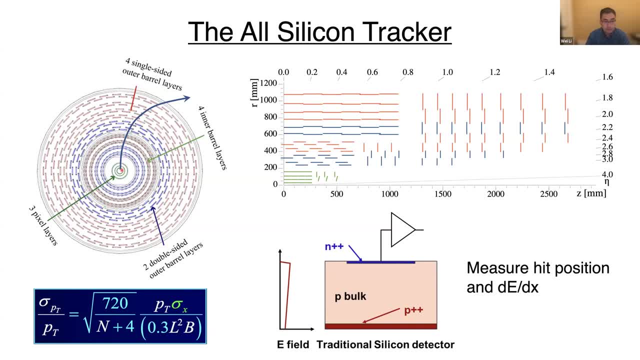 So the idea of the tracker is you know you have a particle in the band by the magnetic field When it comes out, the charge particle, And you measure its curvature and you can measure its momentum. So this is kind of a pocket formula that you can compute the momentum resolution that you can determine from your tracker. 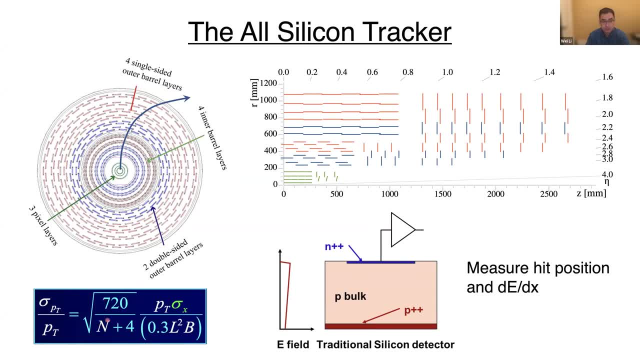 which depends on how many points you can measure. So in CMS we can measure up to 20-something points, Whereas at least TPC you probably have hundreds. It depends on the PT itself, It depends on the resolution of individual hits. 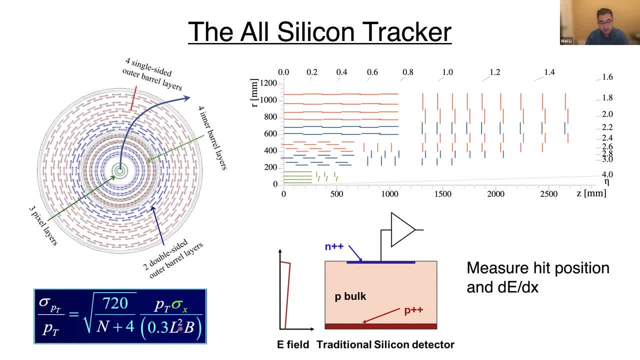 And it depends on the total length of the tracker, Like the radius of the tracker, And it depends on the magnetic field. The stronger the magnetic field, the better the momentum. I'll just quickly remind you of how the silicon detector works And basically you have, like, the PN junction with the bias voltage. 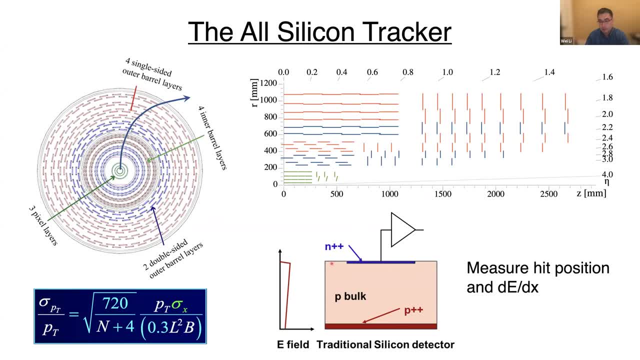 This is the bias voltage applied so that you create an electric field in this active volume of the silicon sensor And when there's a particle comes through it will create ionization of electron and hole pairs And then under this electric field- internal electric field- the electron and hole pairs will be drift toward it. 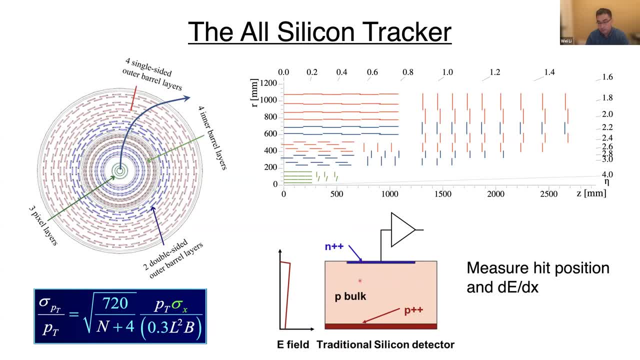 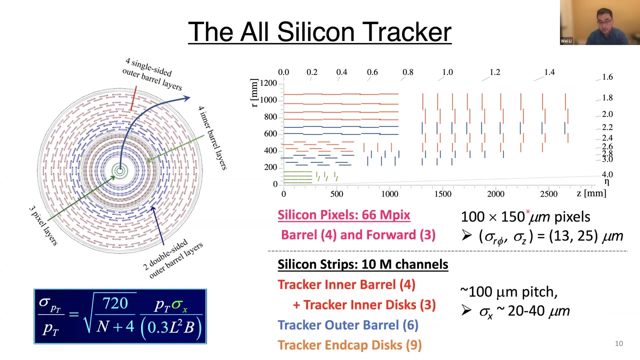 For example, the electrode here, which will get collected as an electronic signal As a silicon detector. the advantage is that it can measure the heat position extremely precise And it can also measure the energy deposition per unit distance, like BEDX. So the pixel detector has a total of 66 million pixel channels. 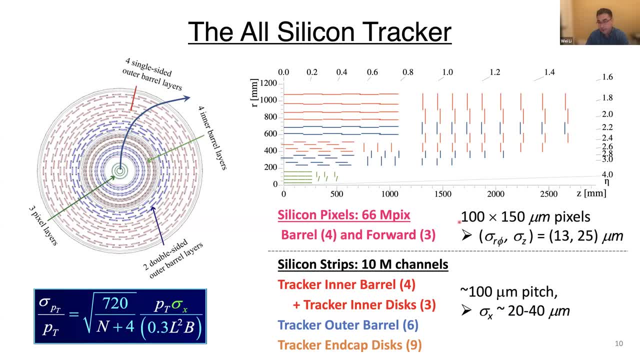 It's a lot of channels, And so each pixel is 100 by 150 microns in size, So that provides you a position resolution on the order of 10 or 20 microns, So very precise, And whereas the silicon strip, that is the outer part, has a total of 10 million channels. 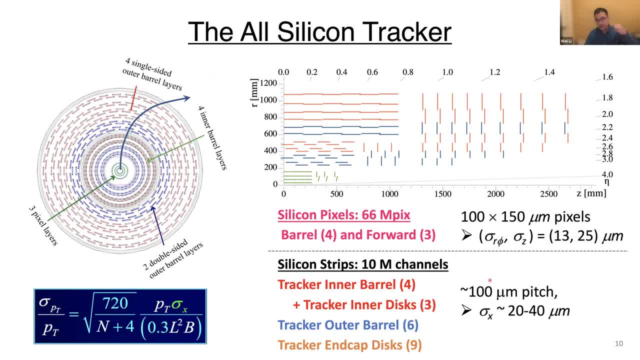 And the strip is about a few centimeters long And it has the pitch size and the distance. The spacing between each strip is about 100 microns. That gives you a position resolution on the order of 20 to 40 microns. 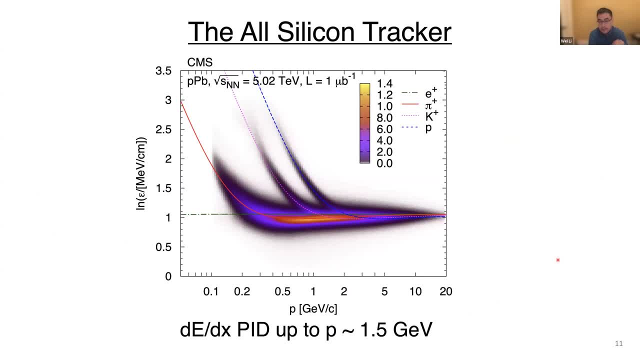 Yeah. So let me, because the topic of today's PID. so let me show you that we can use a silicon tracker to do PID through DEDX And DEDX as a function of PID, It's a function of momentum. 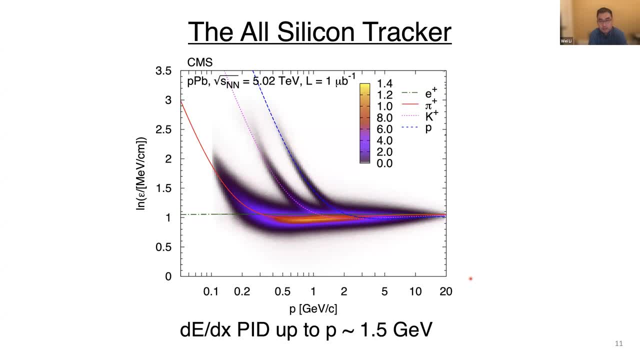 But DEDX here is measured by combining the silicon pixel and the strip detector And it's actually not trivial. That combination is not trivial. You need different calibration of the detector. That's a lot of work And here you can also see that compared to the TPC, the DEDX, as you've seen last week right. 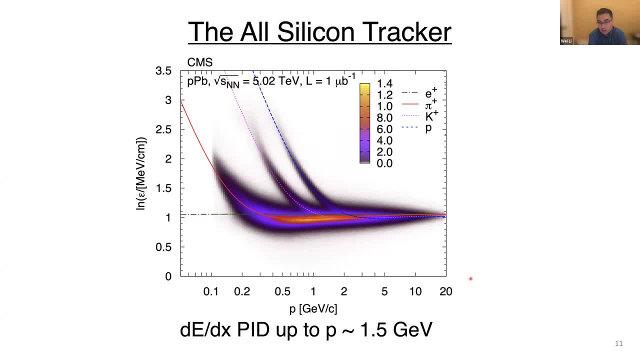 Our DEDX is not as good as TPC. The one reason is because in TPC you measure the PID. In TPC you measure up to 100 points, right In star probably, I think, tens of points. 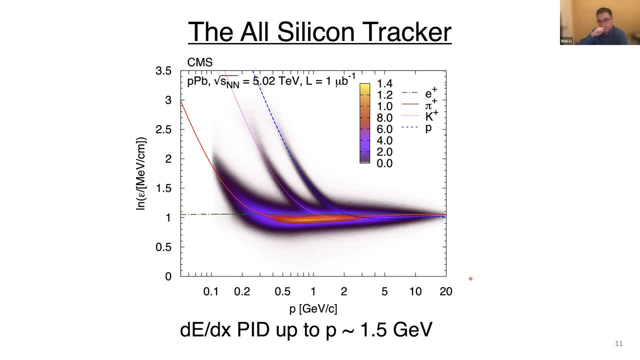 And at least you can get 100 points, So you average over 100 points, Whereas here so we measure like 10 or 20 points. The resolution is not as good as what you get, at least in star, But we can still clearly see the separation of pion, kaon, proton up to something like 1.5 GeV. 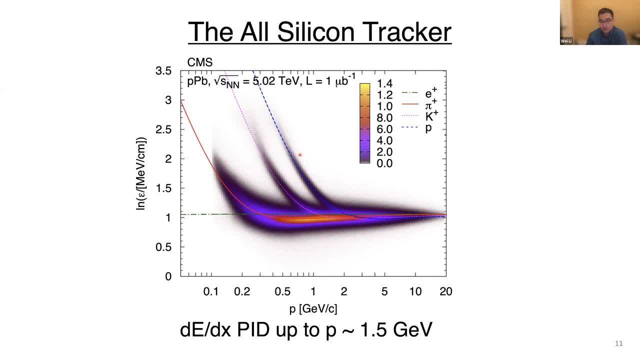 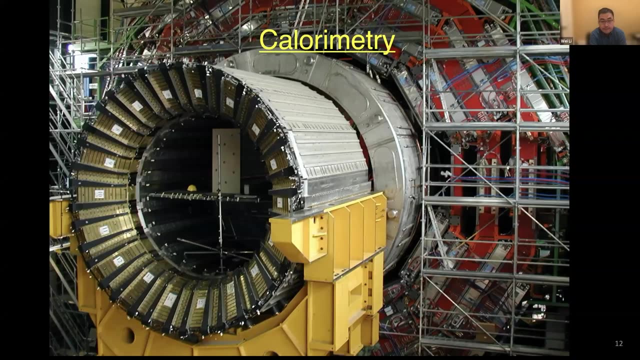 For protons. So that still gives us some PID capability to do some. This is in proton-led conditions, Okay, So next I move on to the calorimetry. The calorimetry consists of two parts. One is the electromagnetic calorimeter and the hydronic calorimeter. 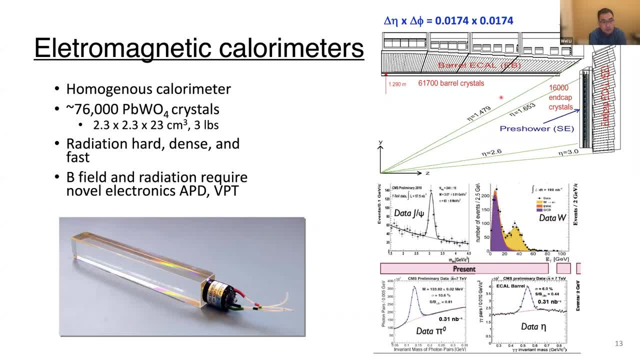 I'll first tell you about the electromagnetic calorimeter. So in CMS it's homogeneous And we use the last tungstate crystal. You can see this is the crystal bars And its length is 23 centimeters long And the transfer area is 2.3 by 2.3 centimeters. 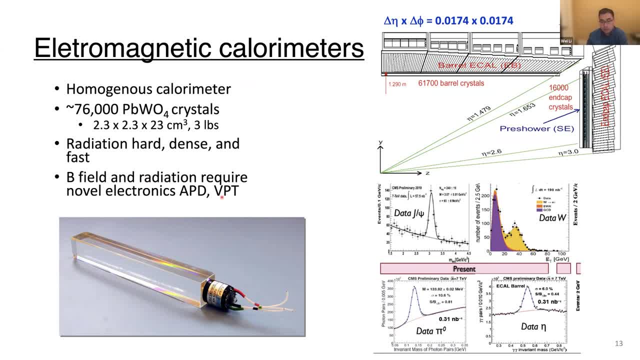 Each of these crystal bars weighs about three pounds. It's pretty heavy because it's a very dense material, And we have in total, about 76,000 of these light tons in the crystal bars And they are arranged in this configuration. 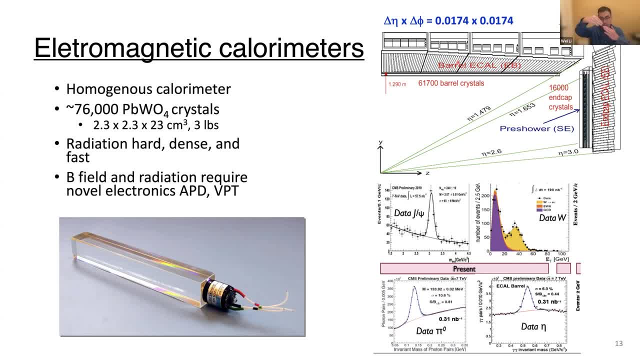 You'll see they are projectile to the interaction point, So you measure the total energy of the parts of the photon, for example, Or electron, Instead of the transverse energy. So they are designed to be radiation hard And they have very fast response. 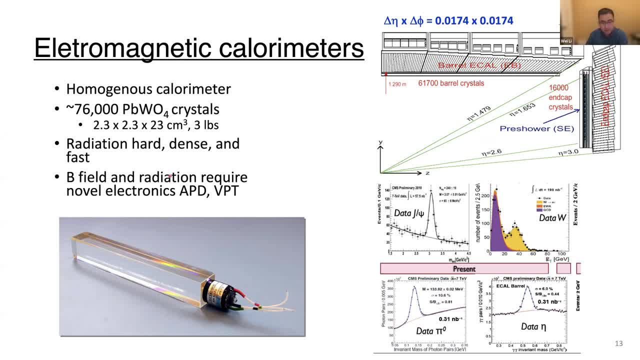 And they have to Tolerate a very strong magnetic field. So the readout electronics are important. So you can't use PMT Because they will not perform well in the high B fields. Therefore we use, for example, APDs, avalanche photodiode. 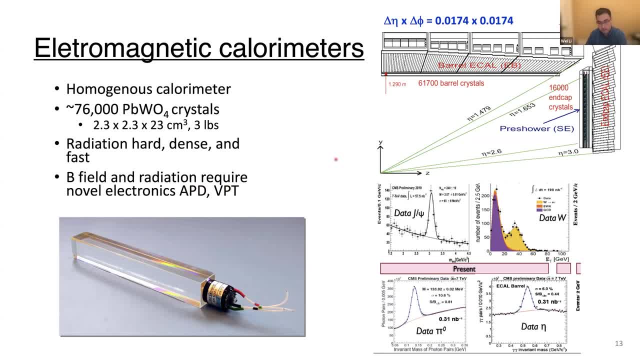 and VPTs and similar technology, Photon sensors that are very compact. So in any case, so with the EMTEL we can identify photons And we can identify electrons With the electrons here this is a drip site, peak from the E plus E minus. 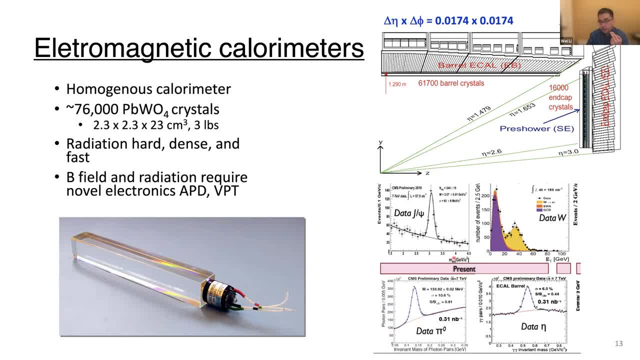 environment, mass distribution And we can use electrons to identify W. The high energy electrons, about 20 Gbd, mainly come from W decay And with the two photons we can reconstruct the pi zeros. That's a clear, nice pi zero peaks. 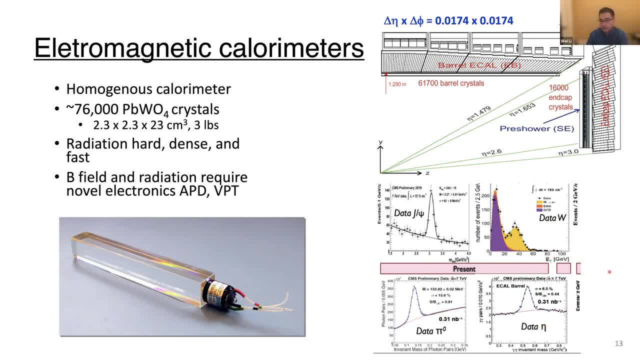 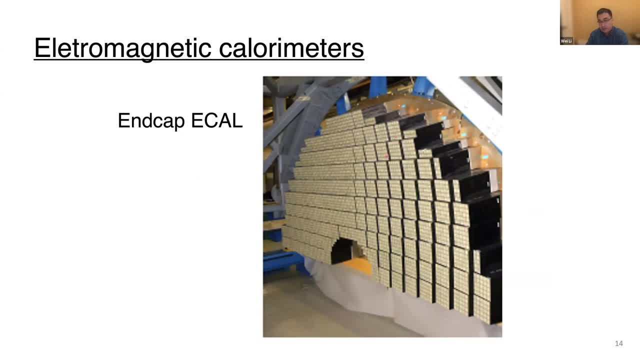 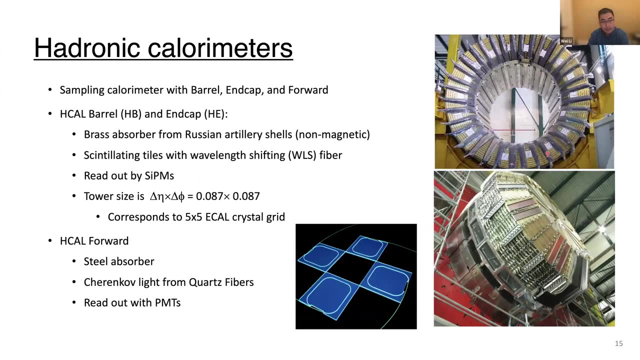 And also particles like eta. This is a picture of the N-CAP- electromagnetic calorimeter. You can see how these, all these crystal bars are arranged. The N-CAP sensor- Hydronic calorimeter, is a sampling calorimeter. It has three portions. 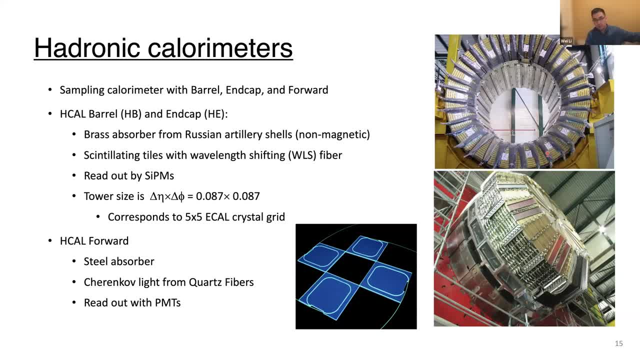 There's a barrel, the N-CAP, and then there's also four hydronic calorimeter. So the barrel and N-CAP use the same technology. So there's a first the energy absorber is made of brass, And then, after the energy converts, 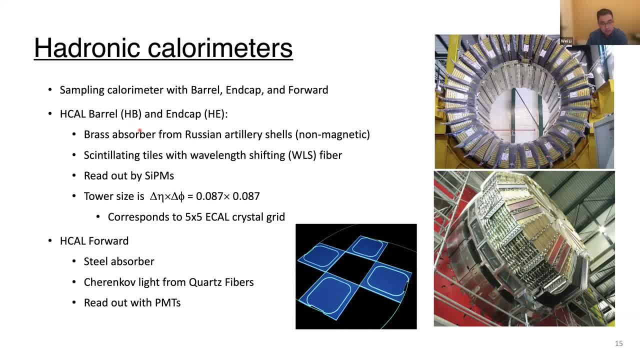 into showers and generating the scintillating light. the light will be collected by the scintillating. there will be this scintillating tile That will generate the light. that will be collected by these through the wavelength shifting fiber and, in the end, 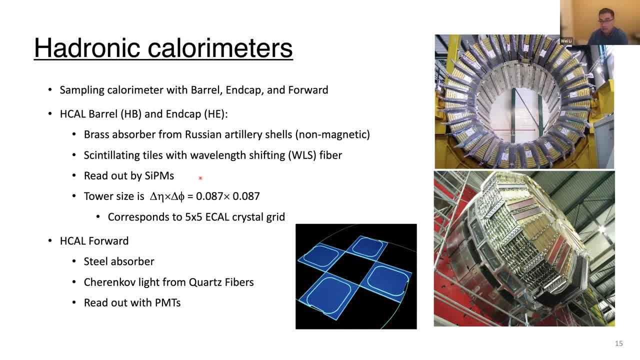 collected by the silicon photon multiplier tubes Again, which can function within a very high magnetic field. The granularity of the- the hydronic calorimeter is what we call a tower- is about 0.087 in both in the eta and the phi direction. 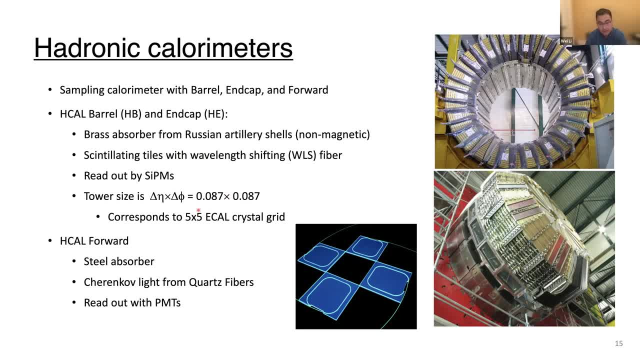 And it corresponds to roughly about five by five Ekl crystal grade. So the electromagnetic calorimeter has about five times better granularity than the hydronic calorimeter, And there's also the further forward hydronic calorimeters. It's made out of steel absorber. 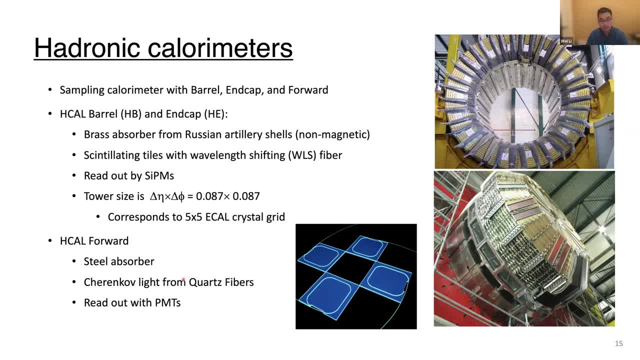 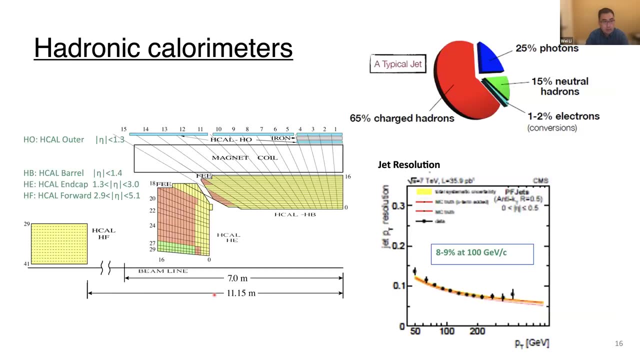 which will generate this training of light And read out by the PMT, the photon multiplier tube, because the H-cal is outside the strong magnetic field, So you can use PMT. Yeah, so this is the side view of the H-cal. 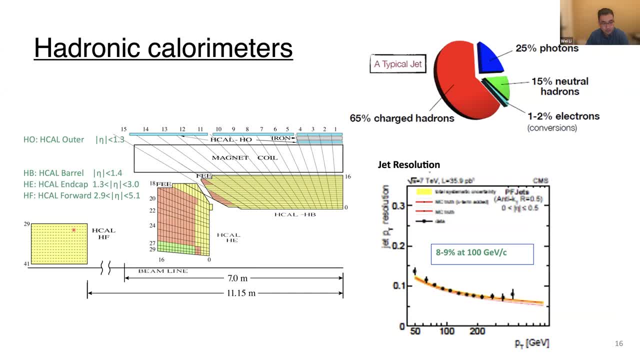 as the barrel end cap forward. So the H-cal is most important to measure jets, for example, And if you look at the particle composition of the jets, so 65% of the jets has the charged hydrons. You can measure those. 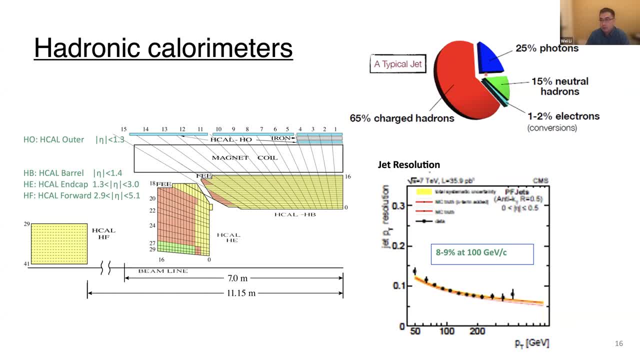 from the tracker right, So you don't have to have the calorimeter. 25% is the photons. You can measure those photons through the E-cal, without H-cal, But you see there are. there are 15% of the neutral hydrons. 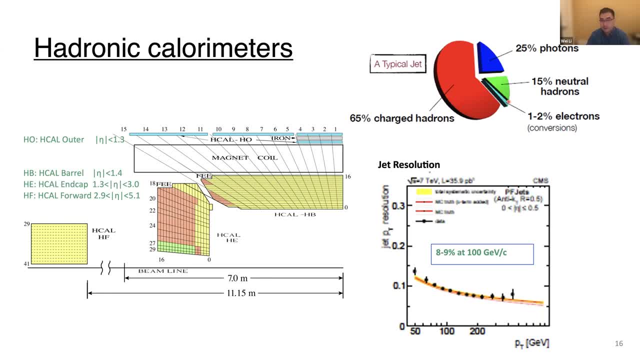 that you can only measure with the hydronic calorimeter. 15% is quite substantial fraction, right? So if you are not able to measure them, you are not going to get the best resolution of your jet energy reconstruction. So apologies. 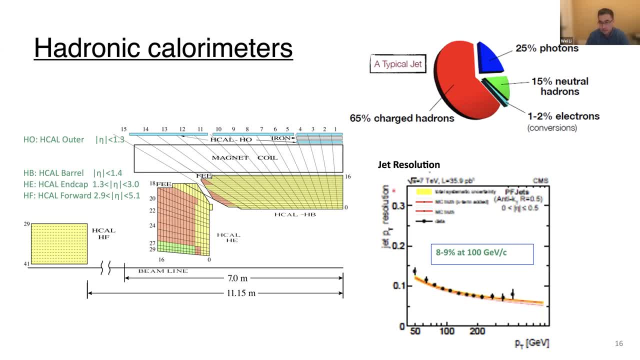 this plot somehow is fuzzy, but this shows you the performance for the jet PT resolution in CMS as a function of jet PT And you can see that in general it gets better and better as you go to higher and higher PTGS And we get about 8 to 9%. 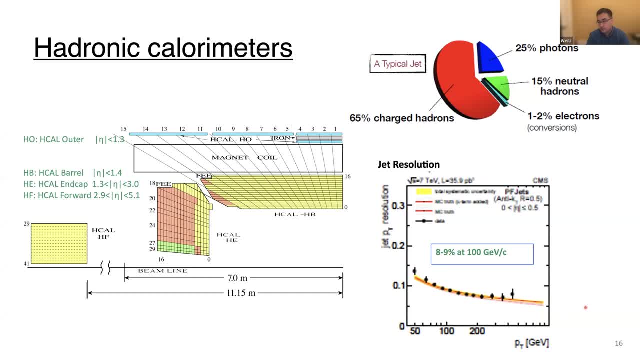 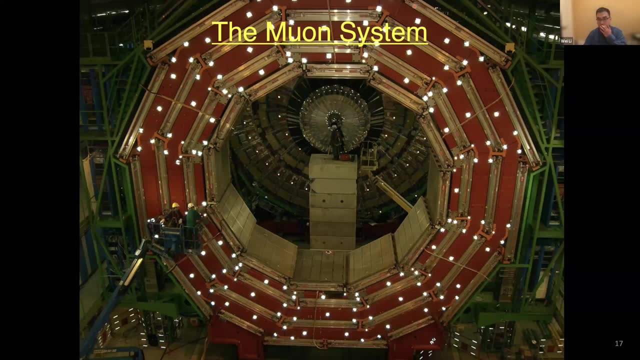 at 100 GeVgs and be better, much better, for 700 GeVgs. So here the hydronic calorimeters play a very important role. Okay Now. next, the muon system is. I'm just keeping my eye on the time. 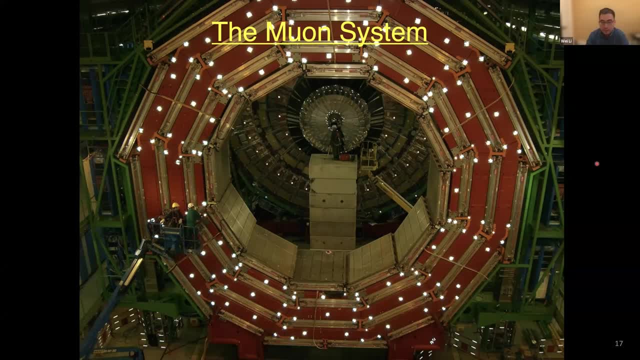 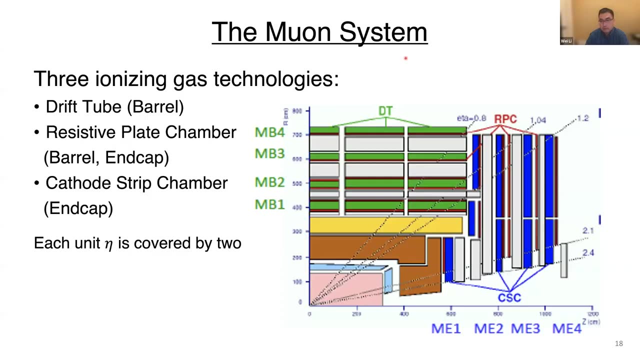 The muon system is the most altered part of the detector And so the muon system. actually, we use three different technologies, three different ionization gas technology for the muon system. Yeah, I can give you a long story of why we. 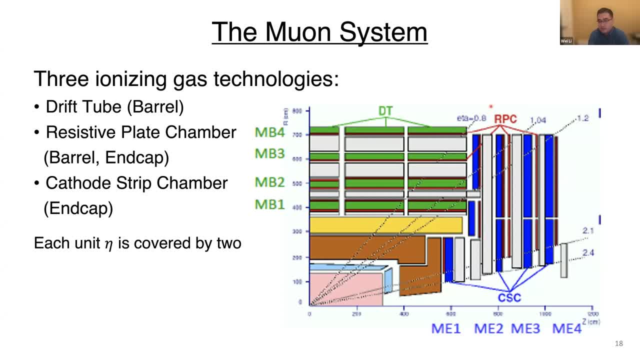 CMS arrived at this choice of three different technologies, But long story short is is mainly driven by the the fact that the occupancy you have to handle is different in the central region versus forward, and also to have the redundancy, have different technologies. 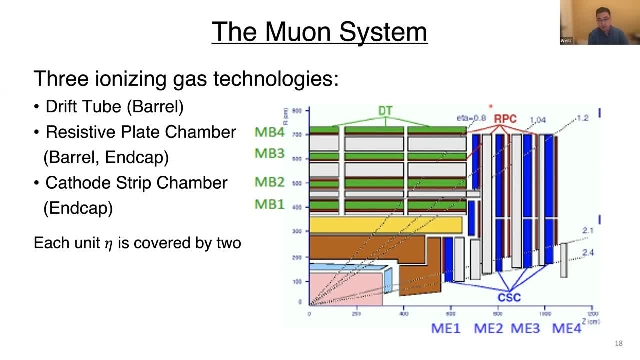 Remember, CMS was designed 30 years ago. So and at the time there is there are uncertainties with certain emerging new technologies and to make to increase the redundancy, The decision is that for every unit, eta is covered by two different. 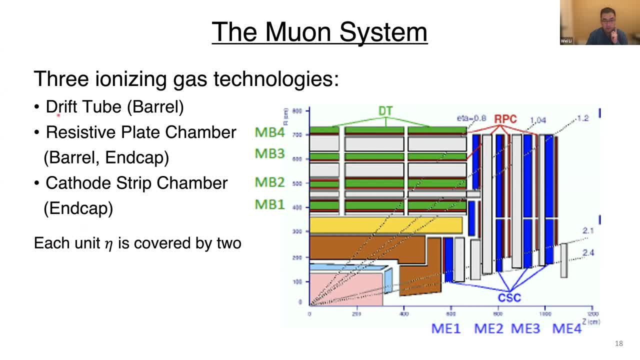 technologies. So in the barrel region we have the- it's called a drip tube, And then the resisted plate chamber is installed in both the barrel and end cap And then in the end cap region there's also this castle strip. 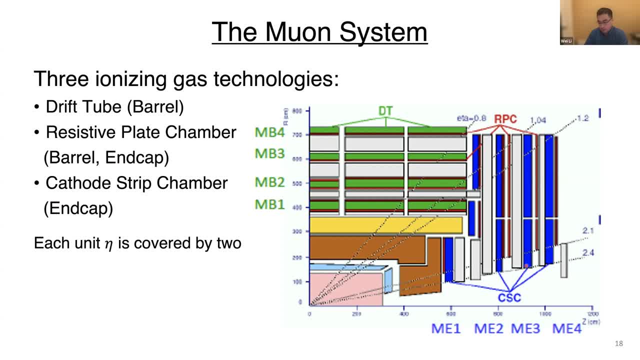 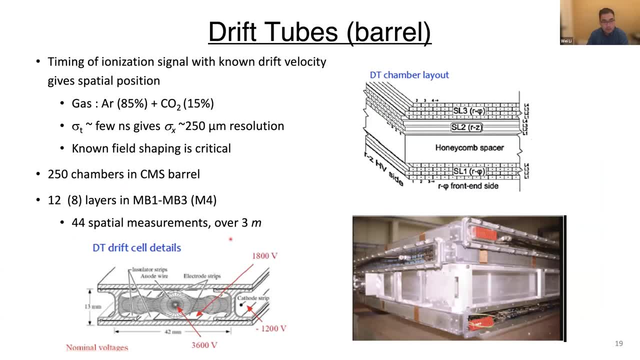 strip chamber. So I'll quickly go through the these three technologies, but maybe not all. all details And the drip tube, I think the best way to look at it. in this picture you'll see it's a small chamber. 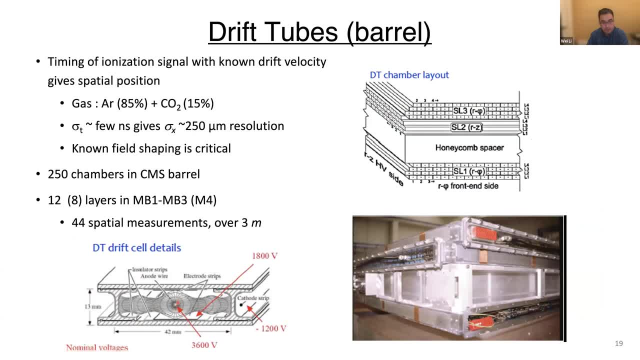 a small tube where you have, in the center of the tube, you have this electrode, you have this anode wire, And then you have the electrode strip on the edge And then you apply the high voltage and you generate this electric field. 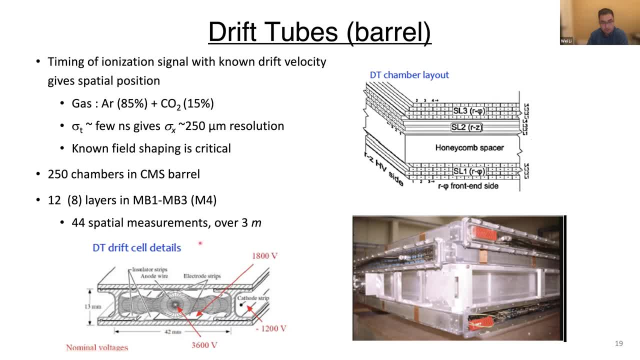 These are electric field lines After the ionization. so the, the ionized charges will be drifted toward, toward anode and electrode, so that the signal gets collected right. So you'll see. so this little rectangle is the. 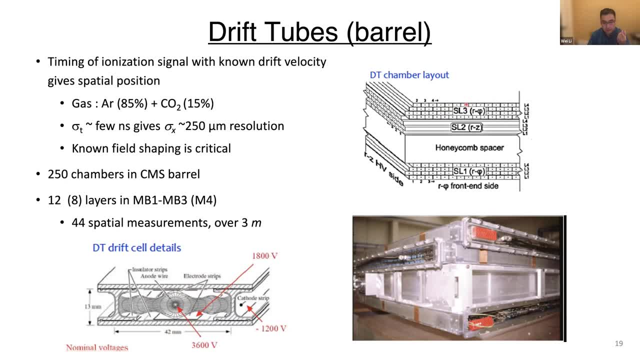 each of them is a, is a cell. It's one cell of drip tube. So yeah, many of so. we can measure the position you know, through the different cells and then do the track: reconstruction of the muon tracks. 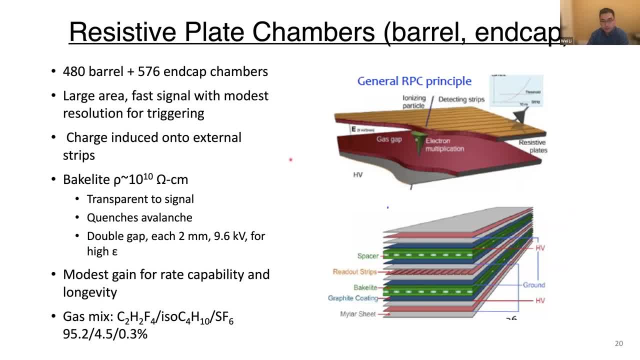 The resisted plate chamber is actually. it was installed mainly because it's it's fast and it can provide us the good trigger. can be used as a good trigger detect And the way it works is is very similar to is basically. 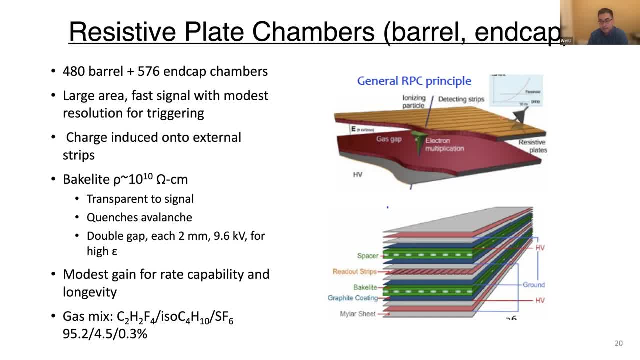 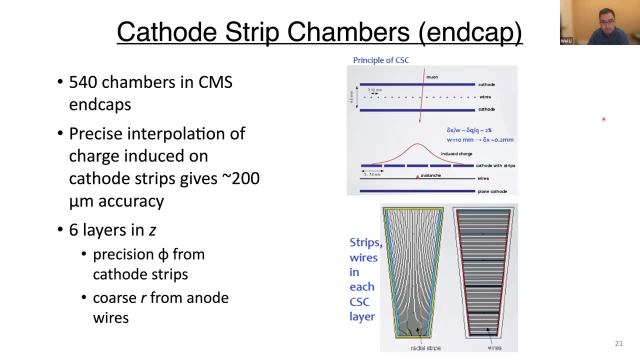 how the gas detector works and that that it, it detect, collect induced charges right. So the it and that one is the target of to the muon track. So that's my final answer. So for the 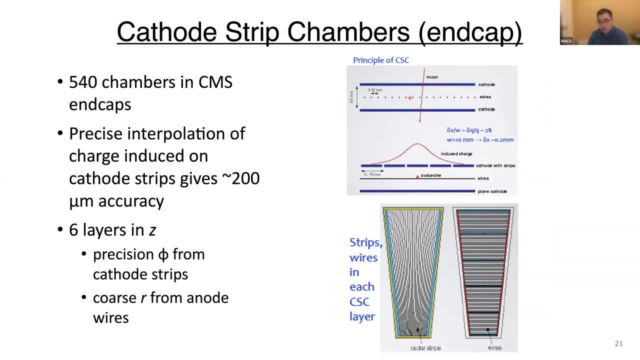 whole expression of the muon track. So you can see that this the muon track, is this the muon So strip and a wire. you create avalanche. you measure the induced charges Here in this picture you'll see these are the strips. 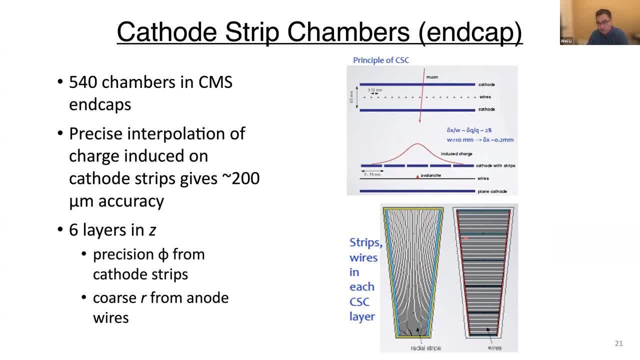 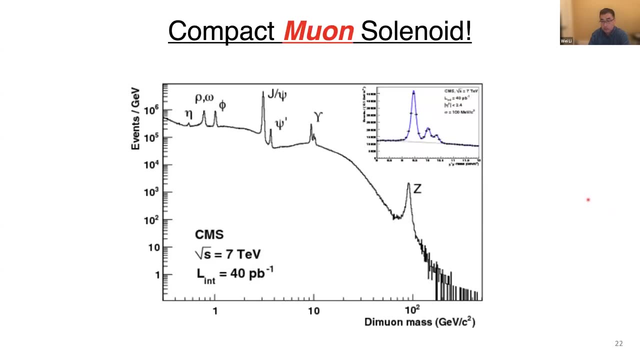 in each CSE layer. These are the annular wires going in this direction, in the five direction We have. in Z direction we have six layers on them, So each muon track will measure multiple points. So the muon is really, because of this, different. 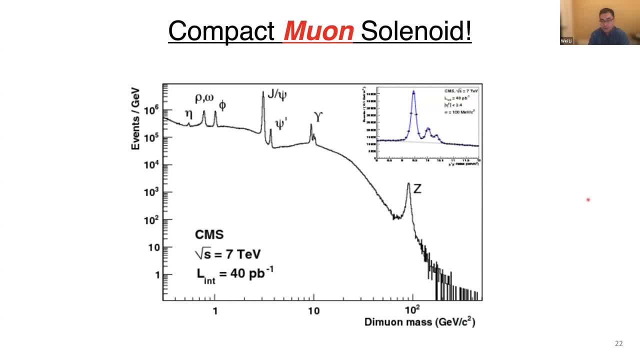 technology and redundancy that built in is really the strength of CMS detect. It has the best muon capability of all the LHC experiments And it's demonstrated in this plot, which is the eumary mass of the dimuon and where you can see that all these peaks. 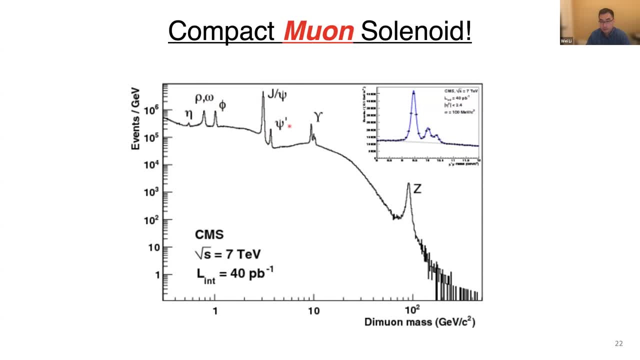 from eta rho, omega, phi, j, psi, psi prime. So oops on the three families members, oops on 1S, 2S, 3S, all the way to Z, So we can clearly identify all of those targets. 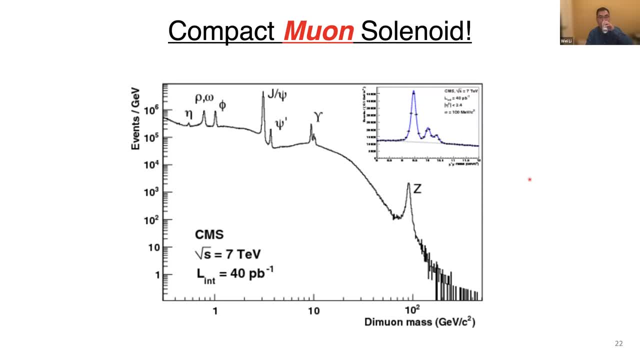 We do a lot of physics with them. Okay, so up until here I've gone through the technology of the detector and some of the basic performance, And next let me tell you about some of the performance. I will tell you about the physics. some of the physics. 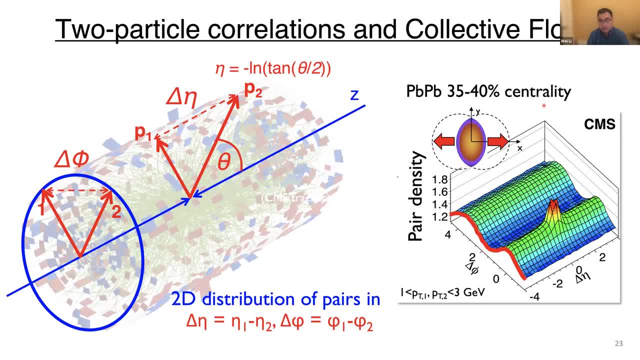 And I want to focus on to discuss the two pilot correlations and the collective flow phenomena in Heimlich calculations. I believe you have background of that already. So in CMS we do a two pilot correlations in the two dimension, in both in phi and eta direction. 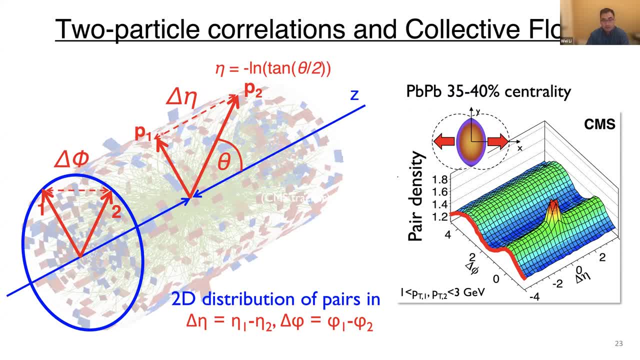 So you take two particles, you calculate their eta, delta eta and delta phi of the two particles and you'll form a two dimensional distribution of pairs in delta, eta and delta phi. And this is what we see in a peripheral light-light collisions, where we see well, first of all, 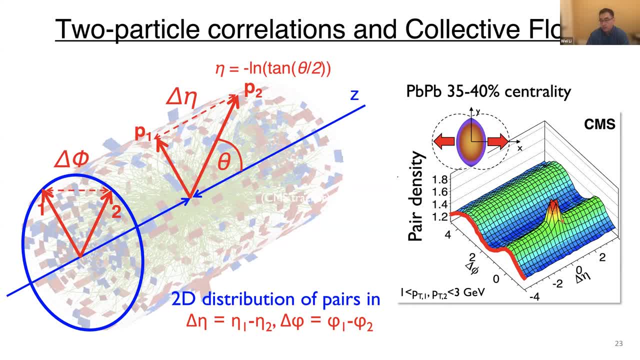 there's a peak at delta, eta, delta, phi, around zero, and that's come from. when you produce a gist or mini gist, they will fragment into many particles and they're all very close in eta and phi. And then, in addition to that, and you'll see the most striking feature, 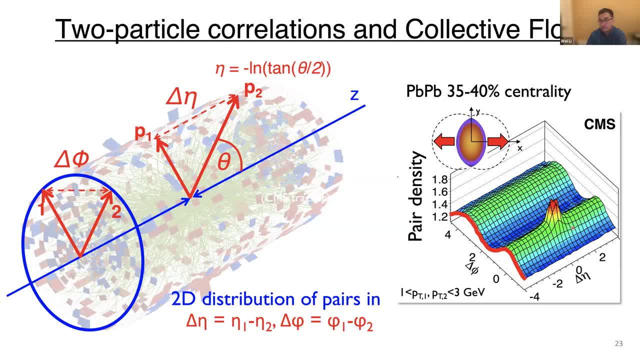 is this long range structure, The long ranges structure that's almost flat in delta eta and in delta phi. there's this cosine two phi structure that come from elliptic flow like this: This is my favorite way to observe elliptic flow because it really shows you this is a global effect. 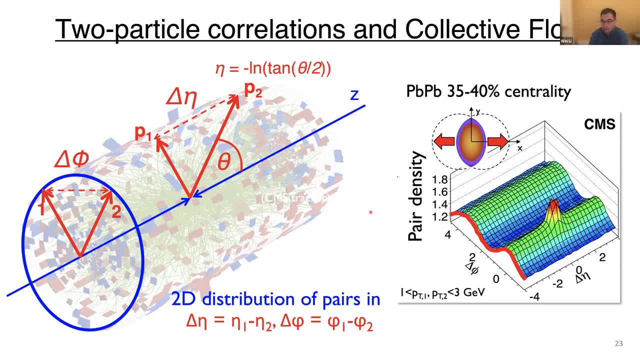 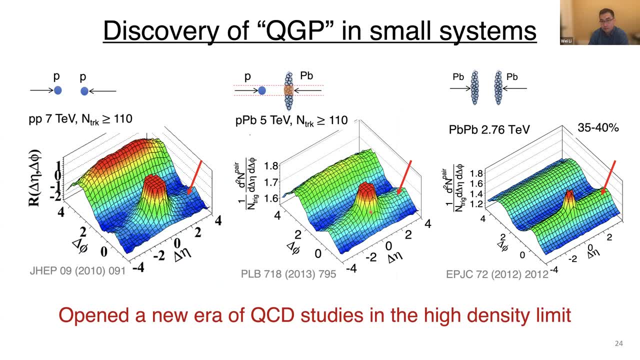 It shows you, It extends over the impair to the rapidity. Quite strikingly, you know, at the beginning of the LHC program we observed that so that this elliptic flow structure, this long range correlation, can also be producing the proton-proton collisions. 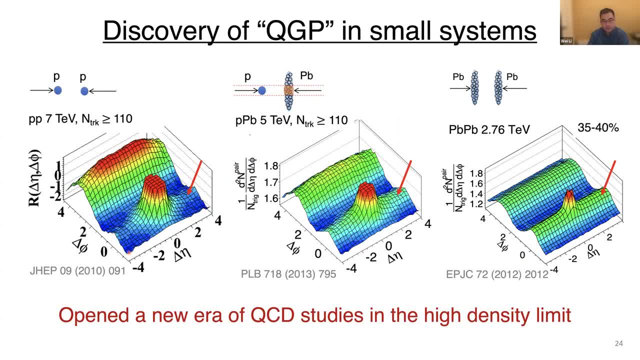 And a couple of years later, also in the proton-light collision. Well, they are smaller in fact, but yeah, fairly significant, And over many years of study, we made you know, over many years of study, over many years of study, we made you know. 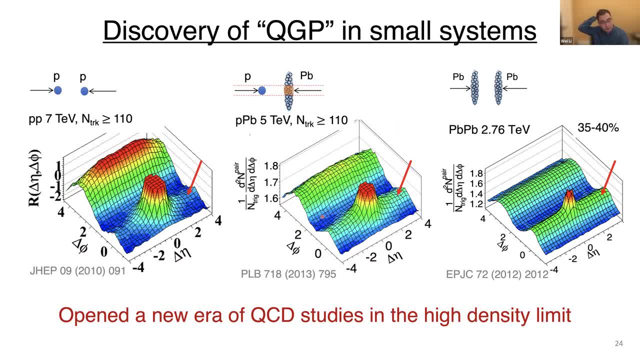 we made a lot of progress and a lot of we have understood a lot of what is really happening with this long range correlations in this small system. But this really opened a new era of QCD study in this very high density limit. So just one moment. 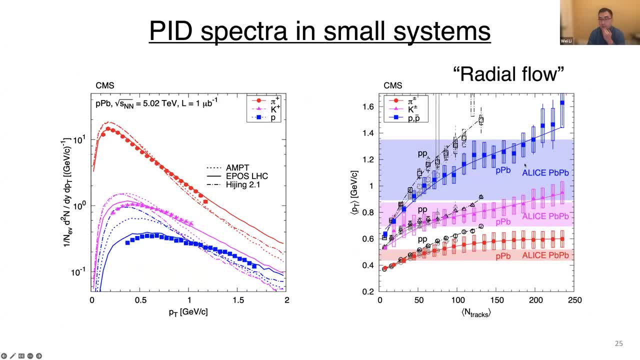 Yeah. So I want to show you some results that we use PID. So one is we measure the spectrum, the PID spectrum, in P-light collisions And this is- this is the pi and k on proton spectrum that we measure P-light through the DEDX, through DEDX. 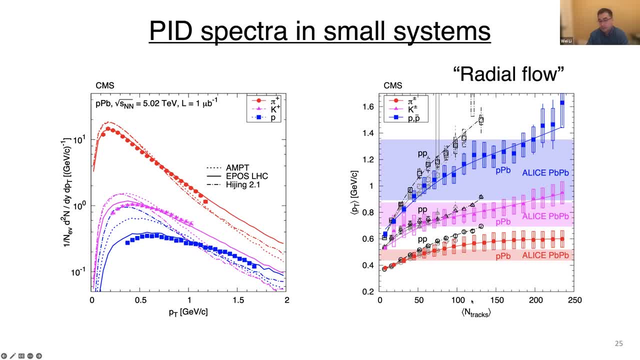 And we also measure the pi, kp spectrum as a function of multiplicity where we see. so in this, on both P-light and light-light, we see that the increase, the increase, the mean PT, the P-increase with the multiplicity, 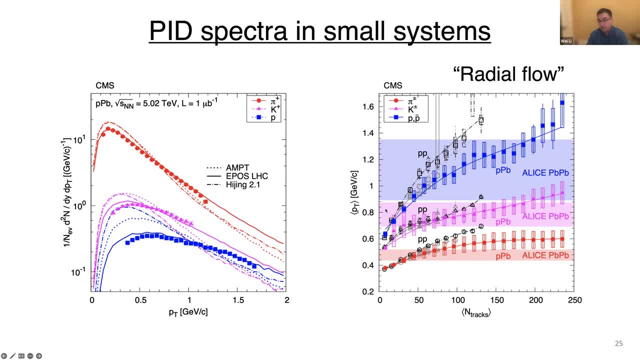 And in a way that the increase is faster for the proton, the heavier particles than the lighter particles, which is kind of indicate the effect- what we call the radial flow effect- that are observed in the high-velocity. So we can also identify neutral hadrons. 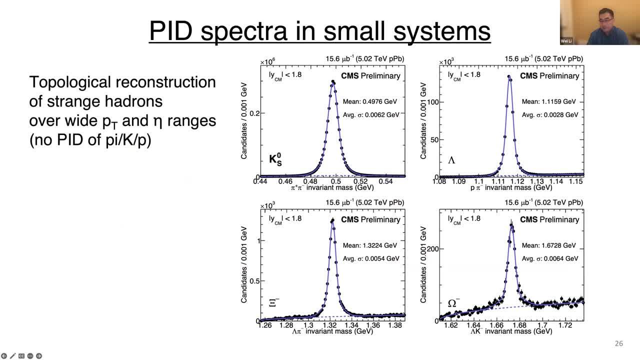 such as k-zero shot, lambda, cascade and omega. so we can also identify neutral hadrons such as k-zero shot, lambda, cascade and omega through their topological decay. So these weak decay hadrons, we don't need the PID of pi and k and proton. 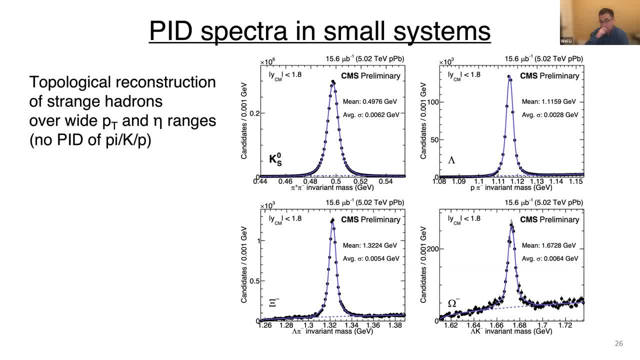 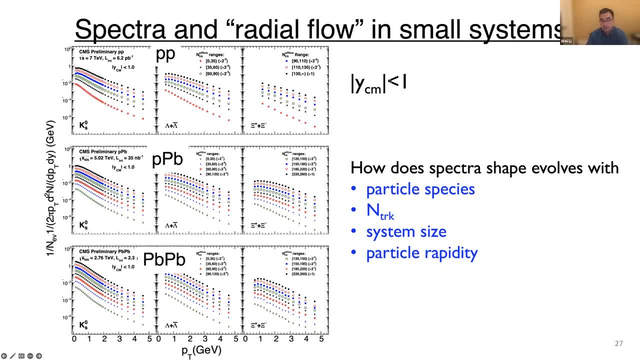 but just from the silicon tracker they reconstruct the vortex. We can nicely reconstruct all these peaks And we have measured quite comprehensively in small system the spectrum of the k-short lambda cascade and most recently also omega. in this is the middle rapidity in different systems. 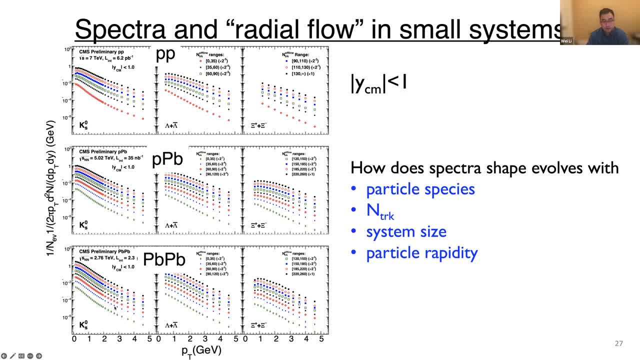 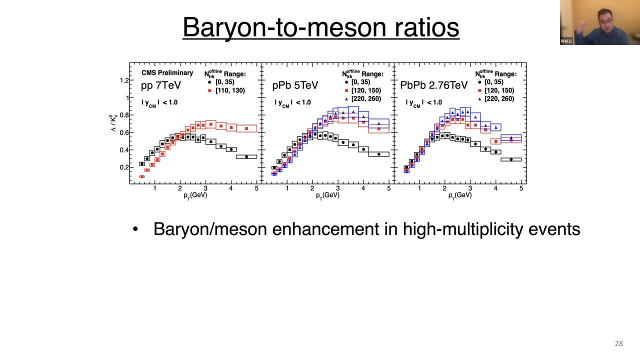 in PP, PLAD and LADLAD and in different ranges of multiplicity- see different distribution here- And so that this give us a very comprehensive information about the particle production dynamics in this system of different size. And so one thing we measure is the background to medium ratio. 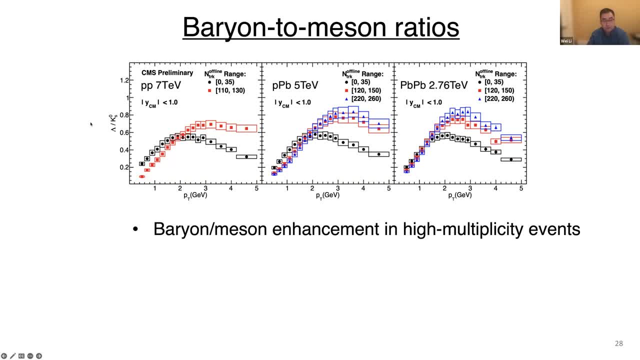 and what you see here is a lambda over k-zero shot ratio in PP, PLAD and LADLAD And as a function of PT, where we can compare the ratio in the low multiplicity, in the black points, versus the ratio in the high multiplicity. 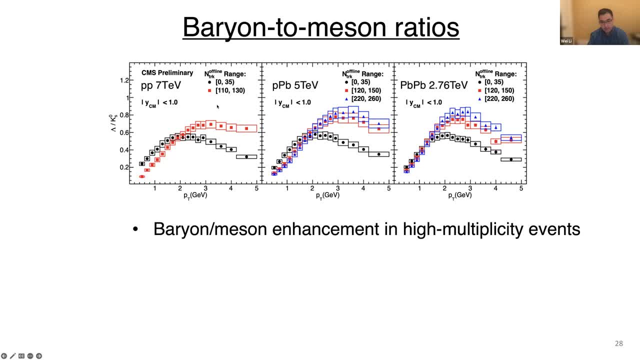 And you can clearly see well in the high multiplicity we see the enhancement of the hadron to medium. That is similar across all three systems. This is something we first see in LADLAD collisions, but we always see the same effect in small system. 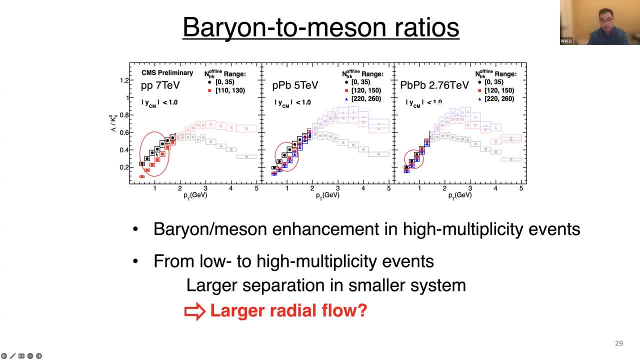 And from low to high multiplicity events. you see this, the shift, the separation and low momentum is actually bigger in smaller system And this could indicate that we are seeing a larger reduced flow in smaller systems because you know you see a big shift in the separation. 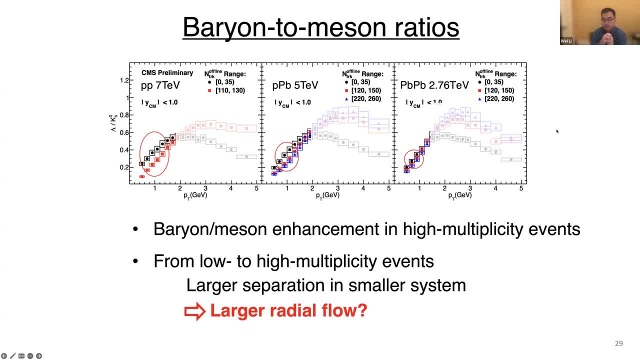 And then the smaller system has smaller system and this could indicate that we are seeing a larger, reduced flow in smaller systems because, you know, because the small system is the size is smaller, it's much denser, therefore it's more explosive. 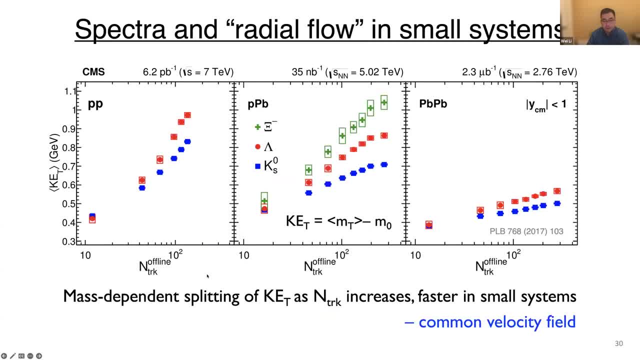 And we can actually see similar effect by looking at the average kinetic energy of the particle. So this is also known as MT minus M zero, as a function of the event multiplicity, And we can see that at low multiplicity they are the same. this is known as the MT scaling. 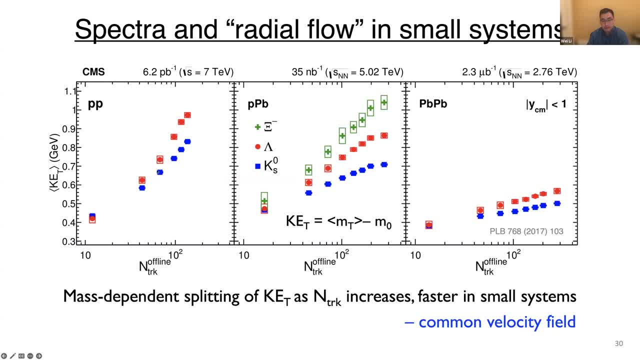 At low multiplicity but as an increased multiplicity the effects from the medium start to show up and the radio flows start to generate, which you'll see: the mass dependence splitting of every kinetic energy as the multiplicity increase, And this faster in small system. 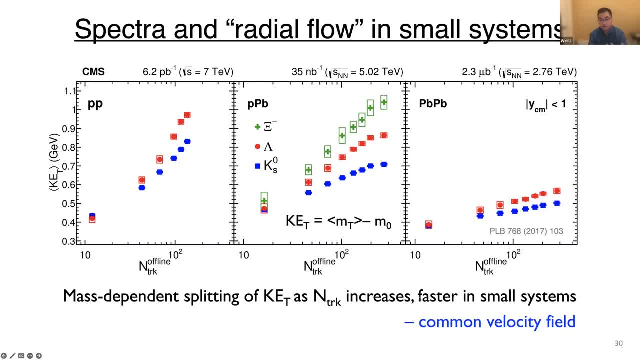 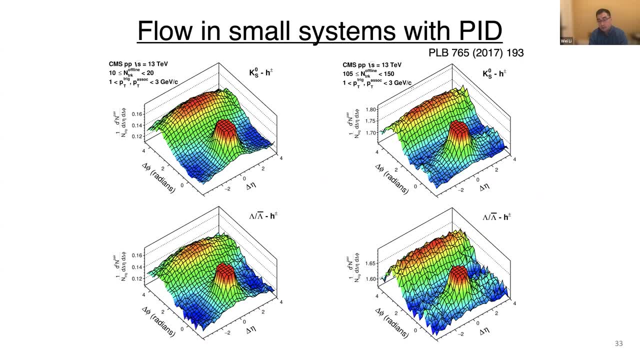 And this indicate that you cannot develop some kind of common velocity field in these conditions. Maybe I'll skip this one and I will move from the spectrum environment, And next we can also look at the two particle correlations with identified particles. Now, this time here. 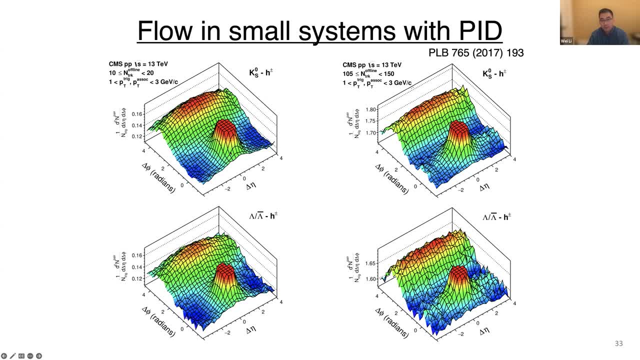 instead of correlating two inclusive hadrons, we look at identified hadron correlation with T-Shroud with the charge hadron, lambda with T-Shroud hadron- Oh sorry, lambda with hadron. So these two are for the low multiplicity events. 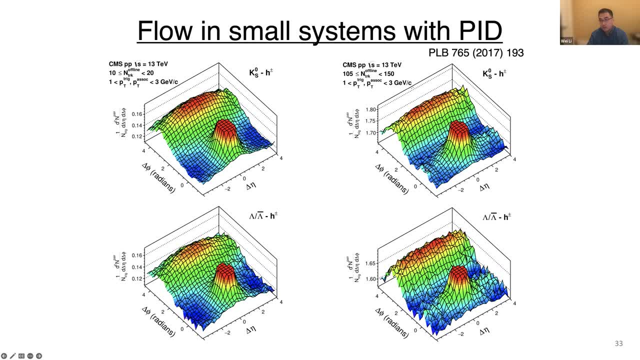 as on the right is for high multiplicity events where you can see that. you can clearly see that long range, near-sight ridge-like structure. This is in the. it is in proton-proton correlations. It's very similar to what we see. 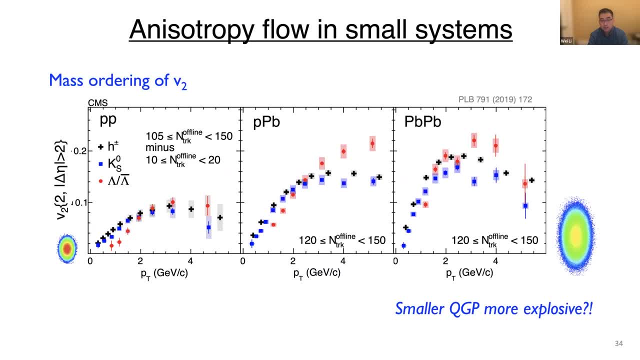 in the inclusive charge hadron correlations. So we measured, identified particle V2 from the small to large systems using the K-Shroud and lambda as a function of PT. You see, this is in the high-multiplicity PP correlations, P-Lag correlations and something like that. 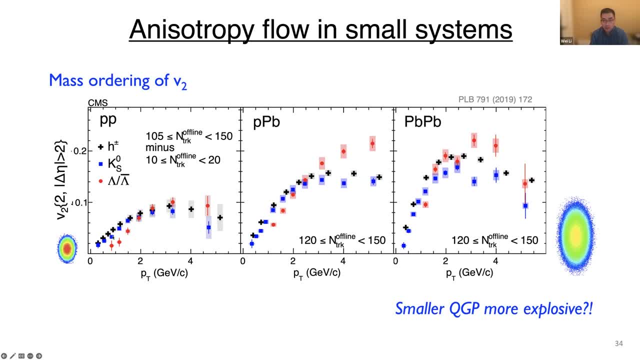 where you can see this famous mass ordering of V2, from the lightest particle to the heavier and heaviest, lambda, which indicates the kind of the radio flow effect And the separation is again, it's bigger for a small system than the larger system. 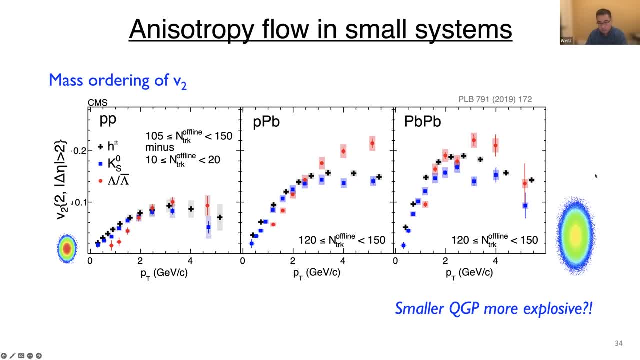 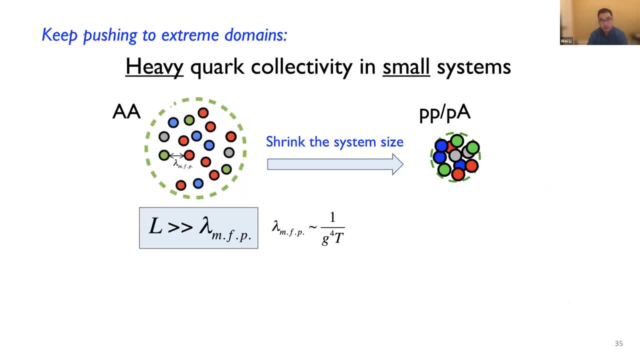 indicates that in PP you create a small 2GP that's more explosive. So, moving from the lighter particles, we also measured, studied heavy particle activity in small system, because our goal is that. so in large system, from the large to small system. 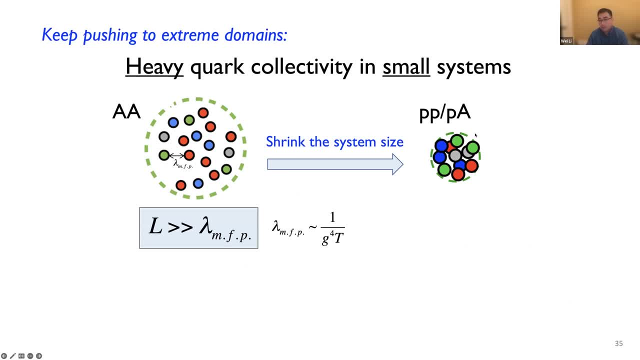 we shrink the system size right. We try to push the applicability of hydrodynamics to the limit, you know when the system size becomes potentially comparable to the mean free path of the system. Now, on top of that, to further increase the mean free path of the system. 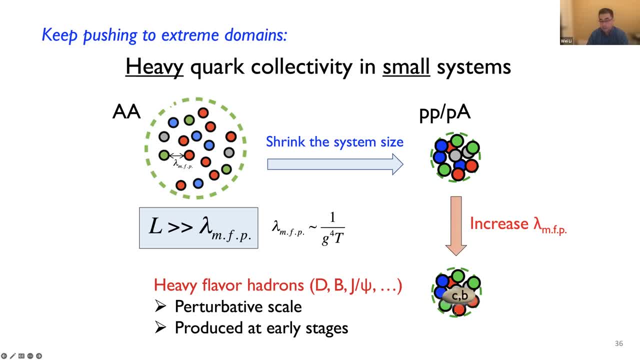 where you can replace the light flavor particle the heavy flavor. so it's like you put a stone in your liquid to see how it responds whether it flows or not. this heavy, very, very high-pitched object- And the nice thing about heavy flavor particles- 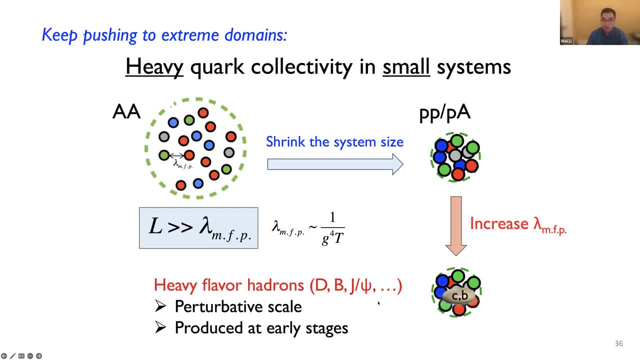 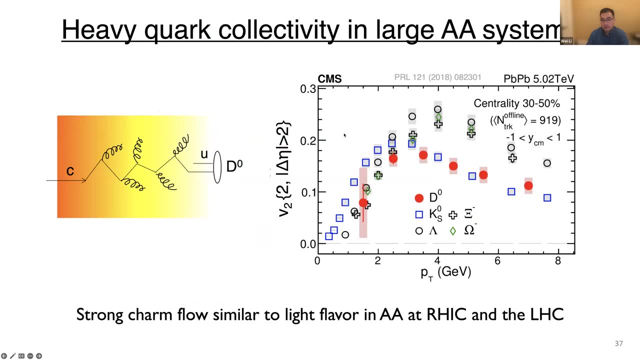 is that they are created at a perturbative scale, so you can do some perturbative calculation, and they also produce at a very early stage, So you can. it can help you to probe the entire dynamic history of the situations. Okay, so this is the measurement of the D0 of V2. 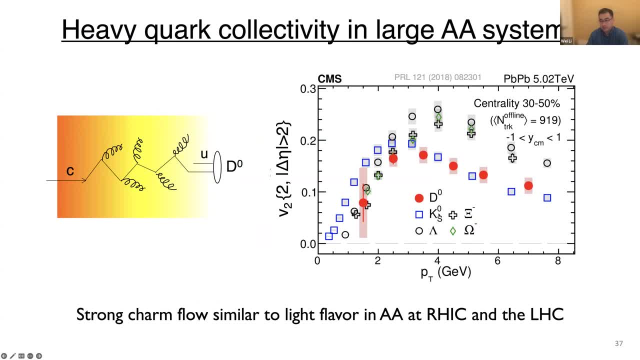 in lilac collisions and compare them to the, the, to the K-shard, lambda cascade and omega, You see that it's a collection of different particle species where we observe very strong time flow in these large systems. So very actually similar to light flavor. K0-shard. 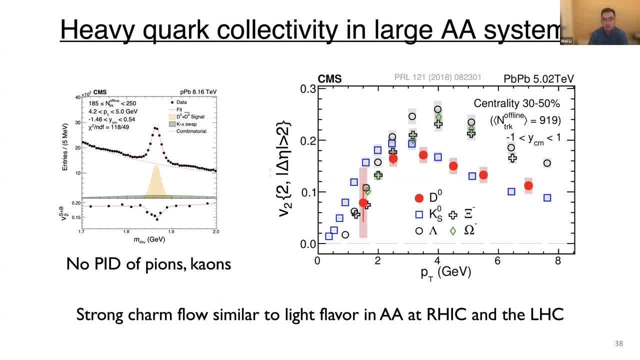 in AA conditions. And then here we actually to reconstruct D0,. we don't have any PID for charged pion K0s. It's really based on the high precision, the silicon detector. we can find a second vortex that can suppress that one. 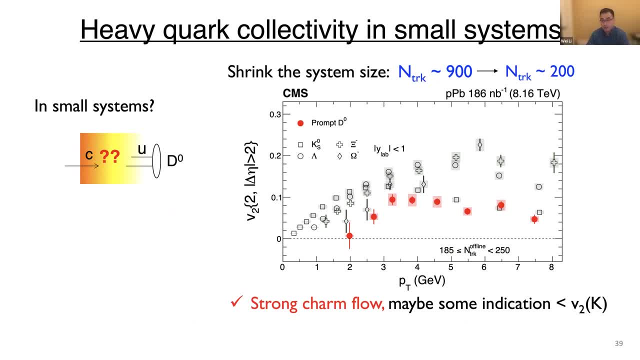 This is for a small system, This is for p-light collisions. We, again, we measure the V2 of all these parts, the D0 and K-shard, lambda, cascade and omega, And we also measure the V2 of the beauty hadrons. 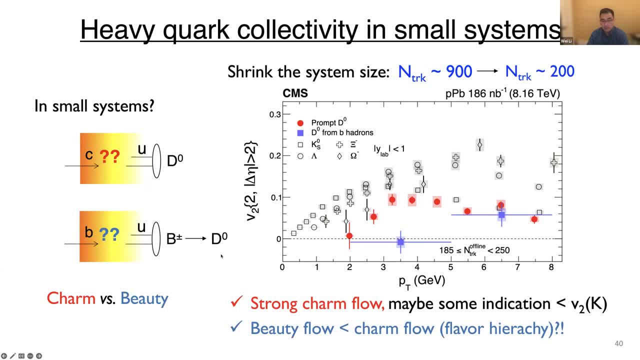 through the beauty. the B decay to D0, where you can see that we observe a very strong charm clock flow. So the prong D0s. in these red points There's some indication that it's smaller than the Ks, but the precision is still somewhat limited. 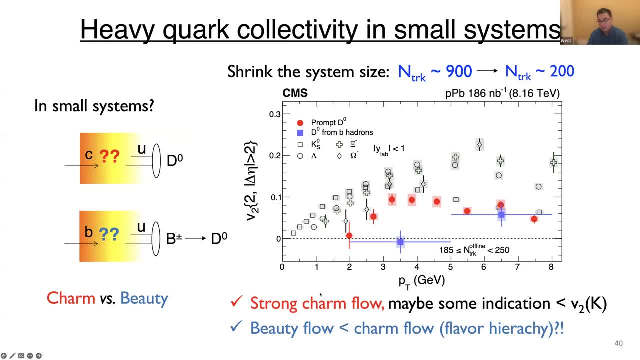 And for the beauty flow it is quite obvious that it's much weaker than the charm flow And we do clearly see a flavor hierarchy or a mass hierarchy that the heavier particles is flows much harder in the QGP medium And there is some calculations and escape that. 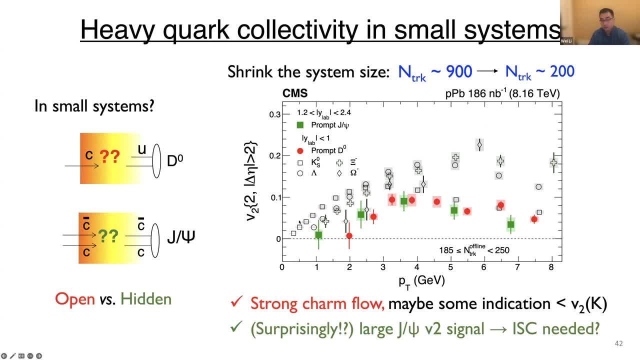 And also want to show you. we also measure the V2, the flow of GF-psi in p-light collisions And, quite surprisingly, the GF-psi V2 is as large as D0 V2.. And what can mean is that this can only happen. 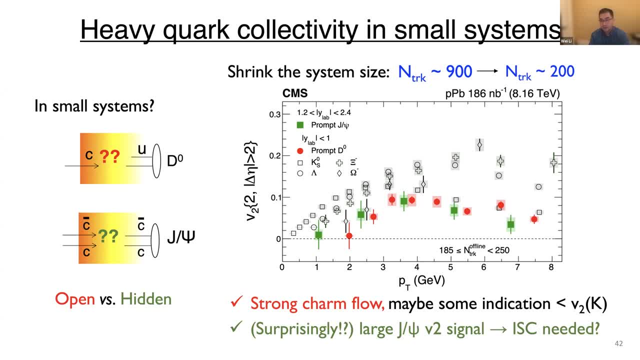 if the charm and the light-flavored particles have similar flow, right? Because D0 has one, has a light-flavored part. So for GF-psi, excuse me, So for GF-psi, we reconstruct through the dimuons. 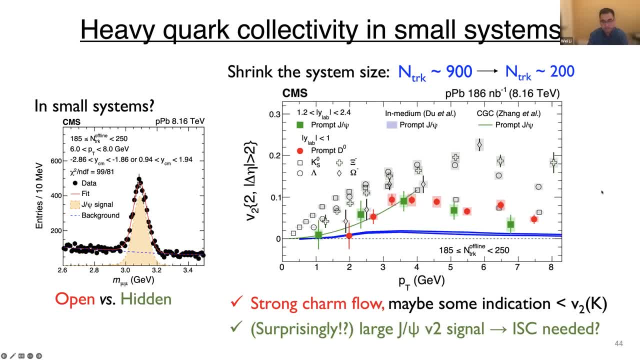 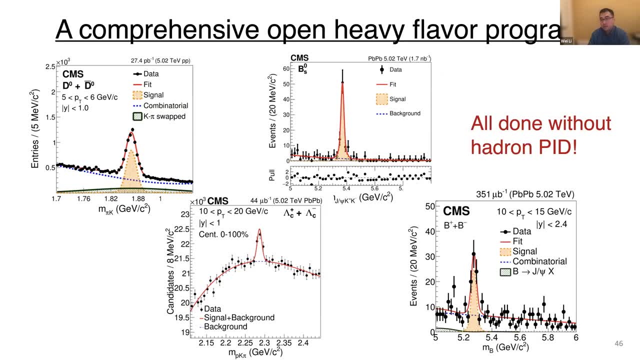 We can have a very clear and nice peak of GF-psi. So so CMS has. despite that we don't have excellent hierarchy ID, we still manage to have a comprehensive open heavy flavor program, as shown in the result of D0.. 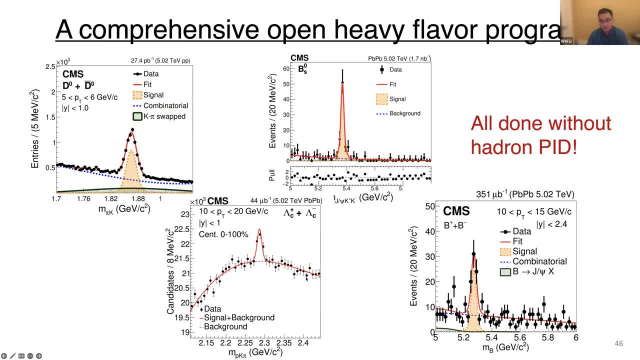 We also reconstruct the Mdc. It's a result of the idea, of course, in the background, this is large. We also reconstruct the B meson, B sub, S, B charge, B hydrons. We using the dimuons. 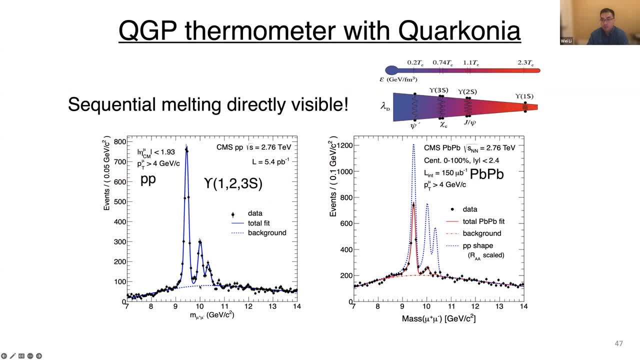 we can nicely marry the upsilon 1S, 3S and 2S in PP collisions and compare that to lilac collisions where you can clearly see the suppression of these quarkonian states. that is stronger, much stronger for more excited states. 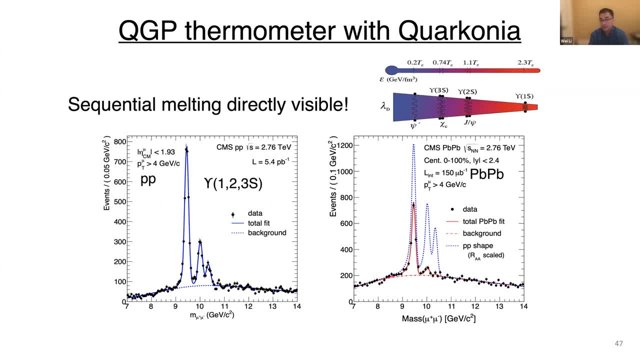 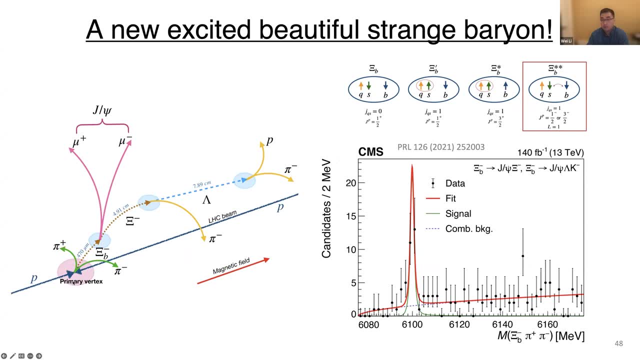 which is expected because of different binding energy of these quarkonian states. So most recently- this is an important current collision- The CMS also observed the so-called excited beauty, beautiful strange hydron, which made of a beauty quark, strange quark. 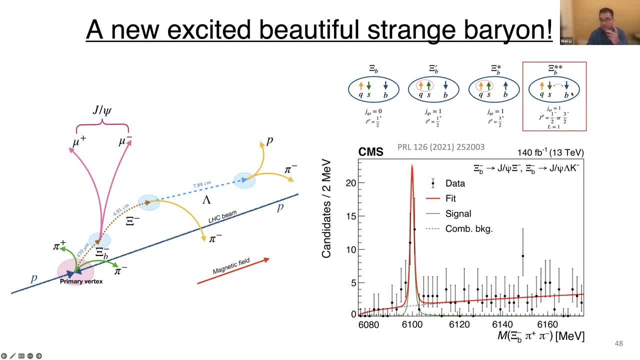 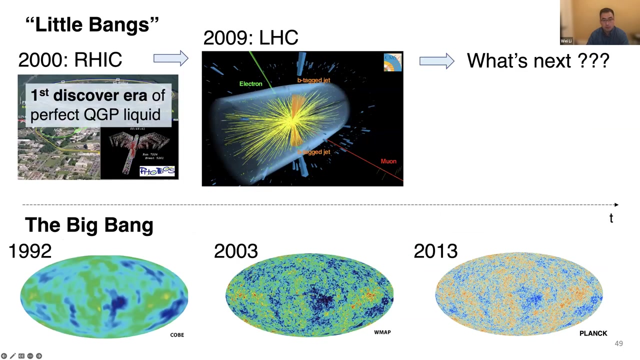 and light flavor. quark And D0 ran in some specific angular momentum stage And the decay chain is very complicated, but we were able to reconstruct it in fact and compare the decay chain and see the peak in PP collisions. Okay, so let me. 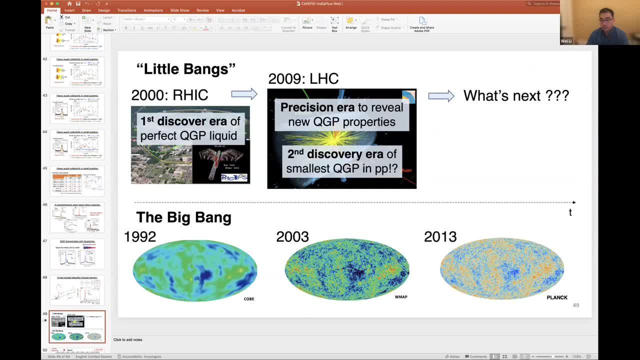 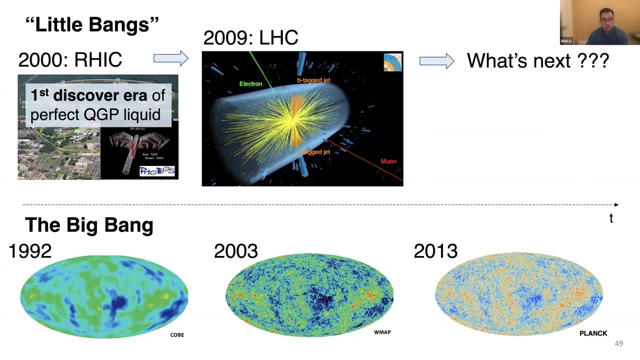 in the next 15 minutes I will quick summary up until this point that so. I used to work at the rig I work on experiment called Phobos. It's a very small experiment. It has a single layer of silicon detectors. 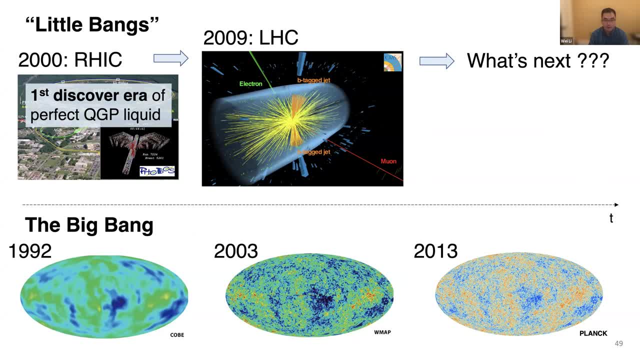 And so Phobos only run for like five years and it finished in 2005.. Many of you may not have heard of it, So rig is like the first discovery error of the perfect QGP liquid. We had a quick look at how it behaves. 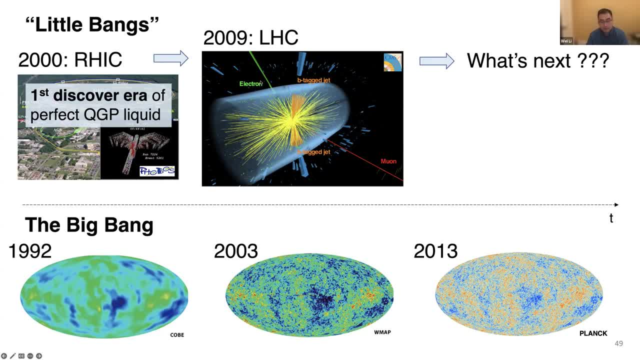 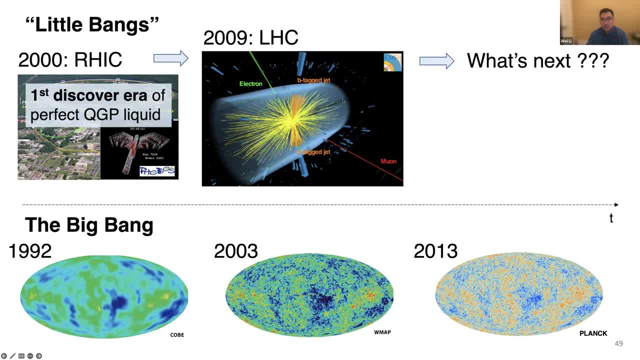 with their identification. So this is event actually having a top part, a pair of top part, produced in the LHC conditions where you can see the two B tech jets and the one electron from the W decay and one muon from the other W decay. 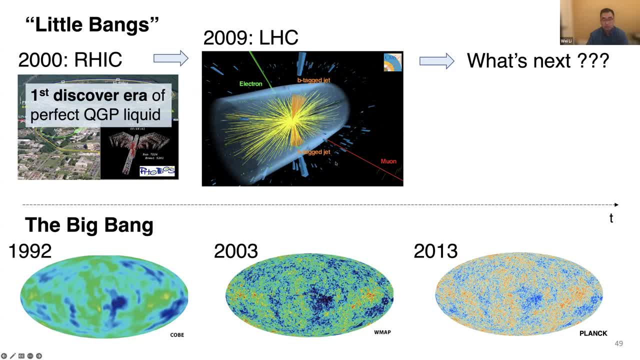 So we're from this. we can strike enormously more precise information that can reveal new properties of QGP. And we also had the second discovery error where we discovered the smallest QGP in these proton equations. So to make an analogy, you know. 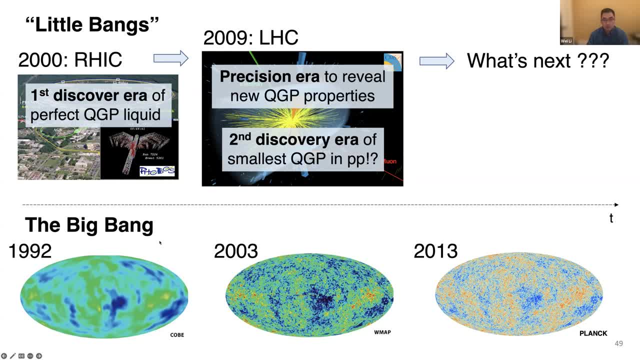 I think the cosmology is the good example where this improving of the electron is very, very important. So we can see that the electron is very, very small And that says, you know, if you just keep improving the precision, improving your equipment. 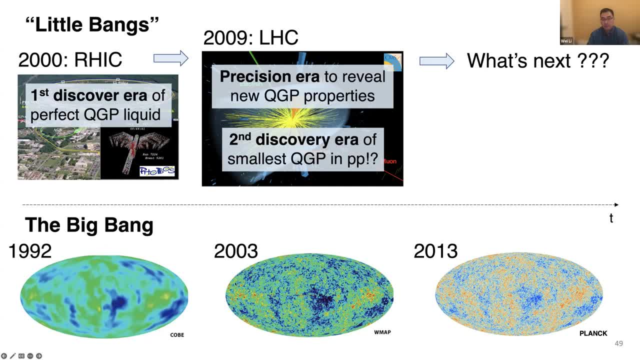 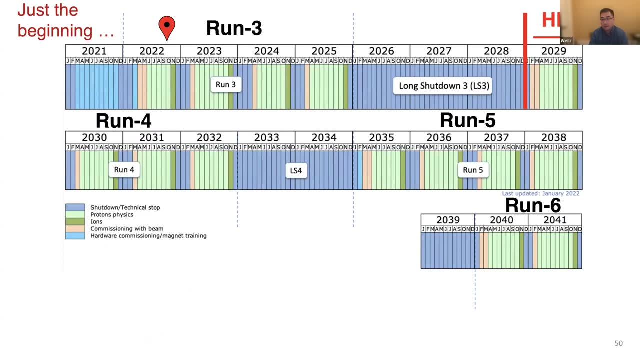 we increase the precision of your measurements, how that will make a qualitative difference from COVID, WMAG And so what? the question is now: what's next right? So what do we do in the future? So, in fact, if you look at entire LHC program, 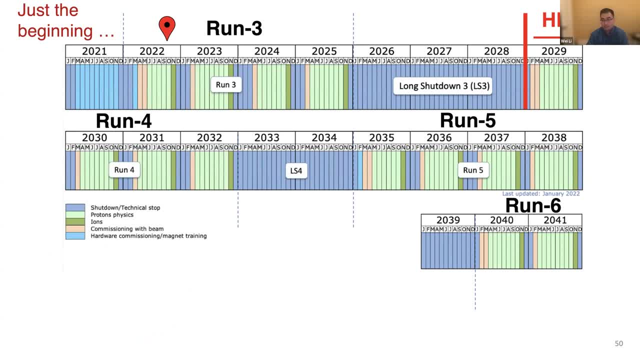 we are still just at the beginning of the whole program, whole program. So we are roughly one-third into the whole LHC program. The whole program planned until the end of 2041.. And in terms of the total amount of data that LHC has delivered, 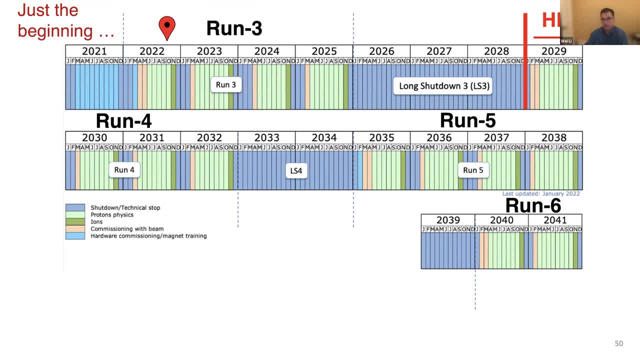 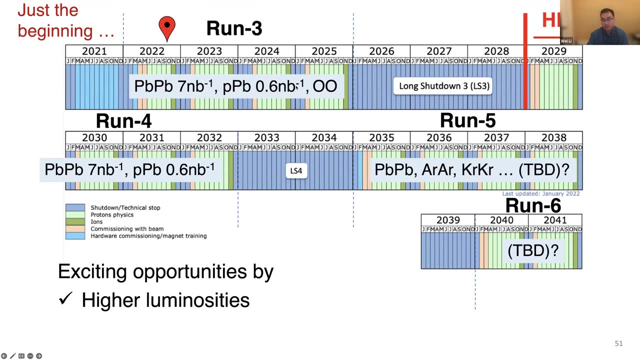 it has delivered only about five percent of the entire data center plan. So we are at the beginning of REN3.. So not only we are going to have a lot more data right? So in the Li-Li collisions we'll have more Pi-Li collisions We're going to have probably in 2024,. 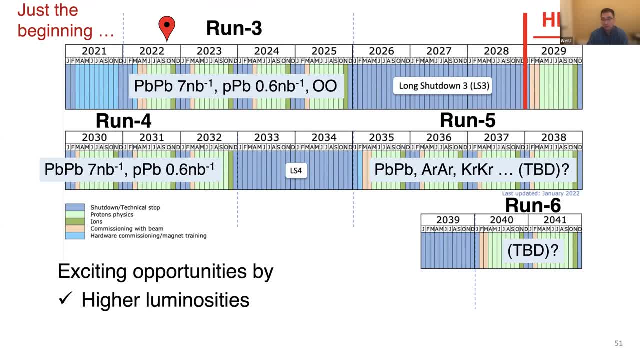 we'll have oxygen-oxygen collisions, the first oxygen collision at LHC And in the future in REN5, likely we'll try to do the lighter ions, argon, maybe the peptone, xenon, Those. the details of those programs have not been decided yet. But in addition to all these, 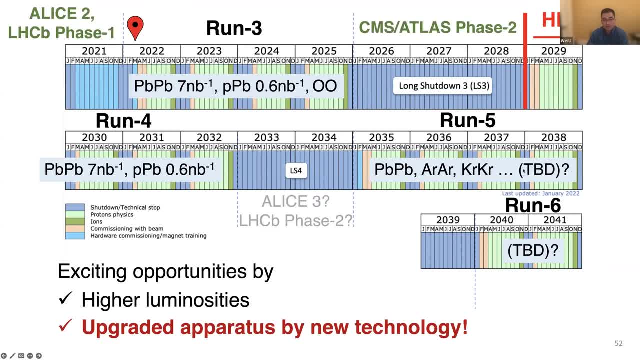 the more data that will be delivered. there will be also an exciting opportunity that will be provided by this upgrade For CMS and ATAS. there will be a phase two upgrade that, with new technologies, will provide us a new opportunity. And so, if you look at the QGP detection, 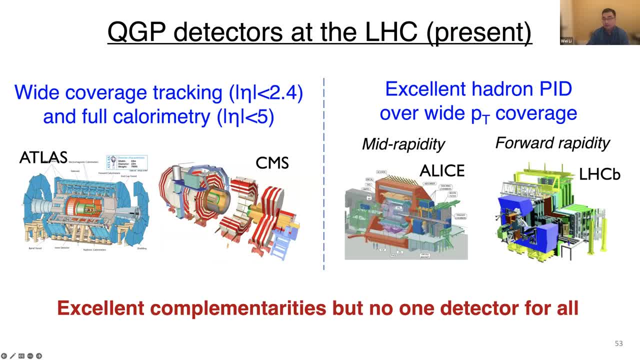 at LHC at the present right, So CMS and ATAS, they have wide coverage tracking full calorimetry right, So that they're a unique feature, whereas the ALIS and LHCB specialize with the excellent Hadron PID capability over wide PT coverage, either at the 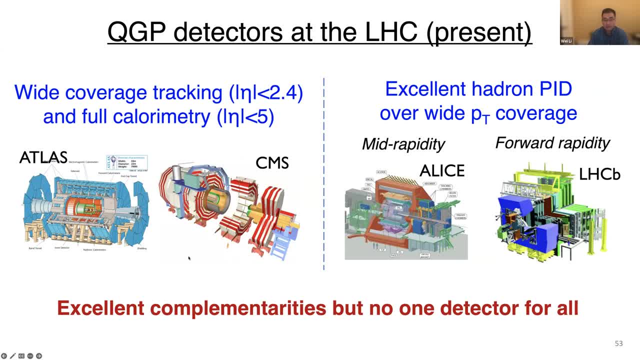 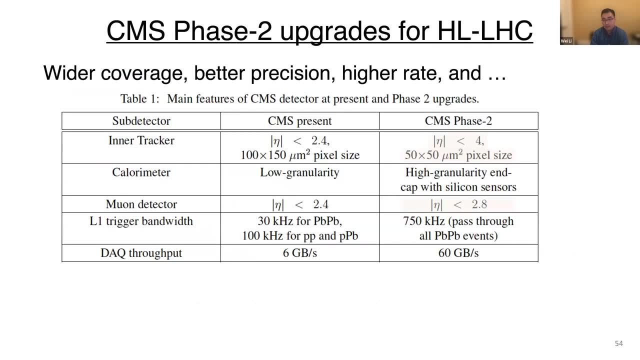 mid-rapidity or forward. There is excellent complementarity, but there's no one detector can do all the physics right. So it would be nice if you have one detector that can have all these capabilities, So that probability actually is emerging at CMS with the phase two upgrade. 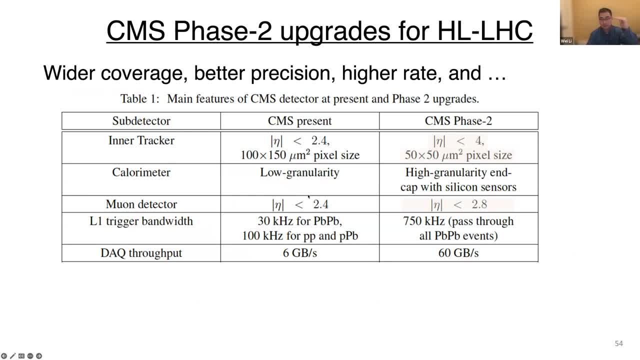 So what's going to happen at phase two upgrade? There will be as many changes to the detector, but we almost got a new, completely new detector in CMS, actually The inner tracker. the pixel size will be reduced to 50 by 50 microns. The calorimeter will have a. 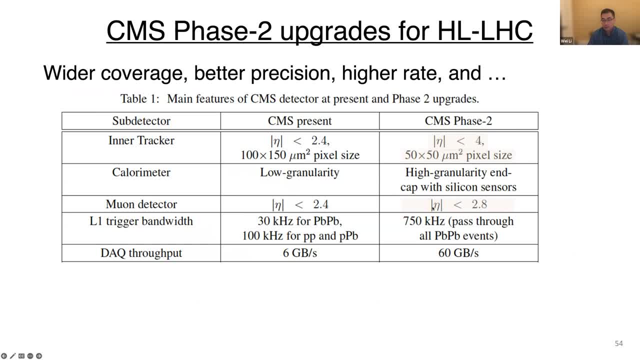 high granularity calorimeter Muon detector will have a larger coverage. The trigger, the data acquisition bandwidth will be significantly increased. so that you know, this is how the two-part correlation will look like by the HL-LHC in CMS and we are going to record all the LHC events with a large readout bandwidth. 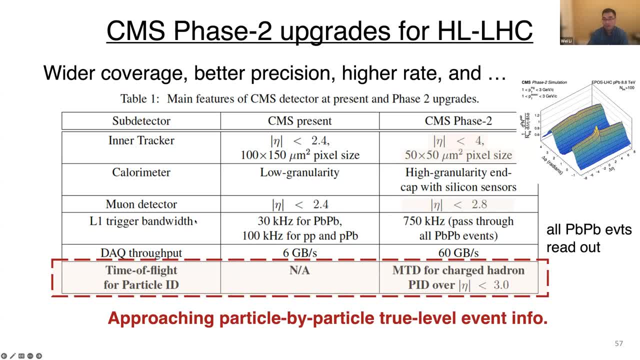 In addition, the most importantly, we are going to add a time-of-flight detector for Hadron PID- And that is new—that we don't have right now. we will have it soon, And so with that, we are really approaching the particle-by-particle true-level. 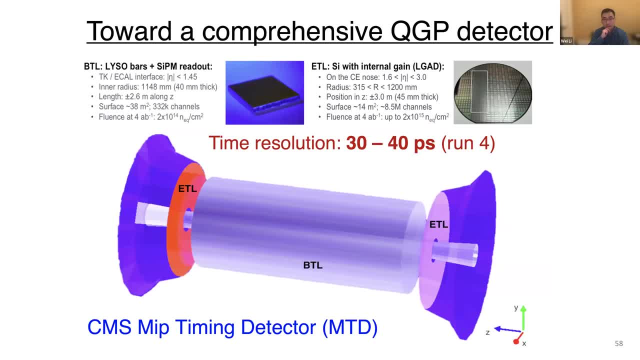 information event in the image. So I'm going to tell you about this new detector. This is a detector I actually worked on in constructing that. It's called MIB-timing detector MPD. It has two parts. The one part in the barrel is the BD. The first part inside is the BD, The second part is the LHC, And the second part is the LHC. Here the ticker is that number, so it shows the ticker, And so the ticker is the number of the ticker, And so the ticker has the number of ticker. 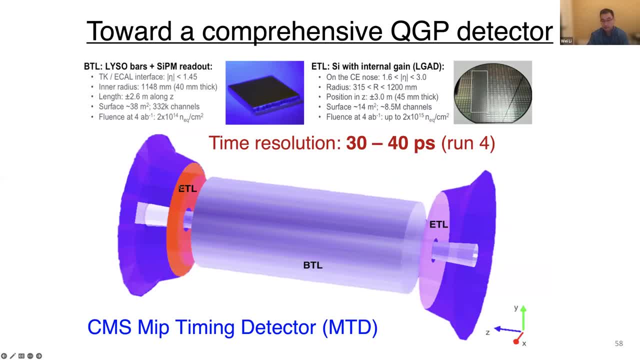 the number of the ticker, And the number of the ticker is the number of the ticker, And so the ticker has the number of the ticker. BTL, the barrel timing layer, and then there's the N-CAP disk for the N-CAP timing layer. 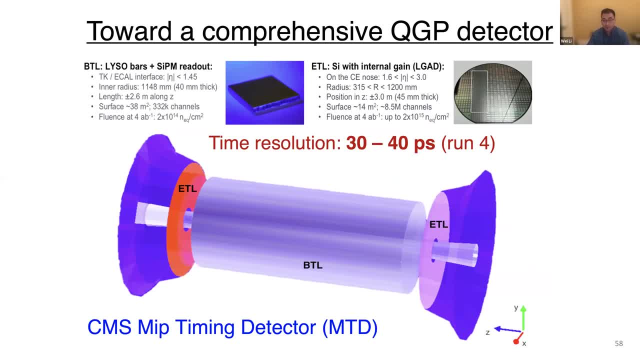 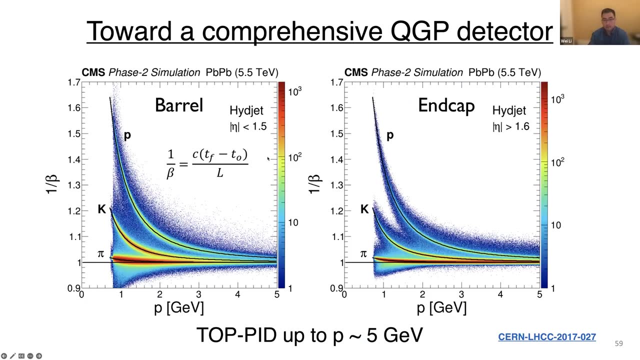 So the system is designed to provide a time resolution of 30 to 40 picoseconds per hit And the two parts they use actually different technologies. the barrel and N-CAP they use different technology. Before I tell you about the technology, let me first show you from a simulation the performance. 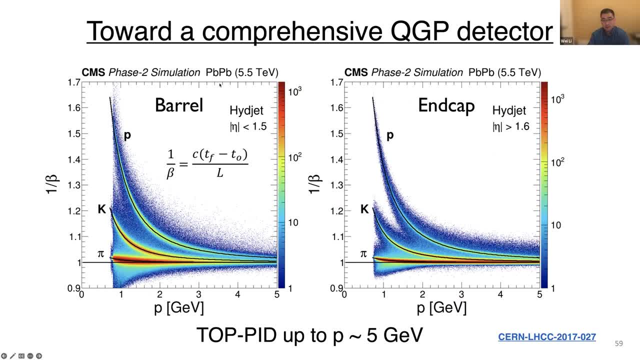 of top PID using this timing detector in the barrel and N-CAP region where you can see the lag-lag collisions, and now we can have very nice PID all the way to 5 or 6 GeV that we don't have at the moment in CMS. 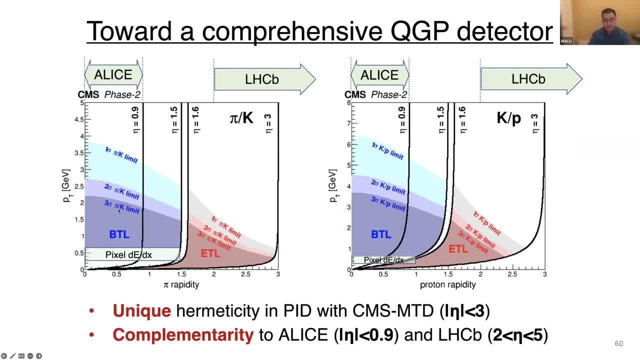 This plot shows you qualitatively the PID coverage in PT and ATAP for pi and ka separation and ka and proton separation, For 3-sigma separation, 2-sigma separation, 1-sigma separation, boundary in the barrel and N-CAP. 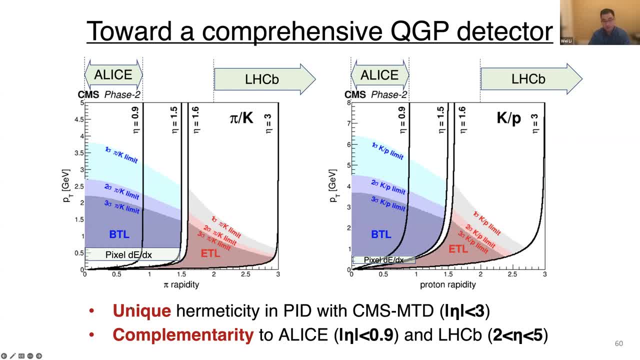 And you can see, the CMS is very unique in the sense that it can cover a very wide range in PID, the eta plus minus 3 units. It will be complementary to ALICE, which covers mid-rapidity, and LHCV, which covers forward. 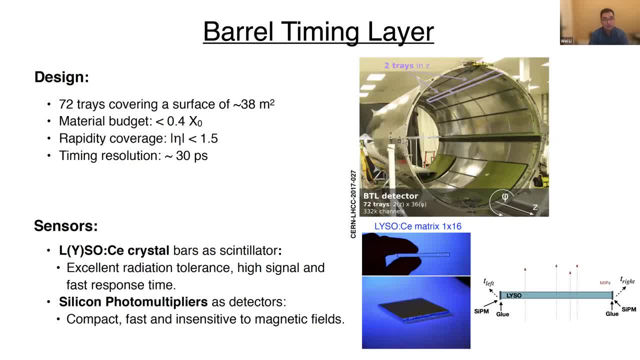 rapidity. So then, the barrel timing layer is made up of N-CAP and N-CAP. These are made of lysocrystal, these are crystal scintillators, And they have good radiation tolerance, And so they're read out by silicon photomultiplier, which is compact and fast and sensitive to. 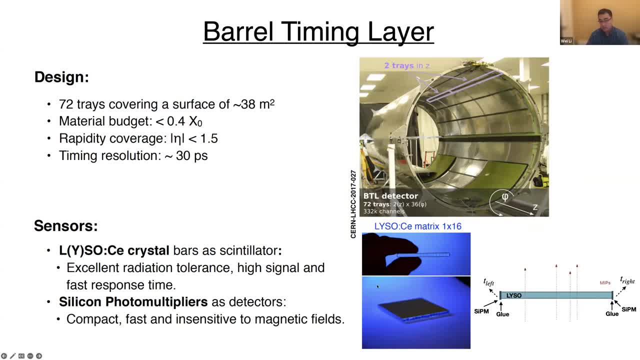 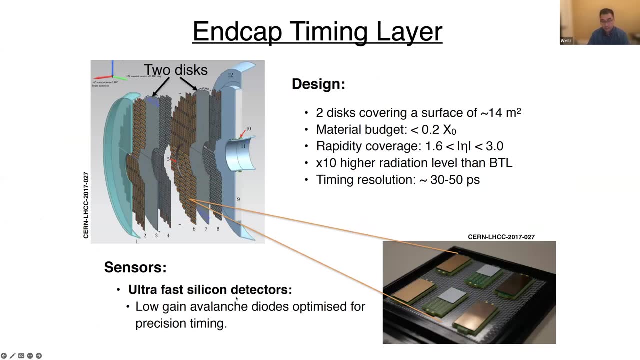 the magnetic field. You can see some pictures of these lysocrystal bars arranged in this array. So we have two readouts on both sides of the lysocrystal. Oh So N-CAP is a new technology. it's called ultra-fast silicon detectors or the Logan. 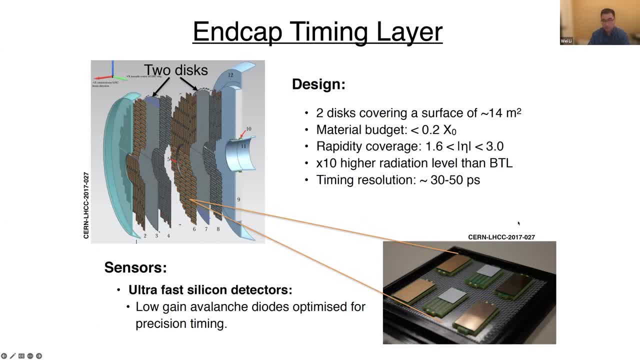 avalanche diode, optimize the precision timing And without going into all the details again. so the goal is to provide a single heat resolution on the out of 30 to 50 percent. So then we have two layers, or we have combined resolution of 30 to 40 percent. 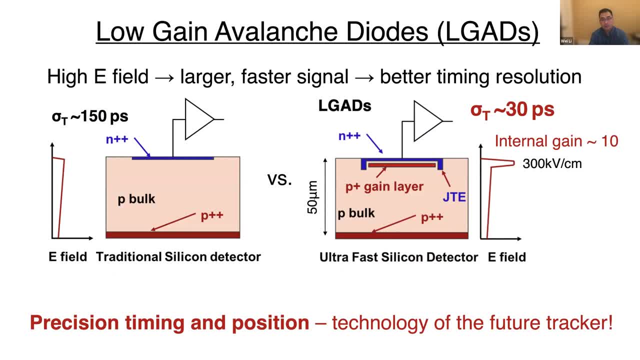 Okay, So this Logan avalanche diode is as I mentioned. it's a novel silicon technology comparing to the traditional silicon detector silicon sensor I showed earlier, which give you a time resolution on the out of 150 picoseconds. This is the L-GAS, the Logan avalanche diode. have these additional the peak gain implant? 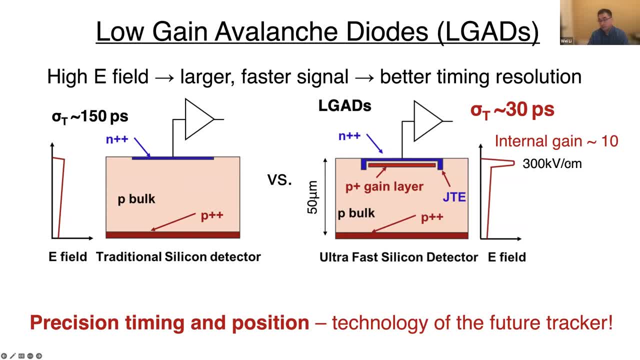 layers And the purpose is to create a much higher electric field in this local region. that will generate an internal gain, additional avalanche, to get an additional gain of an hour of 10 or 20.. So that makes your signal much faster and give you a better time resolution. 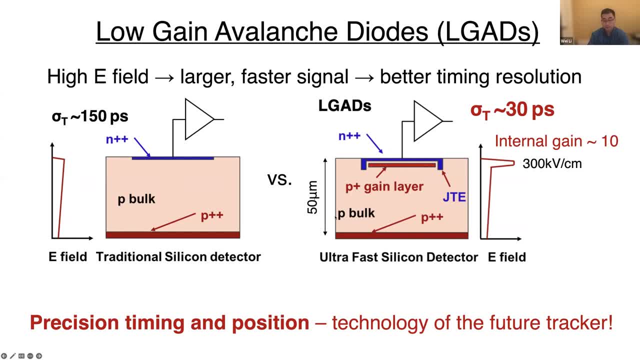 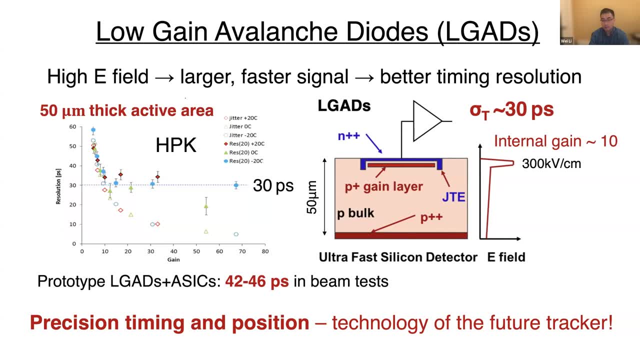 So with this technology, we'll be able to guide the precision timing and the precision resolution at the same time. So this is certainly the technology for the future tracker, and this is some of the BIM test results that demonstrate you that Okay. 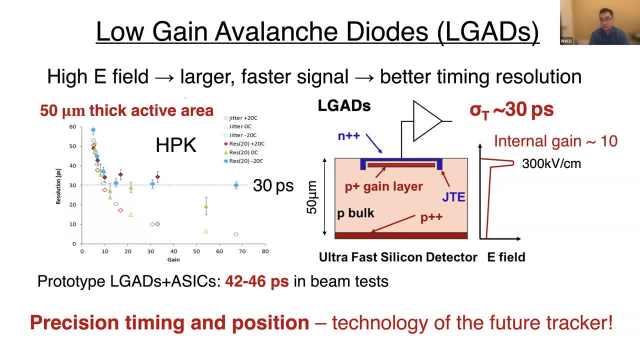 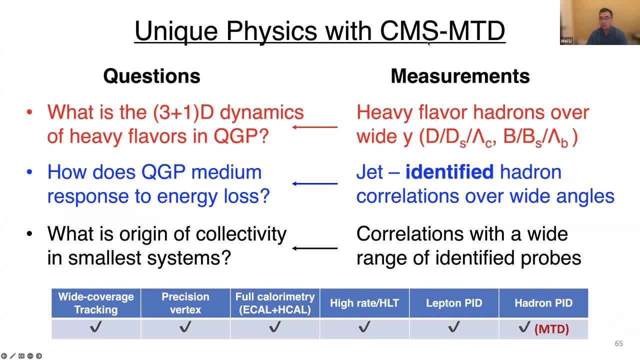 So with that, indeed, we can get this performance. So with that, I will think I'm running out of time. I will briefly show you some physics, what physics we can do with this new timing detector. And, in general speaking, so this MPD will basically provide the last measurement of the 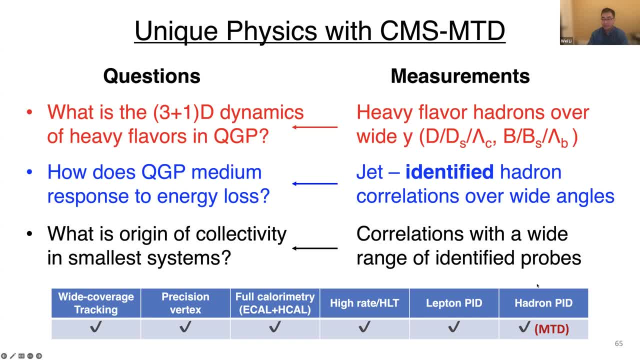 missing capability of CMS, which is the Hadron PID. With that we are, the CMS will become a detector that can almost do errors to the most complete, the detector for QGP studies that will be error-free. We can study the heavy-flavored hadrons over a wide repeated range. 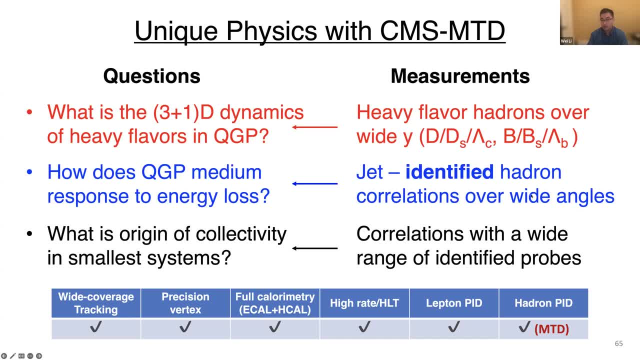 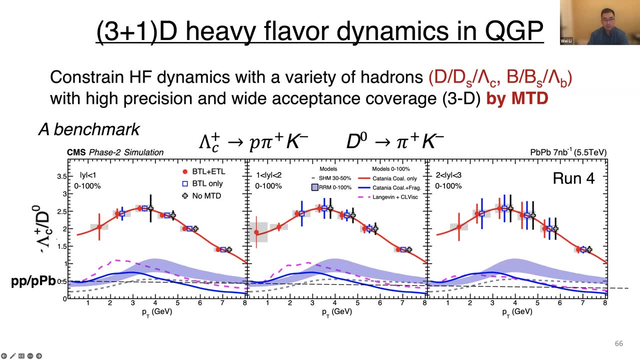 We can do jet-identified hadron correlations over wide angles And we can also study in more detail the small system collectivities with more identified probes. This is to show you the performance with the MTD, how well we can measure the Lambda-C. 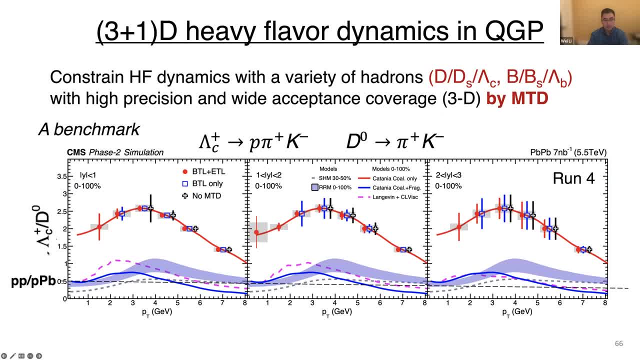 hadron, the Charm-Baron-to-Mason ratio as a function of PT. This is projected precision. You see the black points. this is the result, MTD, and the red point is the precision we can achieve with the PID. Okay, 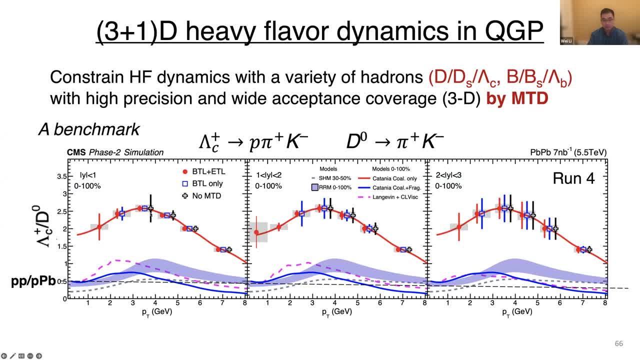 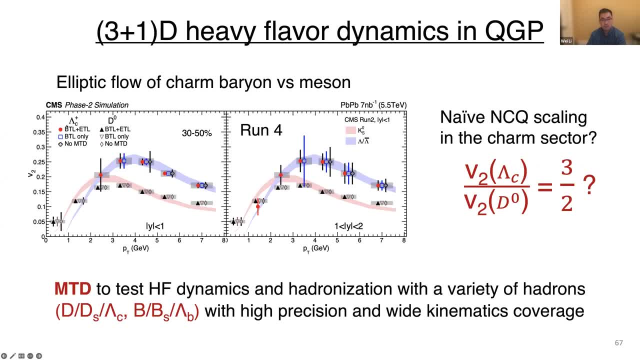 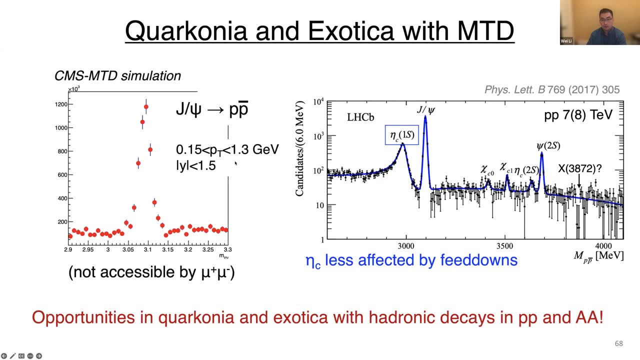 By the MTD, which we can significantly improve the precision range to a much wider kinematic region. Same thing for the V2 measurement of the D0 and Lambda-C, And we can even measure the hadronic decay of GF-Side through the proton-antiproton. 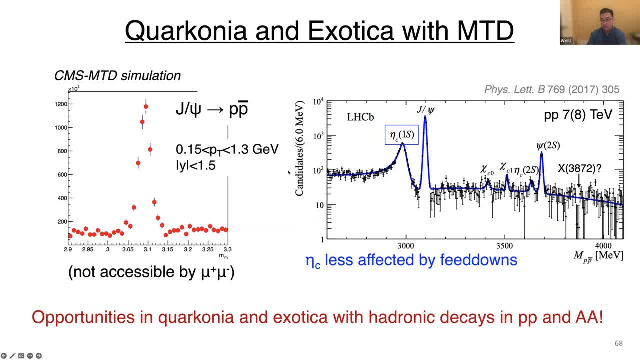 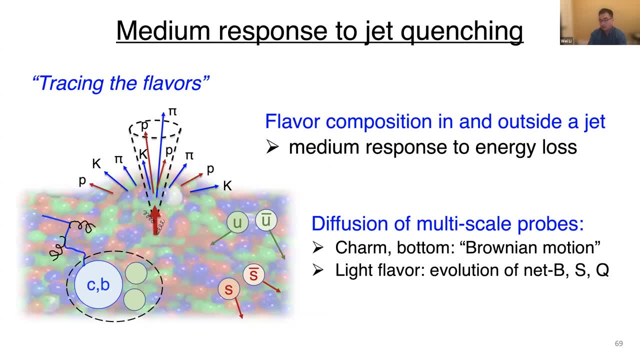 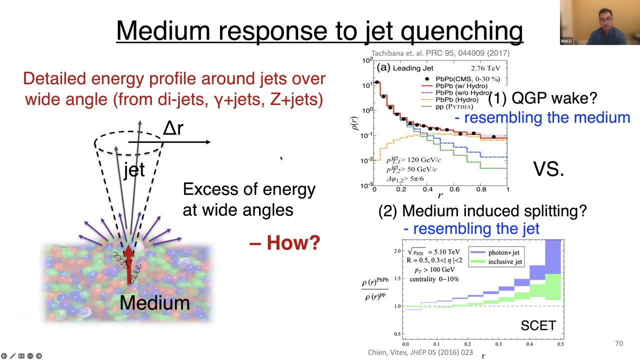 so that we will be able to access the GF-Side to a much lower PT. Okay, We can study the correlation of the jets. You can study the correlation of the jets with identified particle production around the jets, So that I will skip some of this, but generally speaking, this will help us to understand. 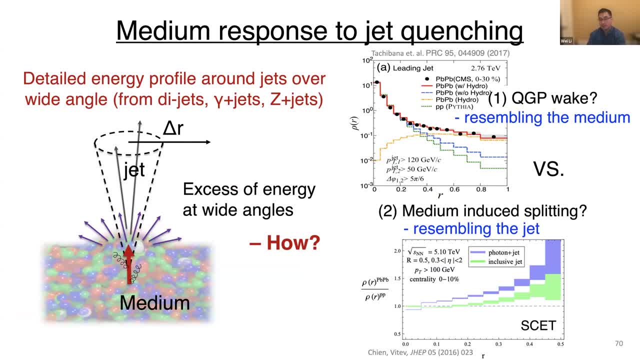 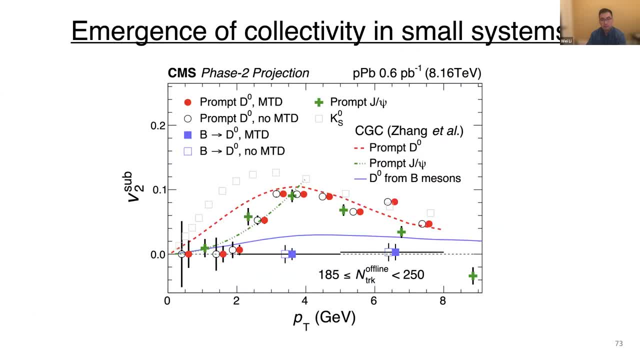 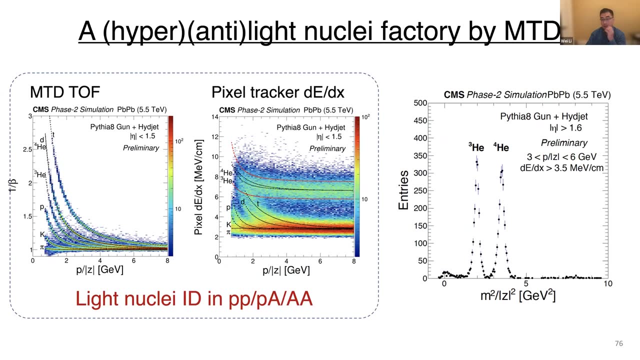 better how the proton will lose energy in the medium and how the medium will respond to the proton. Okay, Energy loss. Let me go a bit faster. I will mention that one last performance is the. with the MTD, the CMS will also be able. 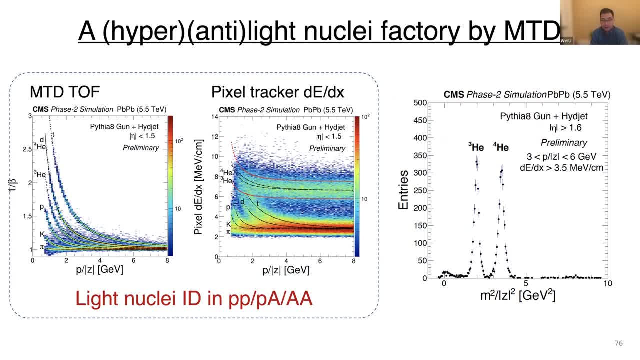 to measure the light nuclei like the, you know, the deutron helium-3,, triton helium-4.. Those are not possible to measure at the moment But with the time-of-flight, combining with the silicon tracker, with the EDX, we will. 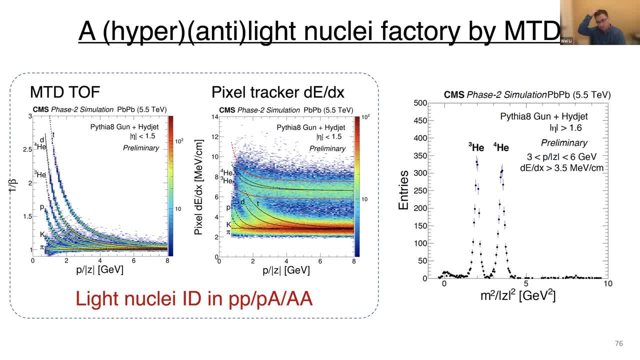 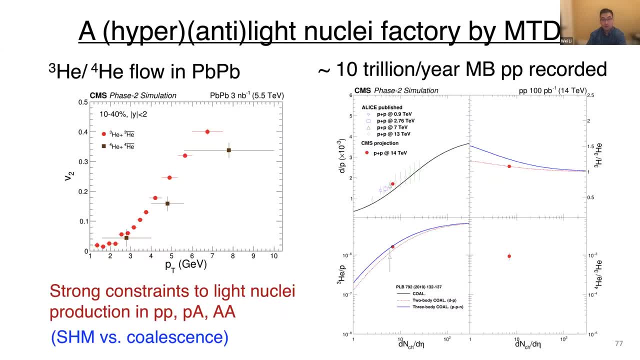 have excellent identification of this light flavor- sorry, the light nuclei- and turn the CMS into a light-nuclear factory. And we can measure the V2 of helium-3 and helium-4 as a function of PT And we can measure the light nuclei in PT collisions that can differentiate different. 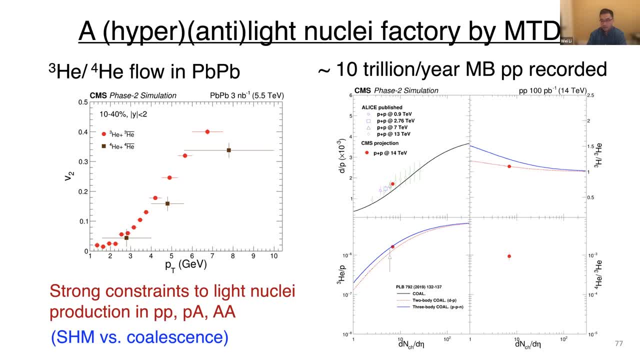 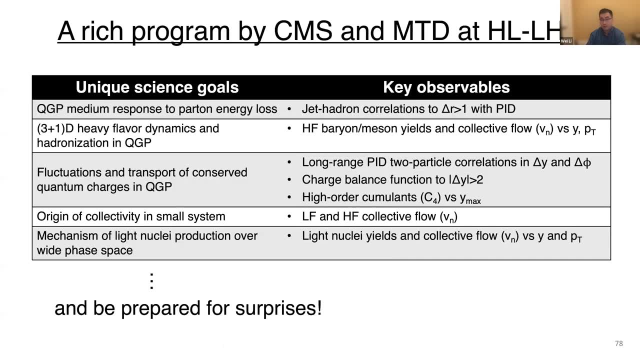 production mechanisms Like the two-poly coalescence, three-poly coalescence and so on, And there is a rich program by CMS and with the time-of-flight detector provided by MTD in the era of high luminosity LHC I mentioned. I didn't have time to talk about all of them. 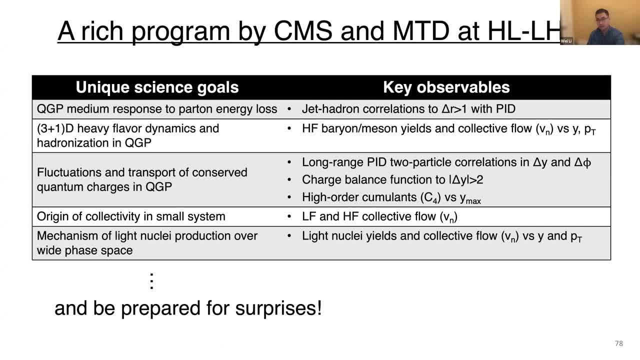 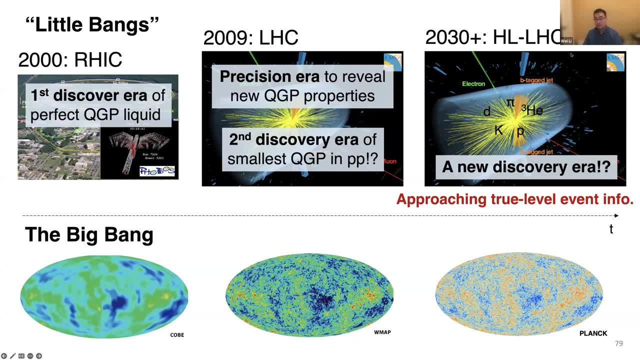 And there's a long list. You are welcome to look at the document that we published, And We are also. We are also prepared for surprises. So, in the end, let me conclude with this slide that you know we are looking forward to. 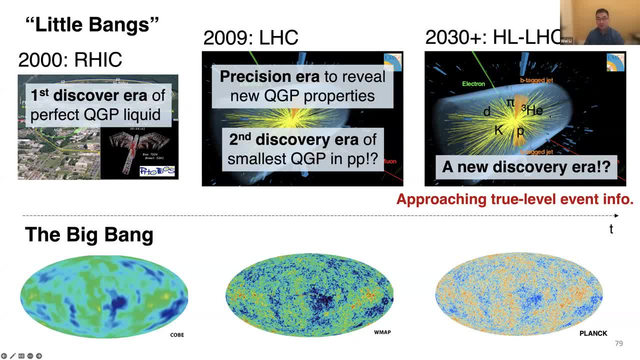 the high luminosity LHC era where, with the new time detector, we will be really reaching, as I mentioned, approaching the true-level event information where we identify the every single particle produced. You know what's their momentum, their identity. 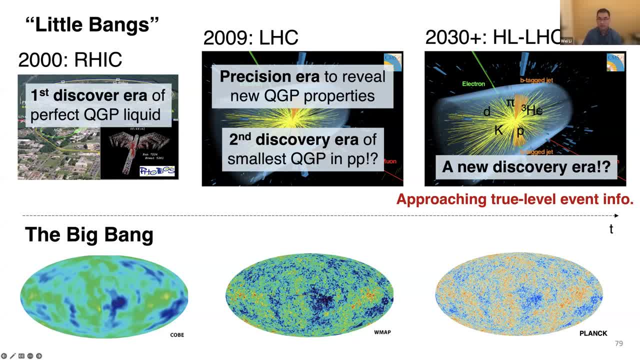 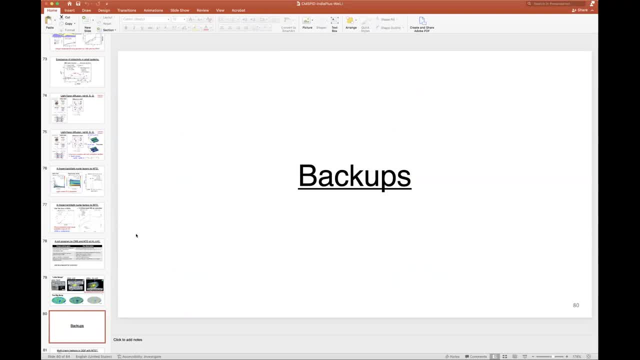 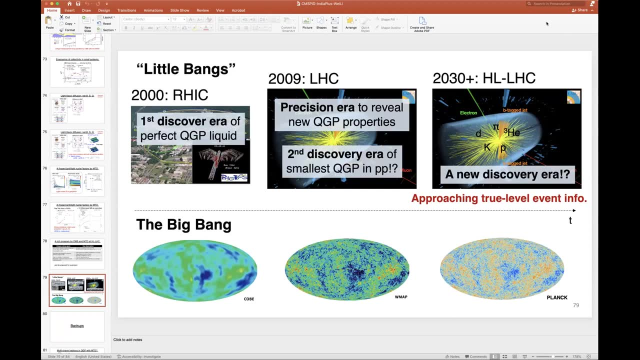 And we are looking forward to the new time detector. Thank you, Thank you so much. So there are a few questions in the chat box, So I will go through them. If you have further questions, add them to the chat box or raise your hand. 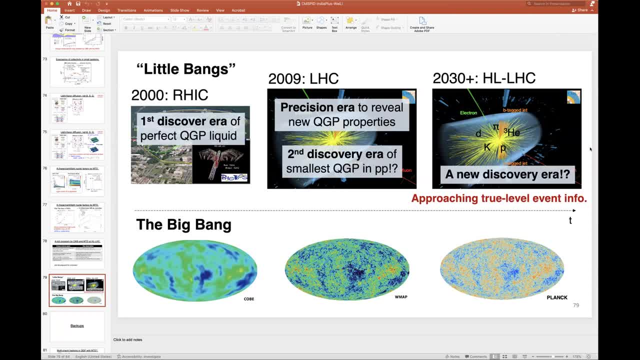 So Bartha asked a question: How do you optimize this energy frontier? 85% PP and the rest heavy iron. How do we optimize So it's determined. So basically, every year we run one month of heavy ions And then the rest five or six months of proton-proton collisions. yeah, is determined based on. 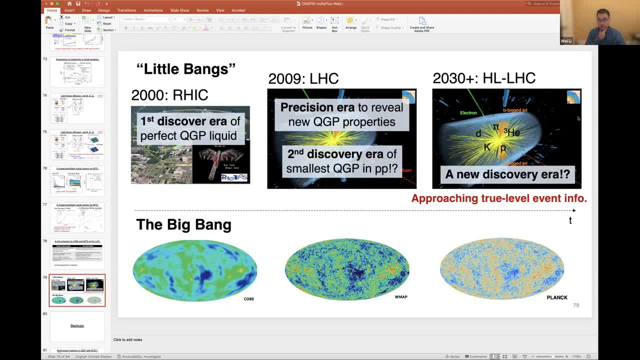 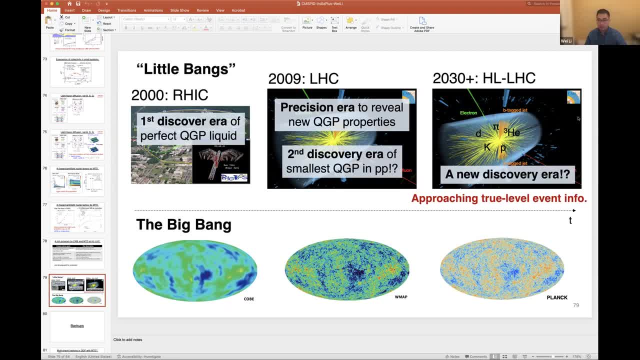 the portion of the heavy ion program, But of course the PP program is. The goal is to discover new particles, right To discover hits, And that will be always the priority, I think, for the next years, for the next years. 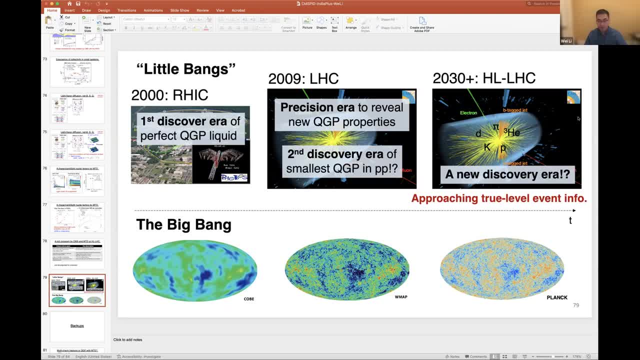 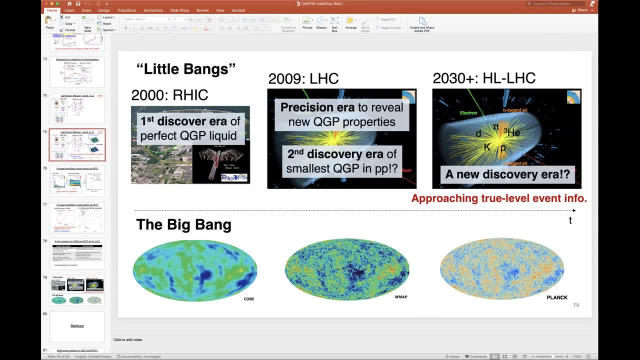 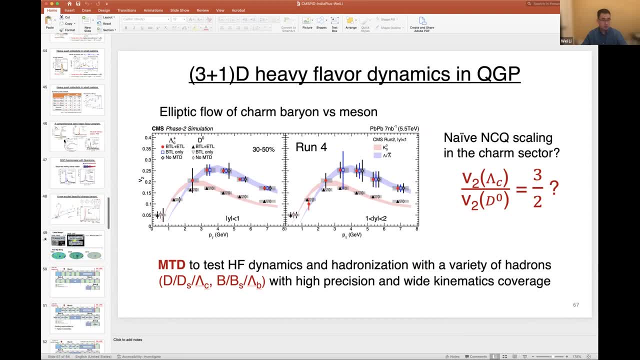 and Partha's question is: did you check the in-situ scaling in this high multiplicity events also? Yeah, that's a good question and I did not have it in the backup. No, I don't, but yeah, we have the plot in the paper. 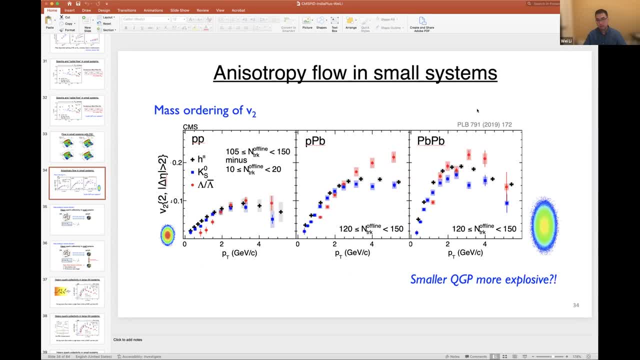 Yeah here, yeah, we had about in the paper where if you scale by the number of parts and you do see that the PLADD has shown very good in-situ scaling, It's even better than that. Proton-proton is not so clear because the intermediate PT region, the precision is still. 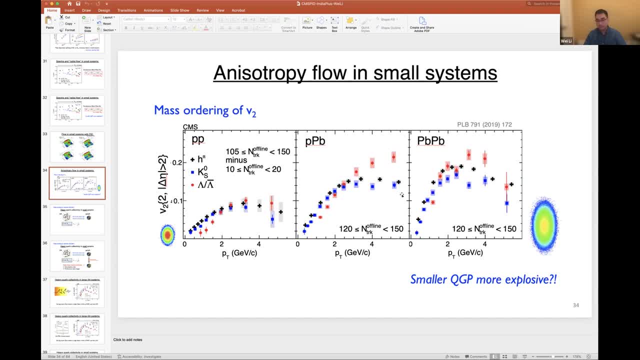 not so good. We still need to improve that and in PLADD we see very good in-situ scaling. Okay, There is also a question: what's the maximum reaction rate for PP and AA collisions? Yes, So the yeah, the bunch crossing rate for proton-proton is 40 megahertz. that's very high. 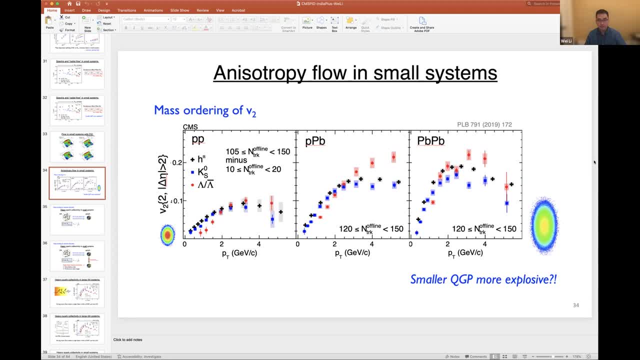 and for Li-Li collisions is at moment roughly 50 kilohertz and proton-Li collisions roughly three megahertz. Yeah, Okay, so one question going down. So I had one question. So in the JET reconstruction, is it done this way that you look at all the particles in the hydronic as well as the EM? 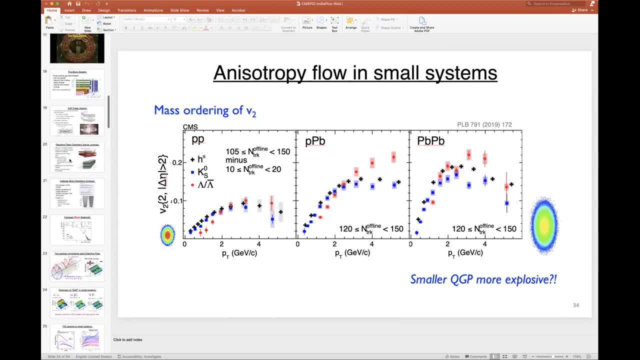 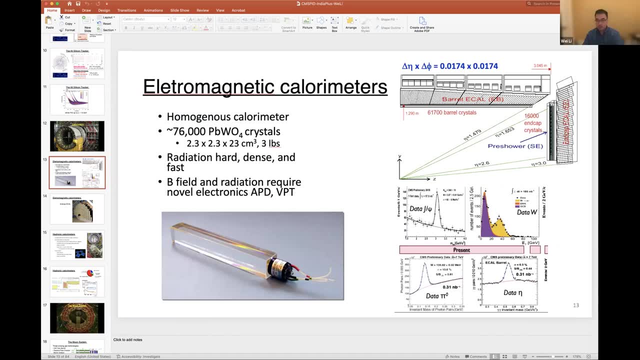 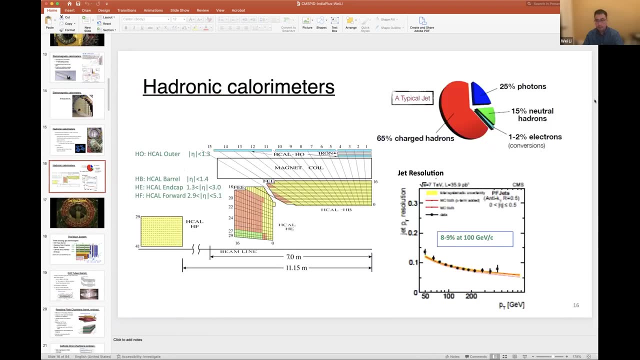 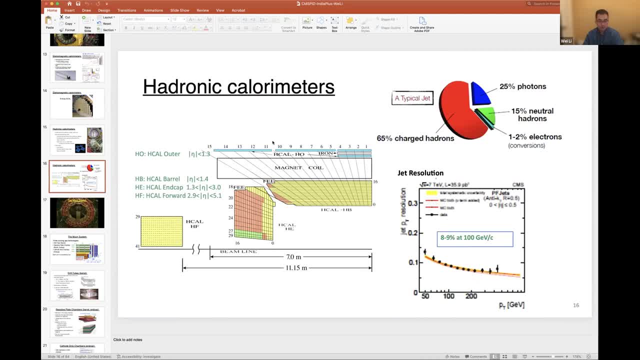 there are. these days we use so-called particle flow algorithm, which means that we first take the energy clusters in the hydronic calorimeter and the EM calorimeter. We try to link them to tracks, first Right And- Okay, And then they becomes a particle. 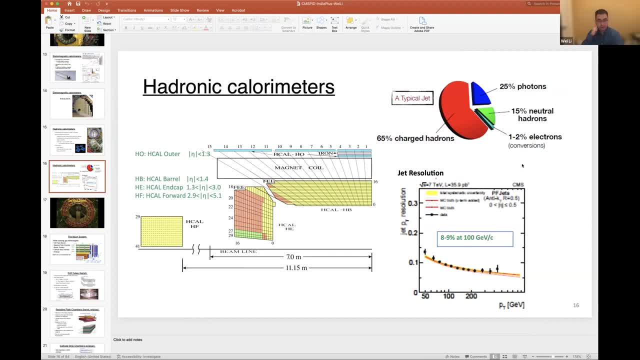 So we. so if you can connect to a track, then this is become a hybrid. So in the end we create a list of particle objects: There are hydrons, there are photons, there are electrons, there are neurons- And then we cluster this particle object. 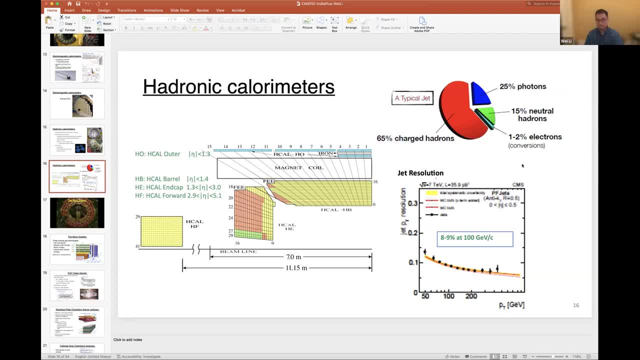 That's called particle flow algorithm. Yeah, Okay, Thanks, And let's see. Yeah, So Sandeep had a question: What could be the rapidity coverage for heavy flavors? Yeah, So, at the moment, you know, with the current CMA detector, 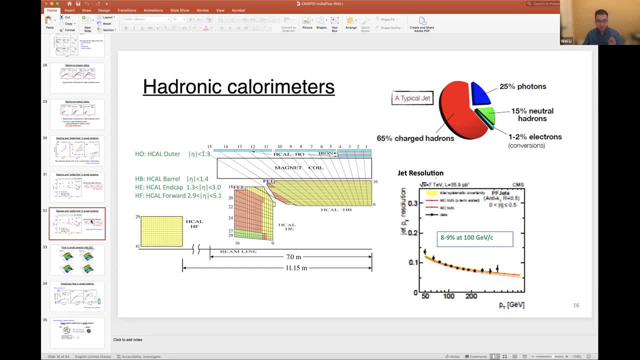 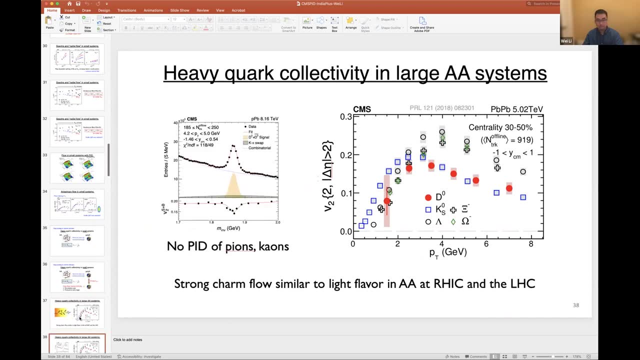 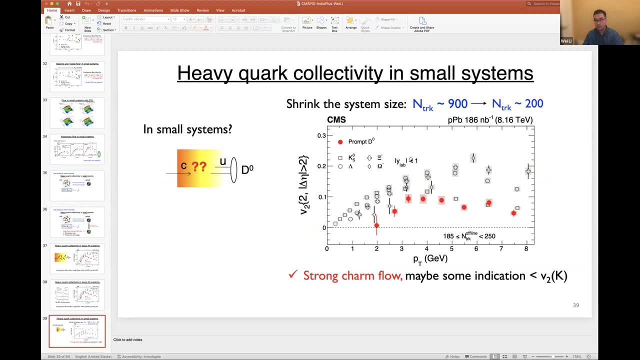 without hydron PID. without, with very little hydron PID, we are mostly mirror the middle rapidity, Heavy flavor, For example here the DMAs on V2 in Li-Li or in P-Li. this is measured at a rapidity less than one. 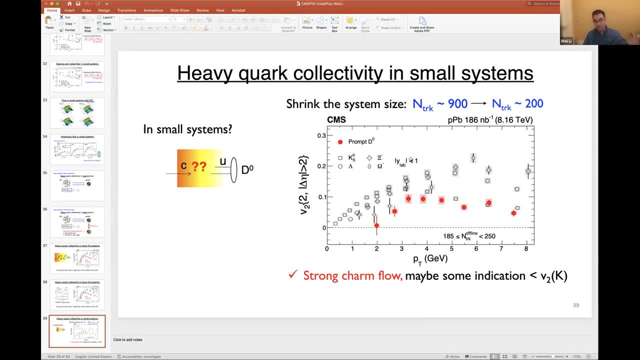 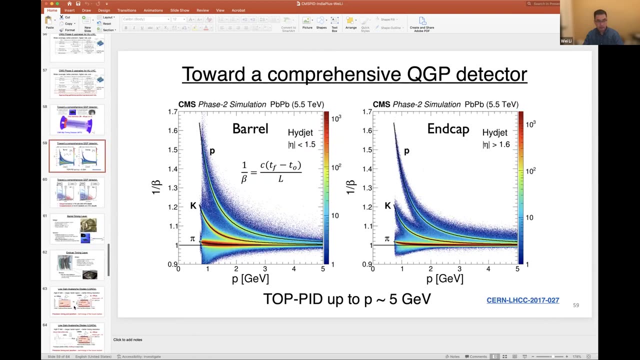 because the high rapidity will be difficult, The background quickly goes up and it will be a very hard to do without PID. However, with the addition of the MTD, this timing detector I mentioned, with the pi and k on proton ID, 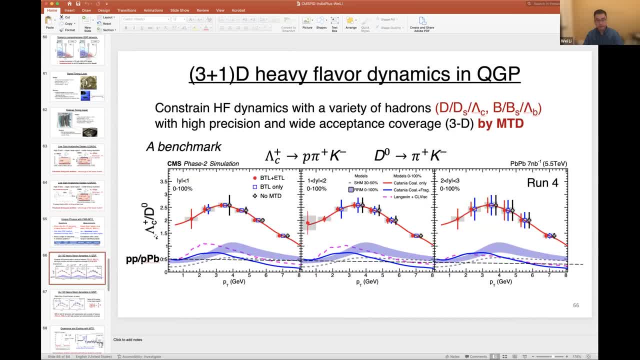 we will be able to measure very nicely the D0 and also the baron, the charm baron and the seed over wide rapidity range. See, this is wide, mid rapidity. wide from one to two units, even wide from two to three units. 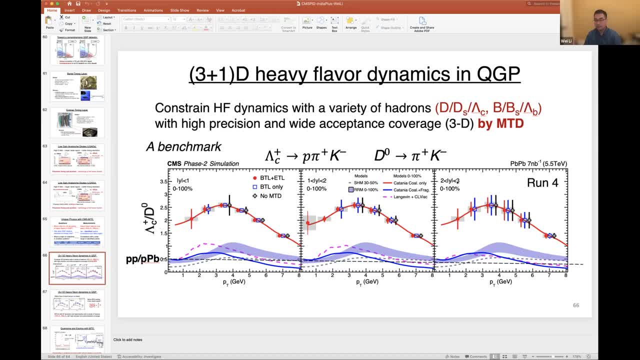 It's a very powerful detector that we'll have by the time of run four. Okay, Then Chitrasen had a question. So do you have any specific detector hardware or software upgrades in CMS to handle high luminosity in run three? 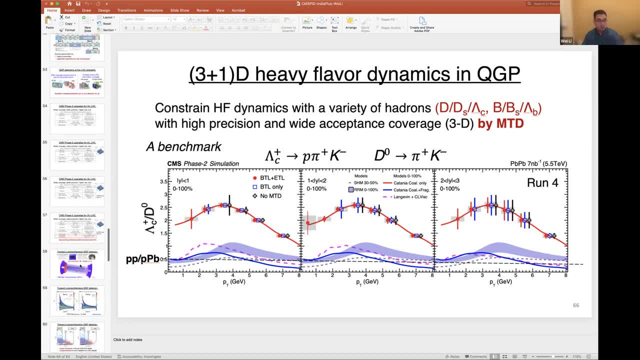 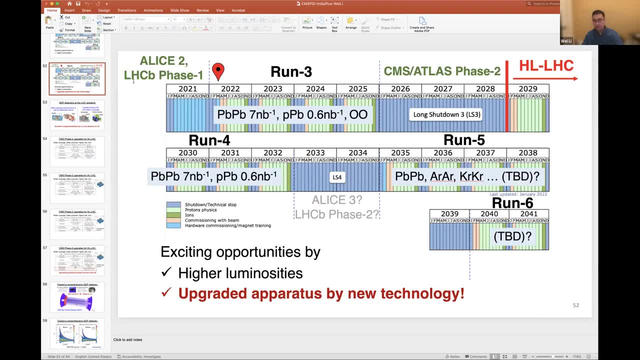 Yeah, for run three. let me go back to here. So for run three there is a. there are some minor upgrades, What we call a phase one upgrade, but it's very small changes Because the runs compared to run two. 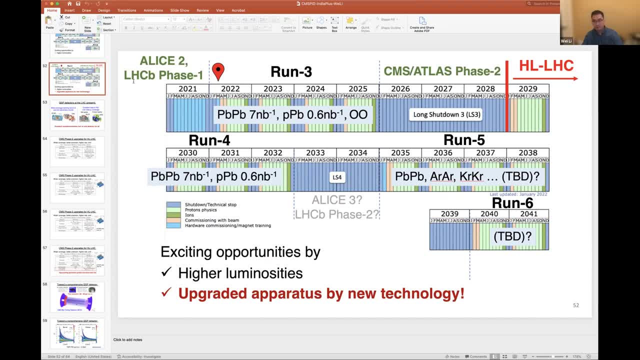 the luminosity increase a little bit, maybe by a factor of 1.5 or two, but not much, not dramatically. Therefore we don't have to have a major upgrade of the hardware. So there's very little change to the CMS detector. 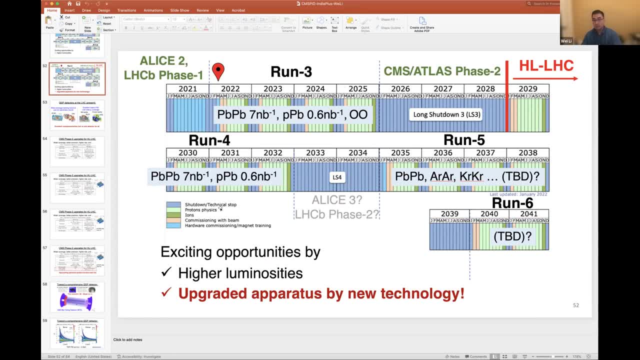 for run three, But for run four the luminosity will increase by another factor of five. Then we need the phase two. upgrade is a major one. The CMS will become almost completely new detector. Okay, thanks. Subash had a question which is: 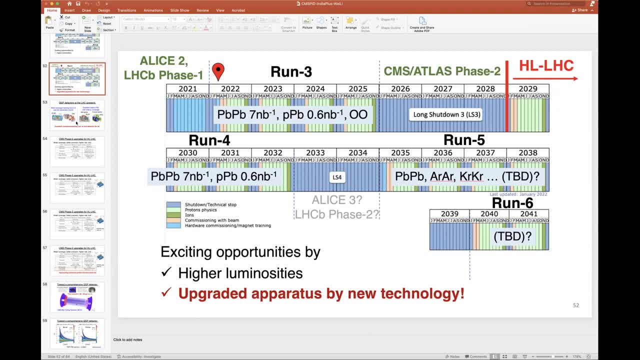 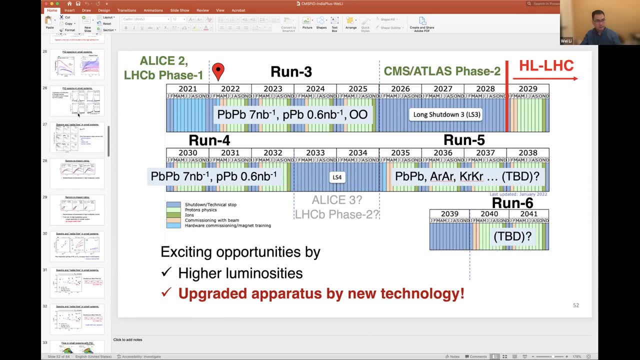 what is the typical DCA resolution achieved and how does it compare with other LHC experiments? Okay, So, thank you That. I don't remember exactly the resolution of DCA, but maybe you can look at the pixel. It's the DCA it's gonna be determined. 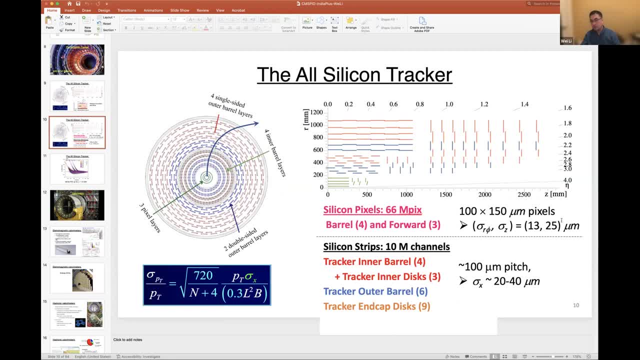 by the resolution of the second pixel detector, Whereas you see here the each pixel is about 100 by 150 micron. And this is the at least the latest inner tracking of the LHC. Okay, So the new tracking detector using the MAPS technology. 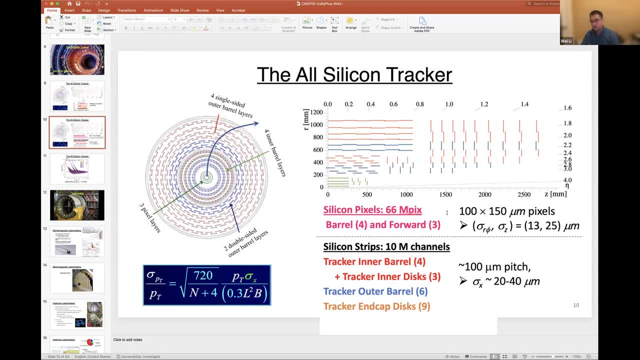 this monolithic silicon sensor has better, has better resolution- I believe it's 50, at least 50- by 50 micron, maybe even smaller and with a less material value. So the DCA, I think that's probably for the new upgrade. 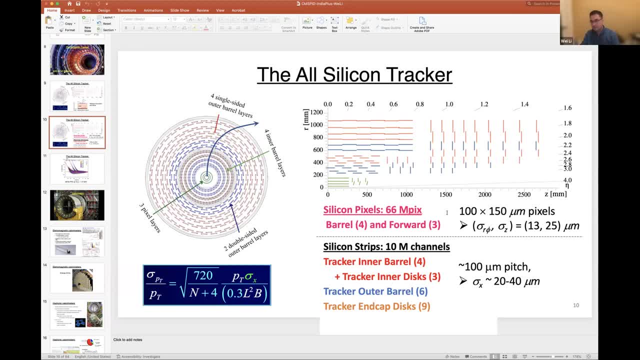 that will happen soon. The previous one- I don't remember what's exactly the what's the resolution And- but yes, at least we'll- soon we'll have a much better DCA resolution, but this is already pretty good. 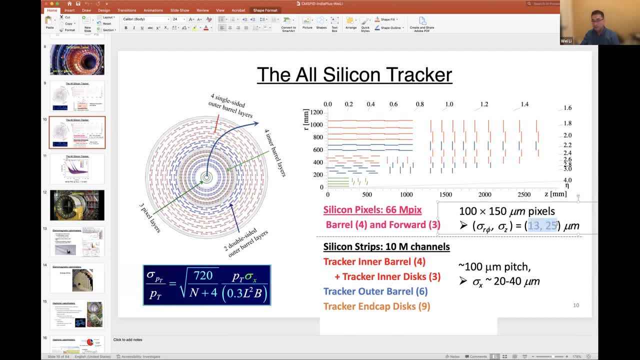 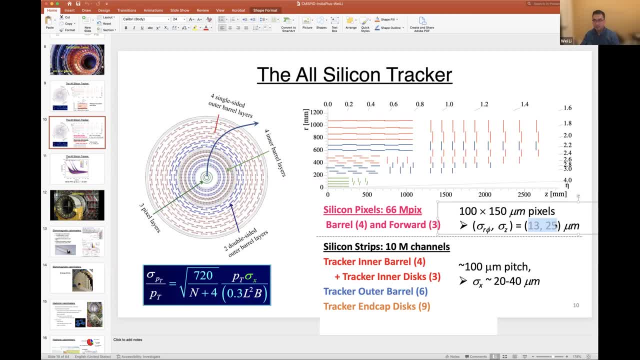 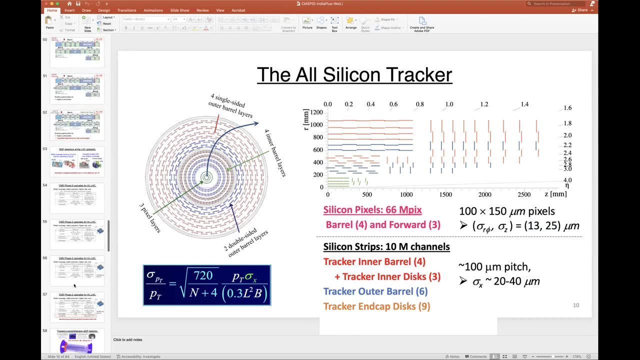 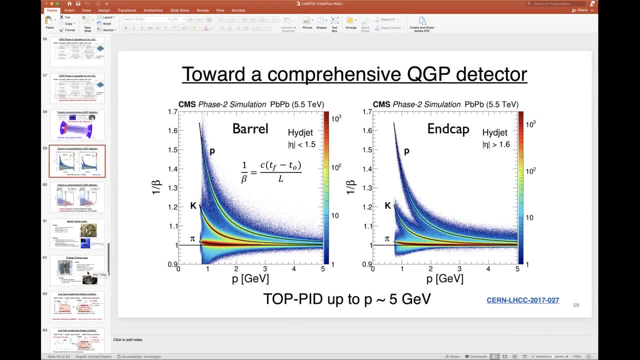 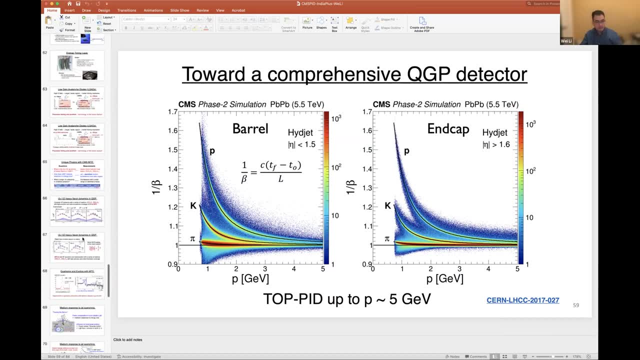 and hyper helium three and between H3 and hyper H3? Okay, So let's see, I'm not an expert in that. So if I remember correctly, the hyper helium three will decay into helium three and the pion. is that right? 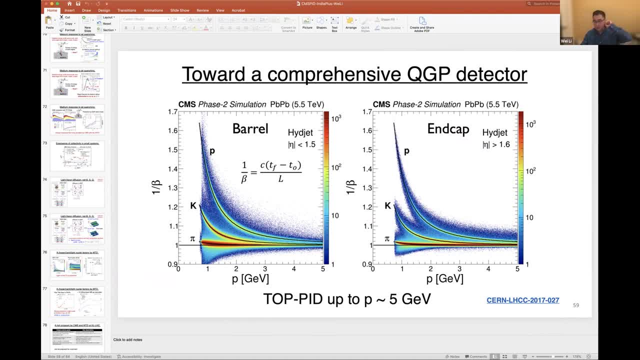 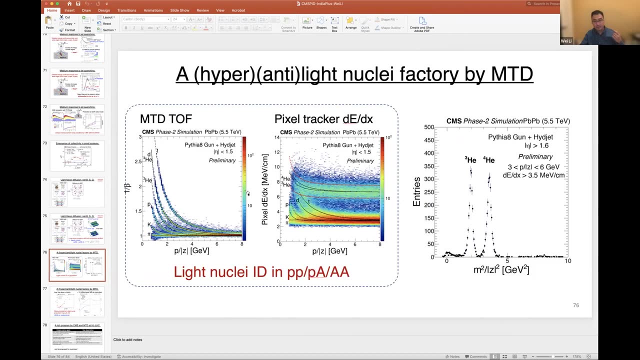 So the hyper nucleus will be detected through the reconstruction, the topological reconstruction And the, so we will be able to identify helium three through it directly. And then we combine that we will do a topological reconstruction with another pion to identify the hyper nucleus. 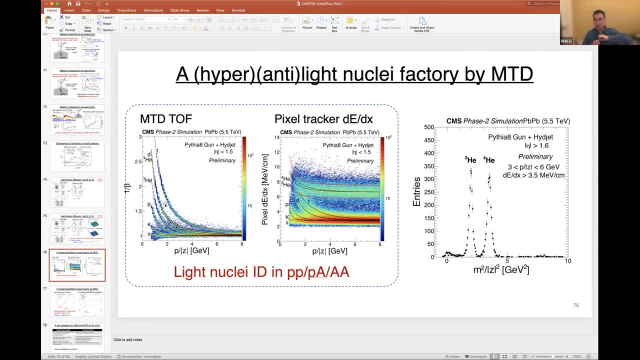 And the lifetime of these nucleus is long right, So that this place vertex will be fairly large. We have not done study yet, but I will expect that we will be able to have very good performance to reconstruct hyper nucleus Including the hyper helium, three hyper triton. 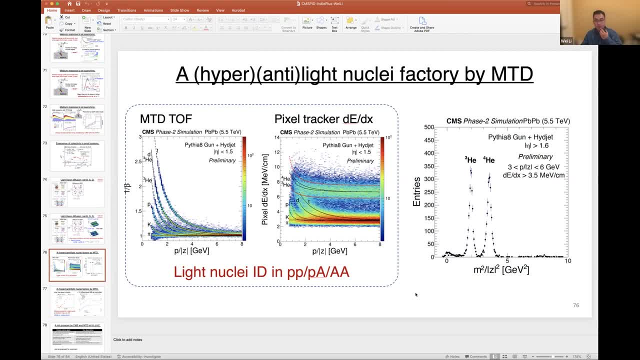 And, yeah, I, we don't have, we will have not done a quantitative study yet. Okay, Thanks. So there are two raised hands, So I'll go. so, Serentum, could you ask your question and then Partha can ask his question. 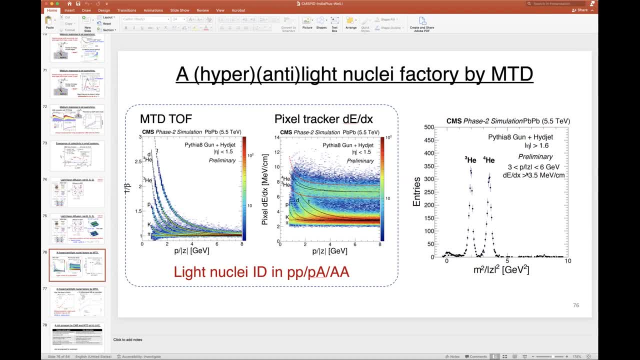 Can you the? Hello Xerin, This was a follow-up to the question on hyper nuclei, and I think it has been partially answered. So what I was interested in, one of the things that I would have liked to know is an estimate of the fraction of hyper nuclei. 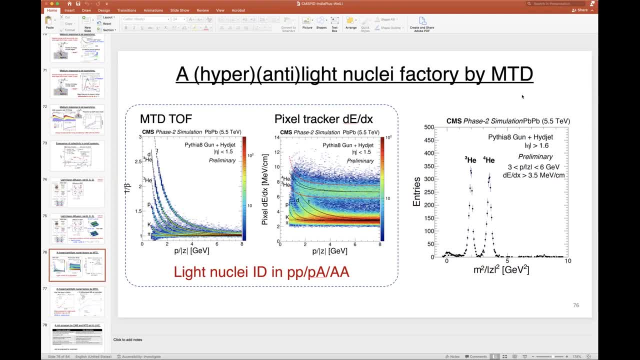 that you would be able to identify, because I'd like to know identify. But since you don't have a complete study, I suppose you can't answer that question right now. Yeah, like the efficiency acceptance, Right? Yeah, we don't have. we don't have a study yet, but in principle we have a coverage of 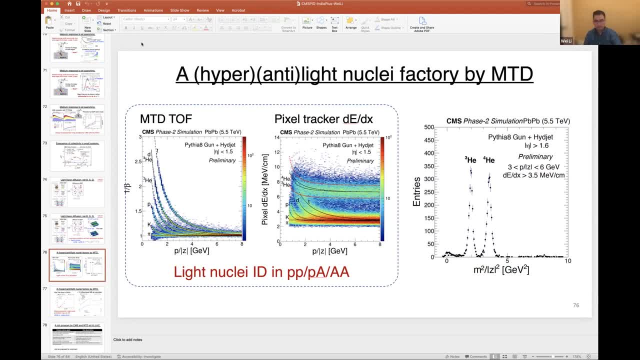 three units in eta. And yeah, as long as the particle four within the acceptance will detect them. Yeah, I think it's a quantitative question to study. There are actually lots of topics one can study with this no-timing detector. We have not done that yet, Thank you. 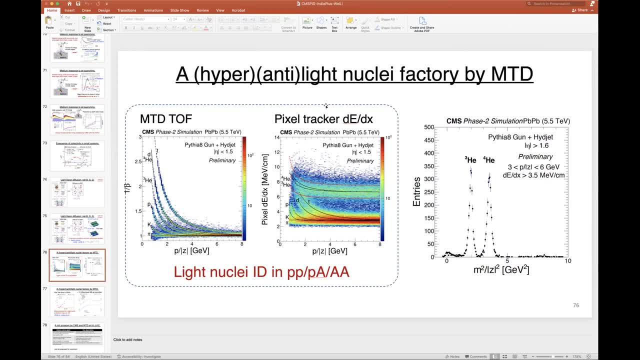 Okay, Barta, go ahead. Okay, Yeah, So my my question is regarding your Charmonia or Jetray measurement. Oh sorry, You use quite a high PTT threshold, Hello, Hello Barta, your sound is breaking a little. 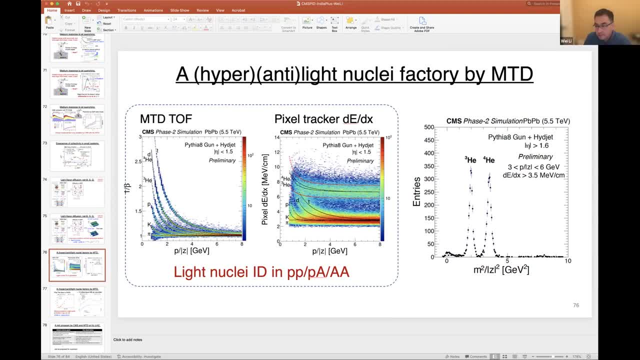 Is that audible? Yeah, your sound is a little breaking. So my question is regarding this high PTT threshold, High value of the low PTT threshold for the Jetray measurement. It is around. at mid-rapidity it's around 6.5 GV by C. 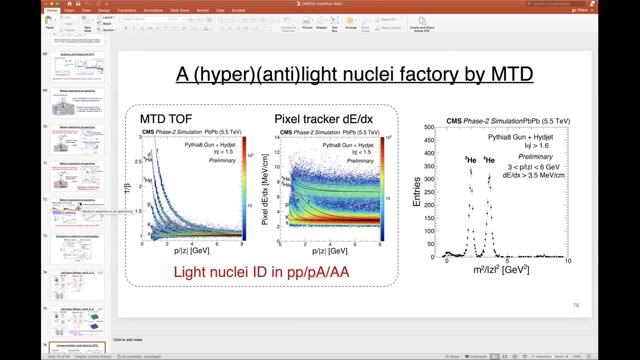 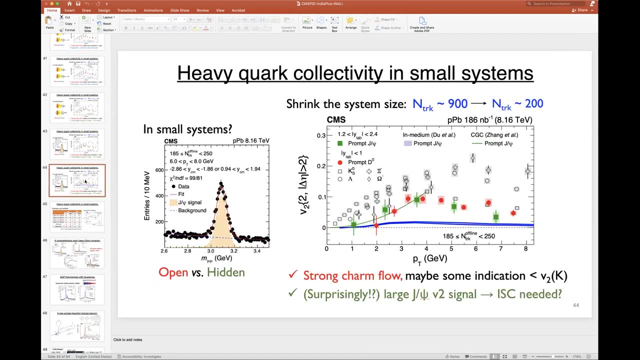 And if you see now a large amount of V2 for Jetray, for lead-laid or P-laid, do you consider it to be of hydrodynamic origin? Barta, Okay, Yeah, I think I captured the question, Yeah. 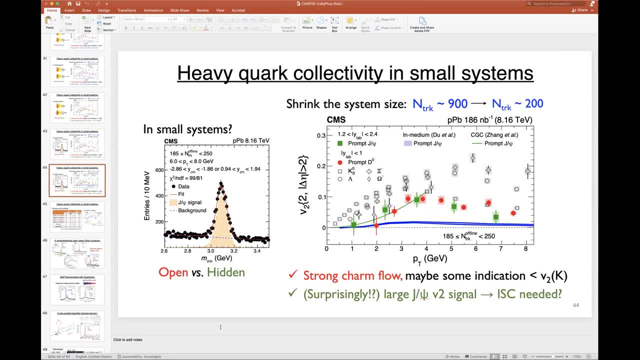 Barta, could you type the question because it was breaking down, breaking up quite a bit. Yeah, I believe I captured the question and let me try to answer Meanwhile. maybe Barta can type the question so that everyone else will get the question. 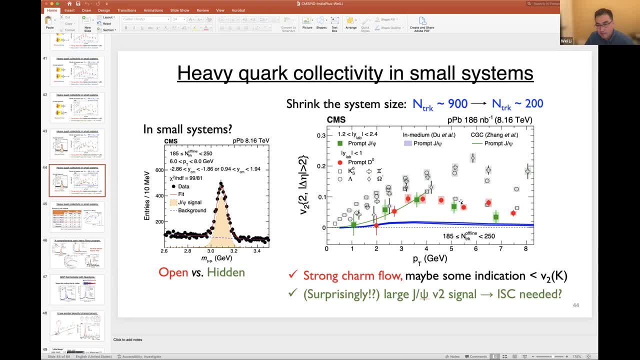 So I think his question is about this plot. Correct me if I'm wrong. You're asking the GFSI V2 in P-laid. Do we see the significant GFSI V2 up to 6 GV or 5-6 GV? 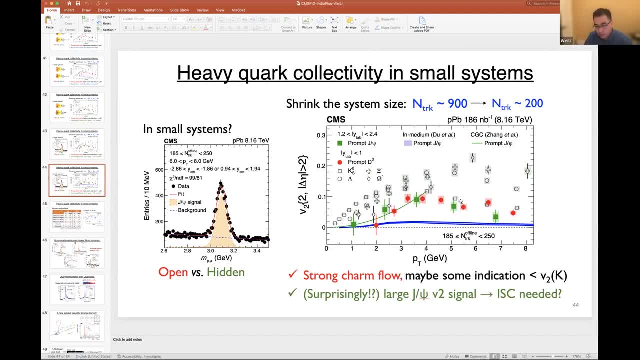 So that is way above the range where we expect the hydrodynamics to apply right. So how do we interpret that? Do we interpret that as the flow, The hydrodynamic flow, of GFSI in small system right And the large value of low PT? 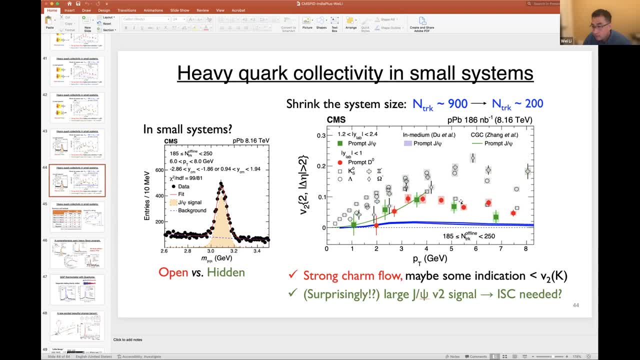 Oh, so you are asking the low PT for GFSI. Okay Yeah, Low PT. Okay, So then I got it. Yeah, Yeah, So it's a good question. And let's look at this plot. So I have a calculation here in this blue line. 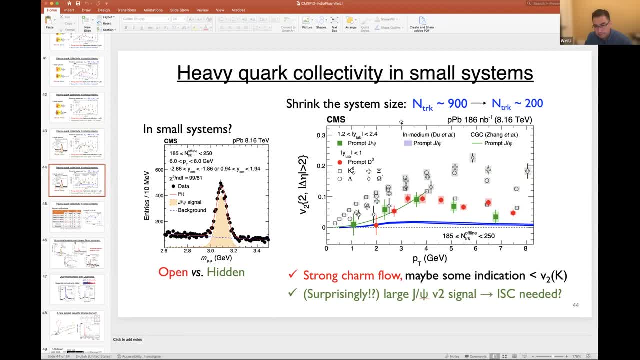 And this is from Ralph Ralph's model, where you have a medium and you have charm quarks, And then you have a medium and you have charm quarks, And this is the flow, And then it is This is the flow, And then they will recombine into GFSI. 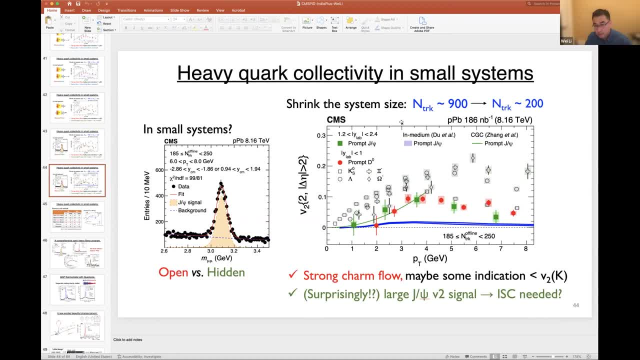 This is how, in this model, they generate GFSI V2.. In P-laid collisions: Yeah, So in that sense, this is a prediction on how much hydrodynamic V2 of GFSI you can generate based on this. Yeah. 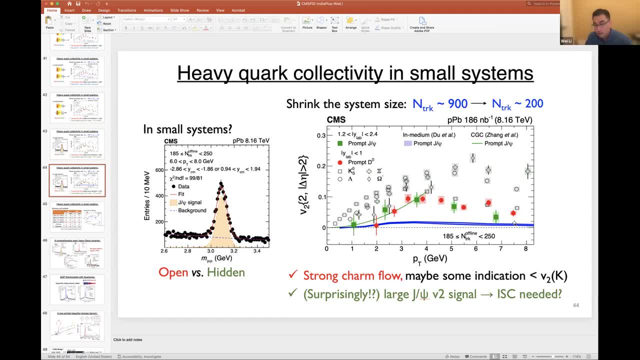 based on our understanding of how GFSI produce, hedronized, propagates in the medium, And you can see that it is very small compared to what we have observed, And that's the reason I said it's a bit surprising that we see these very large GFSI signals. 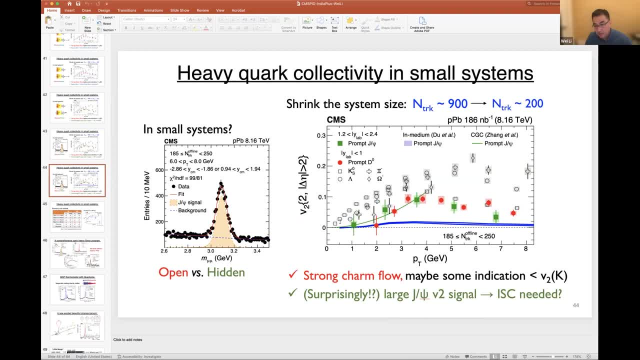 as large as the D0 meson, which is one light clock, one charm clock, And that has not been understood. It is certainly not understood by the medium-motivated hydrodynamic-motivated model And there are speculations that maybe there is an energy loss mechanism. 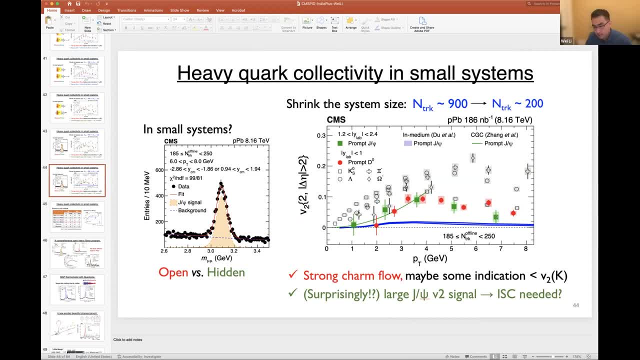 that's not built into this model because this algorithm has a lot of hard probes And there might be energy loss mechanisms that give you additional anisotropy. maybe explain the discrepancy Or maybe look at this curve here, And this is from the CGC calculation. 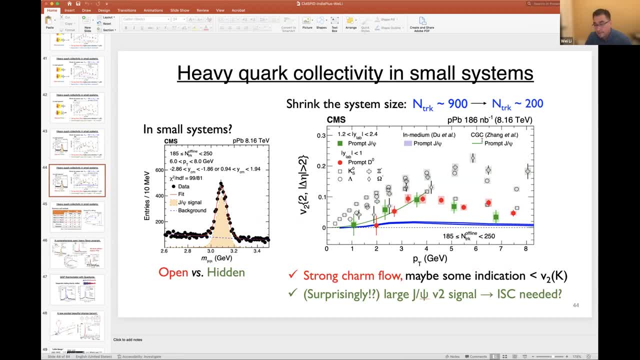 So this is a color glass condensate model that gives you an initial state anisotropy. So with this, without hydrodynamic V2, give you a large initial anisotropy. They claim that they can describe the data. It seems to go through the data. 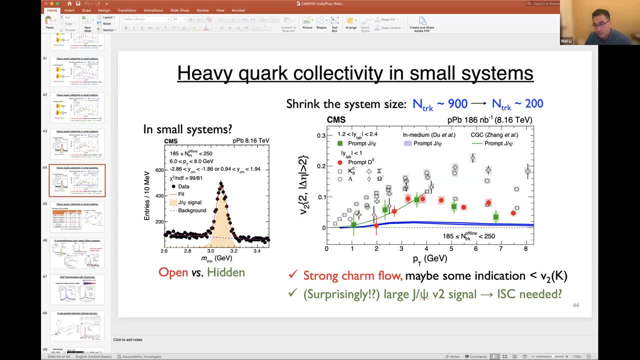 And that will be a very different mechanism from the hydrodynamic flow, the final state effect. So at this stage, the past-length dependence of energy, loss of the charm clock and absorption that can give you additional anisotropy. So that's not in rough. 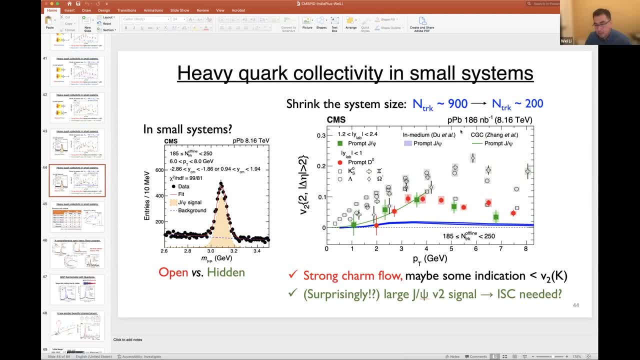 it's not in this calculation. This is only like the hydrodynamic part. So, yeah, maybe that's missing. Or there's this effect from initial state, from the gluon saturation effects, And that is at the moment. we can't tell yet. 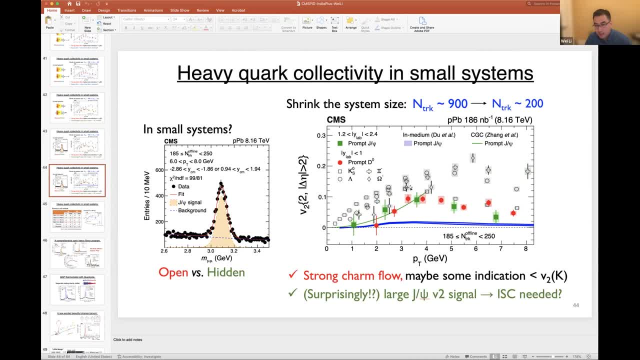 And at the same time, meanwhile, you can see the measurements itself And certainly it's still large right. So that's actually our goal is to try to improve this in RANS3, to really decrease, improve the precision and make it much more precise as D0.. 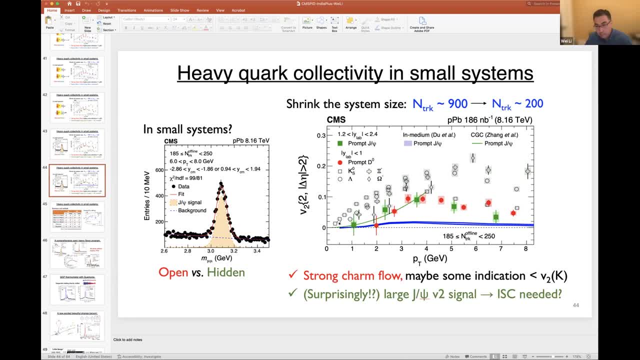 And then we'll see. actually, there's a very interesting prediction from the CGC model that the V2 of the GFCI and the V2 of the Upsilon will be the same. So in the CGC model, And of course that will not be the case. 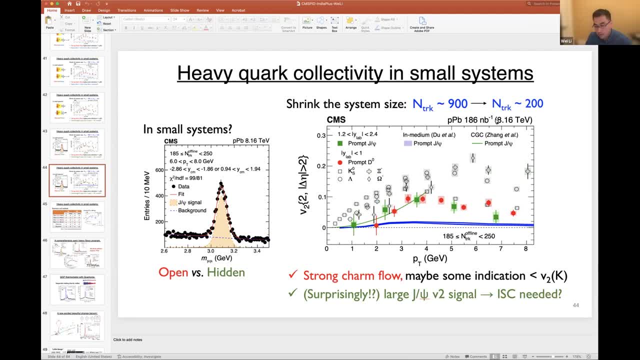 for the hydrodynamic scenario, because it's much harder for the beauty clock to flow. So that's something we can measure. We can test in the new PLED run that's scheduled in 2024.. We can measure the Upsilon V2. 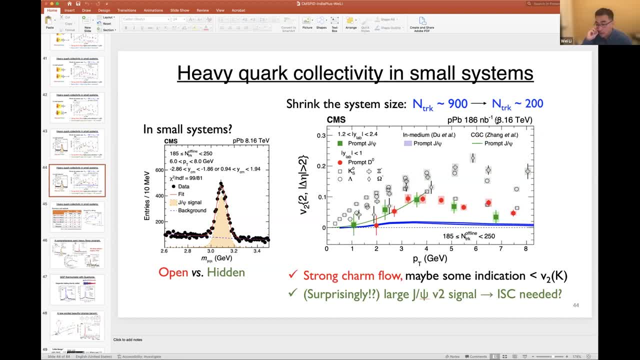 and we can compare it to the GFCI V2 in PLED. We'll see whether they are the same or not, or they show a mass hierarchy And yeah. so I think, and meanwhile I think the medium motivated model should consider maybe the energy loss. 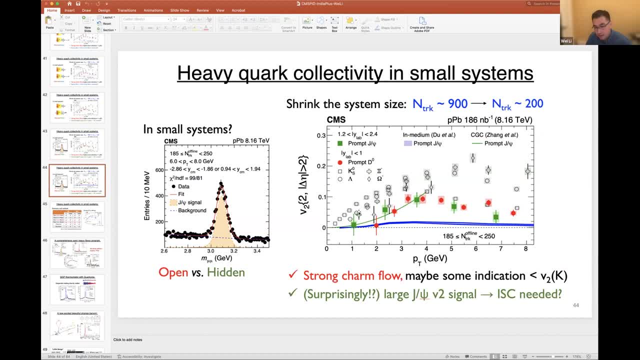 of the GFCI to see whether it can account for additional signals that we may get closer to the data. Yeah, Okay, Thank you, I don't see any, just one second, Okay. Yes, I didn't see any further questions.